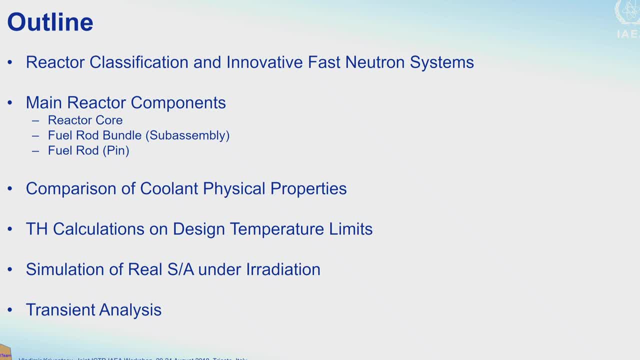 of what is important for the calculations of thermohydraulics, And I will show you the basics, very basic principles: how we simulate thermohydraulics and temperature flow rates and so on in such reactors, which is actually very basic and many of you know very well this. 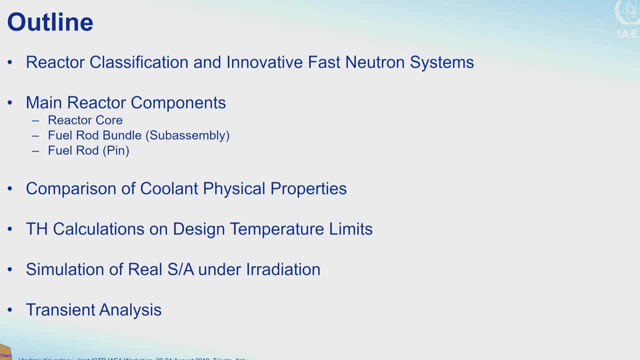 but we will discuss also and to see how we go very quick And the features of the simulation of the fuel assembly- real fuel assemblies which are under radiation are deforming- And few examples of the transient analysis which is most important. 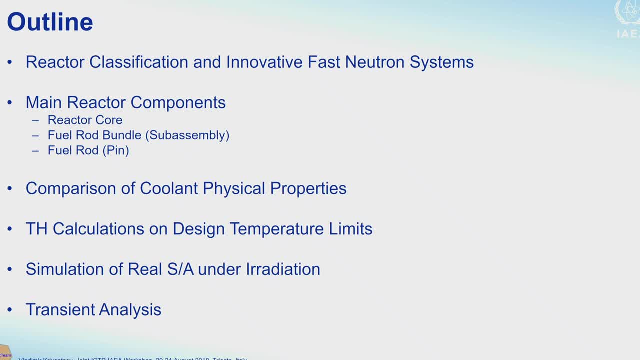 and for the safety. It's one of the most important steps and also very complicated problem to simulate, unlike this basics principle. Please, during this my talk, interrupt me anytime if you want to ask question or comment or you find maybe mistakes or errors in my presentations. 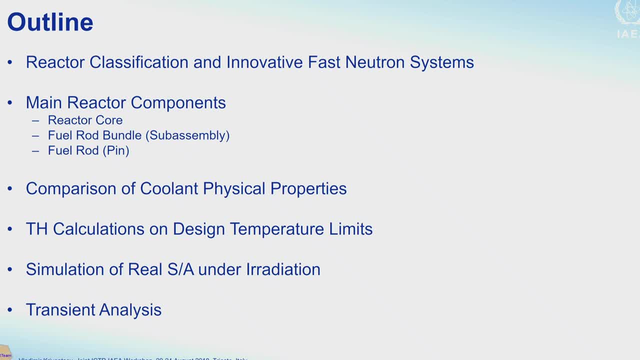 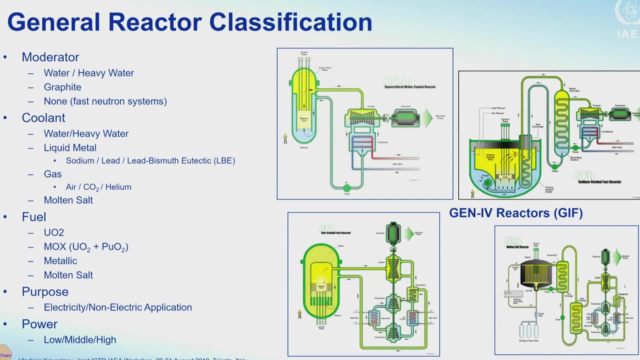 please let me know or for any questions, please interrupt freely. We have enough time, I hope, and we can do Okay. So, as you see, this shows. this slide shows again this famous generation for reactors, presented by GIF. 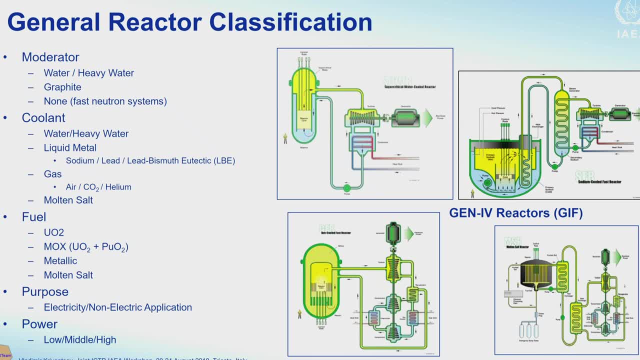 We also in the IEA. we have little bit different terminology. We call it innovative, innovative advanced reactors and most of them are in fast neutron spectrum for the reasons like Massimo explained in the first lectures and you know already, And generally there's different methods, how to classify the reactors and so on. 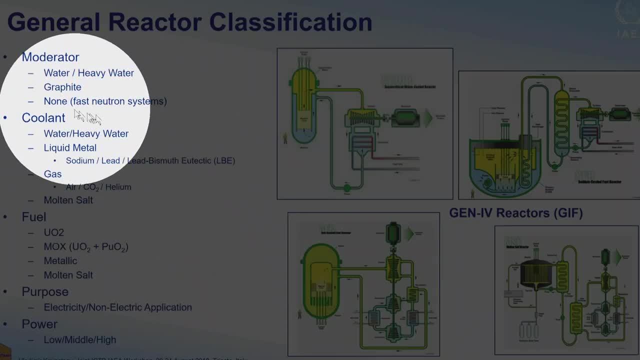 We can use. first of all- and for us it's important- reactor can be classified. one of the features is moderator. Is it water, heavy water, graphite or no? moderator, or could be other possible things? Another classification, I would say so: moderator, then coolant. 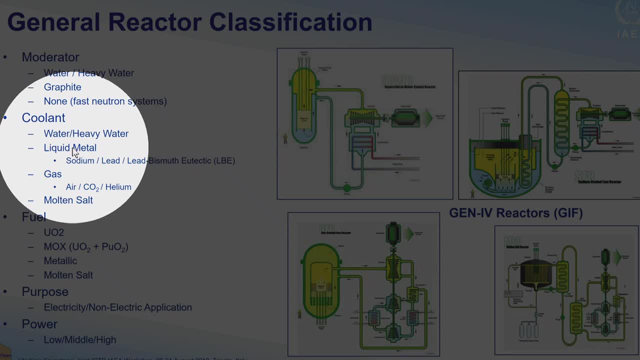 Again, coolant can be water or heavy water or supercritical water as well liquid metal, in this case sodium, lead or lead, bismuth of tactic and air or- sorry, gas coolant reactors. it could be air, carbon dioxide or helium also. 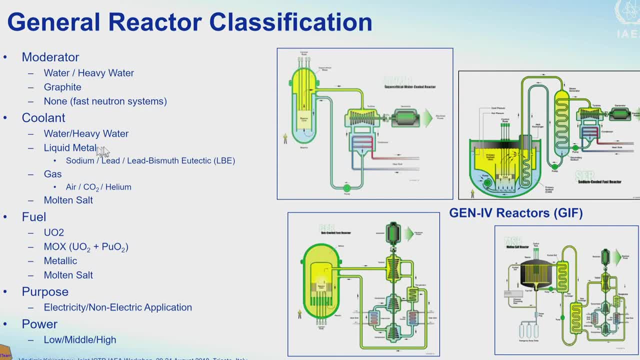 as well as molten salt. This is important things to for classification of the reactor, Of course. next things: it comes fuel and fuel could be uranium oxide, MOX fuel, just mix of uranium and plutonium dioxide. It could be metallic fuel, molten salt. 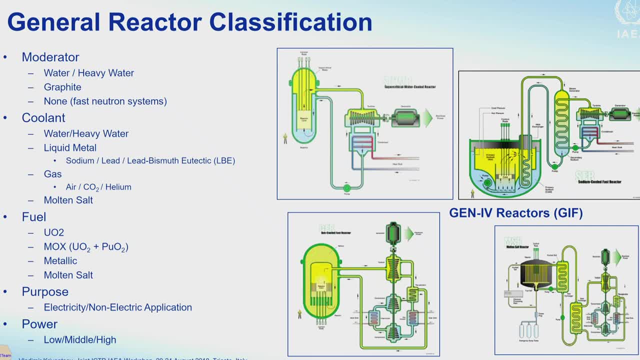 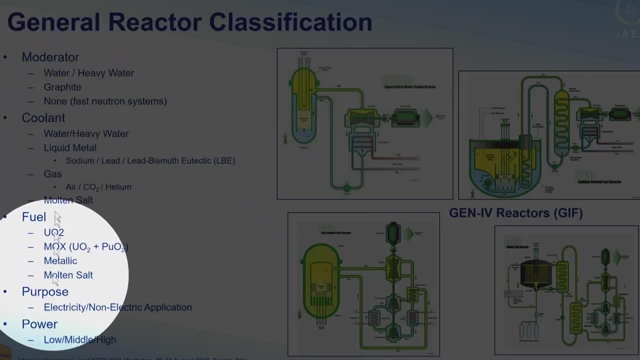 and also another types of fuel, like modern fuel, nitrite fuel and also fuel can be also thorium and some others. Another important classification is the purpose of the reactor. It should be designed for generate electricity or non-electrical applications. 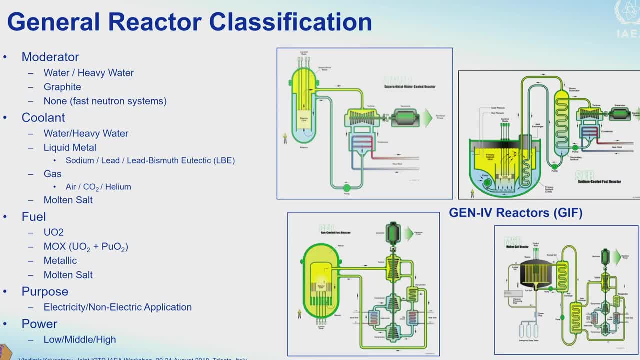 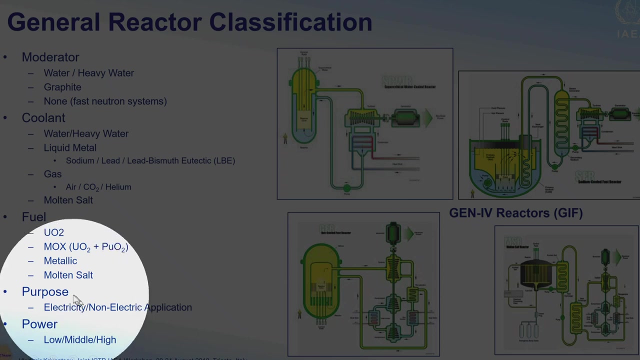 for example, to generate hydrogen or- to excuse me- or to water desalination and several other processes which usually require high temperatures, can be used in the technology And by power we also can classify a reactor, so it's low power, middle, high. 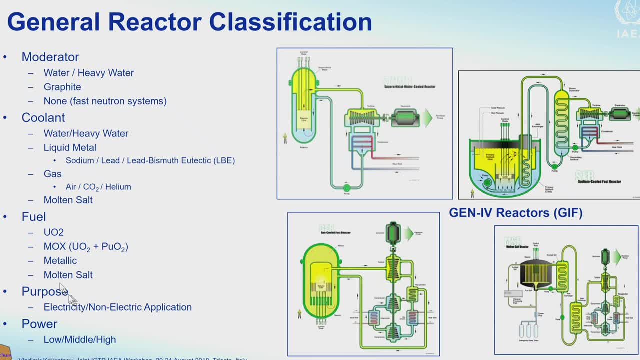 I remember that it was like in Soviet Union from the times when the reactors were started. it was attempt to give, based on this classification, moderator, coolant, fuel purpose and power to give the name of the reactors, like VVR 100,, 1000,, for example. 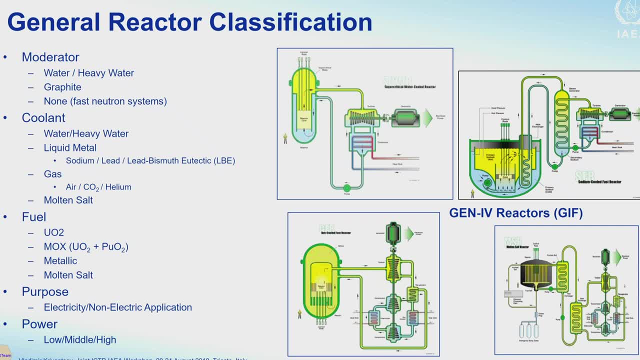 means water moderator, water coolant, E it's energy to produce electricity, energetic reactor and power is 1000.. Then you go to BN 600 or BN 800, so it's fast reactors and B means boost. 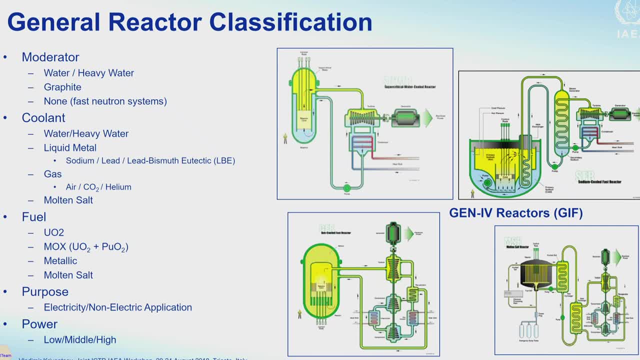 then it's a little bit different. means fast spectrum, then we don't use moderator instead of moderator. it means fast, but also clear. N means natrium in Russian, or natri in Russian means sodium, so it's fast sodium reactor. 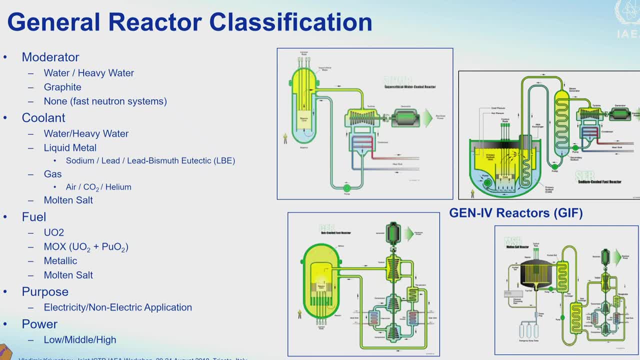 fast sodium, and then you have electric power of this reactor. So this is, of course, this classification is, as any other you know, pretty artificial. so you have many combinations. you can have many combinations of this. In fact, not many, but several. 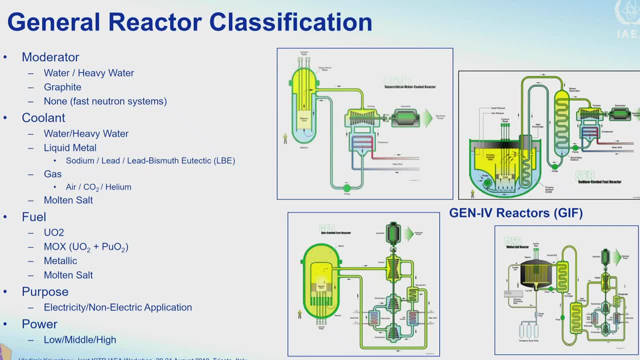 and you can invent new, especially for the new innovative designs. it can be different, but this is just to understand the logic behind this and as you see that all in from six conceptual designs of generation four, we have four of them. 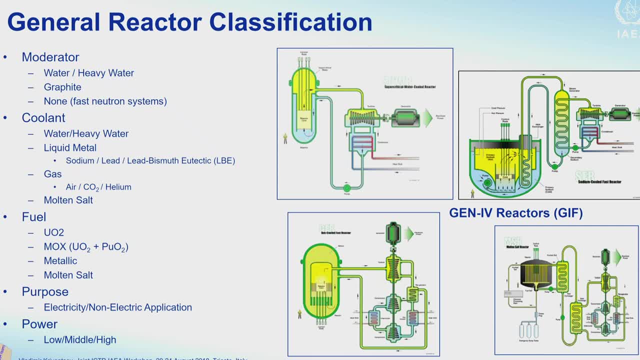 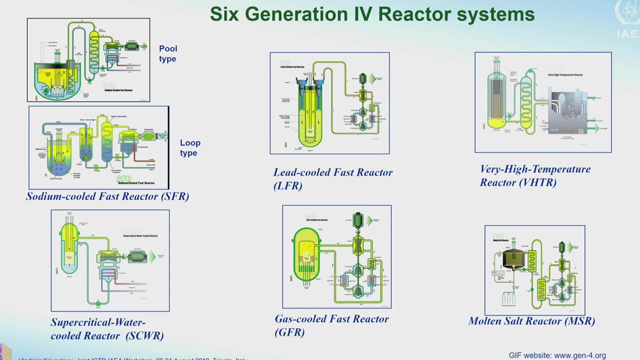 it's fast reactors with fast reactor spectrum, or they can potentially work either in fast or in thermal spectrum, like molten salt reactors. And now I will also again. there are more detailed classifications, for example for the sodium-cooled reactors. 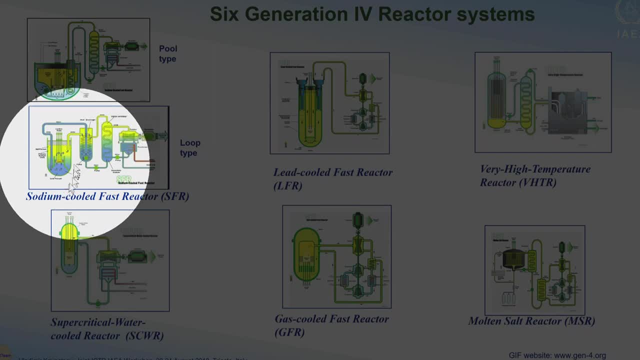 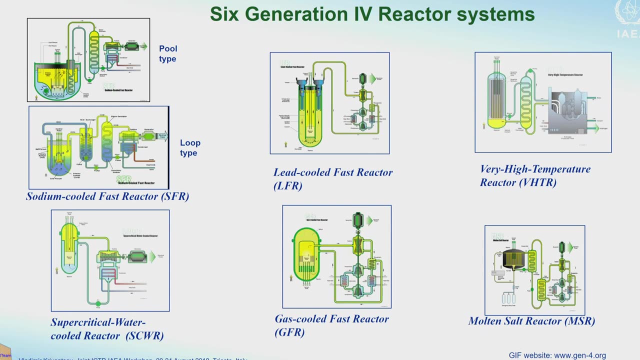 you can have pool-type reactor or loop-type reactor. two types, they're all. both are related to the GIF or GIF generation four international forum reactors concepts. but pool-type is usually using, so loop-type is a special case of the reactor. 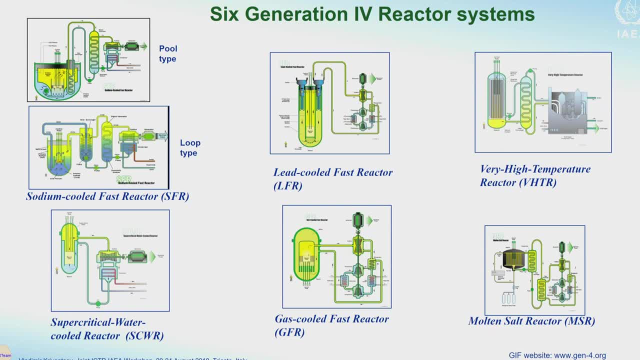 which is used for the countries where probability of escape is very high, like in Japan. So Japan is developing the GSFR, or we're developing GSFR, which is loop-type, but in main cases or small reactors also could be loop-type. 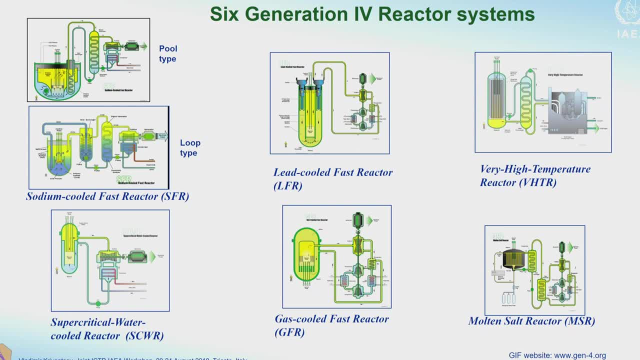 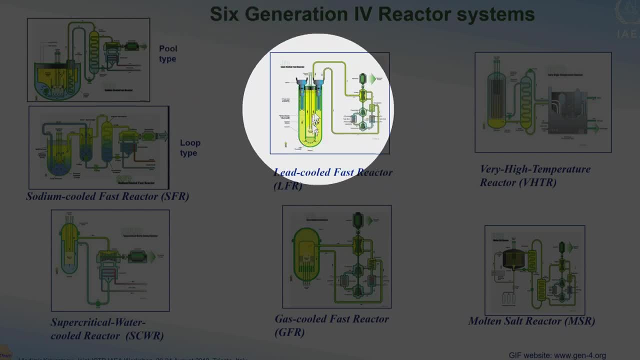 but pool-type is just mainstream for the SFR sodium-cooled fast reactor. Then another possibility is lead-cooled fast reactor. LFR, which is also could be, is a lead or lead with motor tactic, which is, as you know. 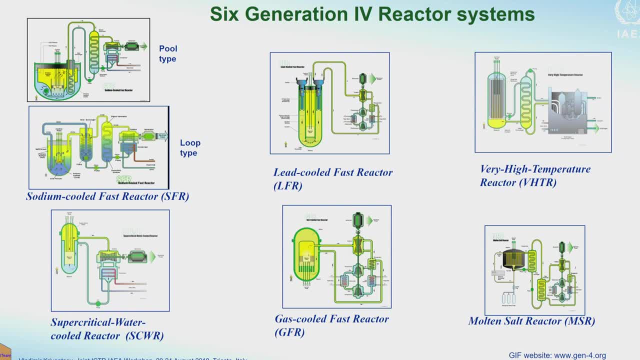 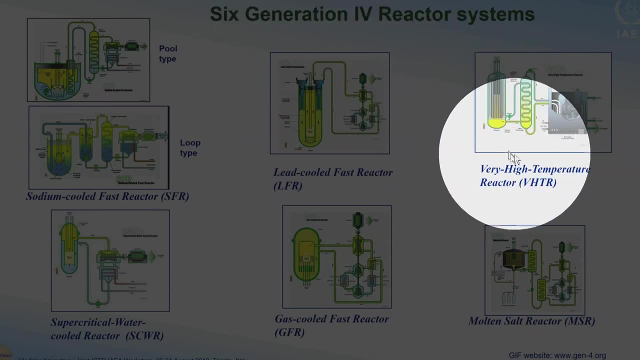 that is the main benefit of this reactor: that we can eliminate intermediate loop, which is present on the sodium-cooled fast reactors because of its sodium violent interaction with water, and this is new improvement. So there is another concept which is not fast reactor. 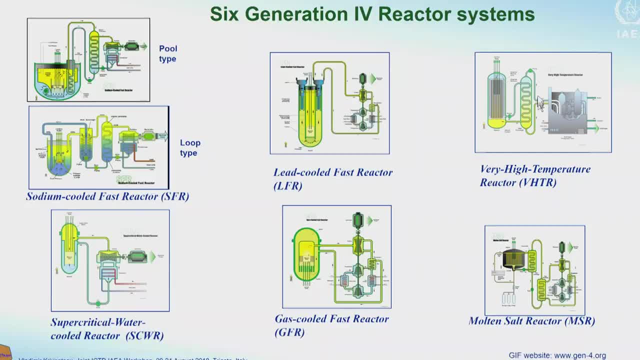 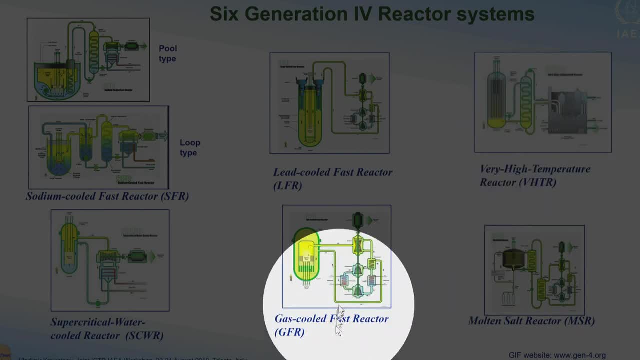 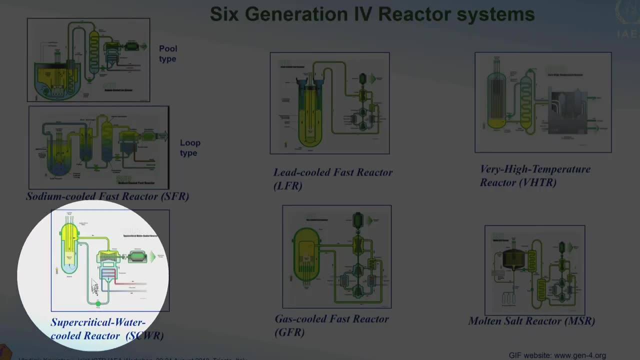 but also innovative very high temperature reactor and- and this is gas-cooled reactor- And then gas-cooled reactor also in fast spectrum, GFR. we have also supercritical water-cooled reactor that can work, actually is in fast or intermediate spectrum. 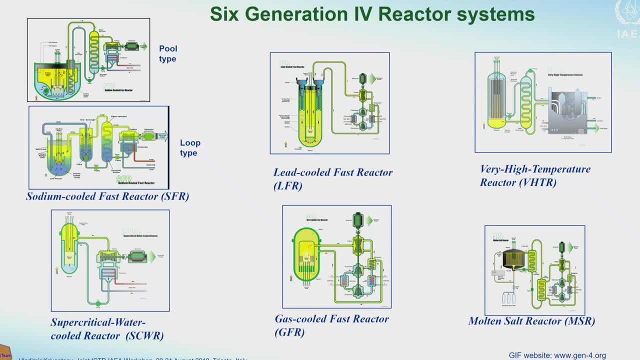 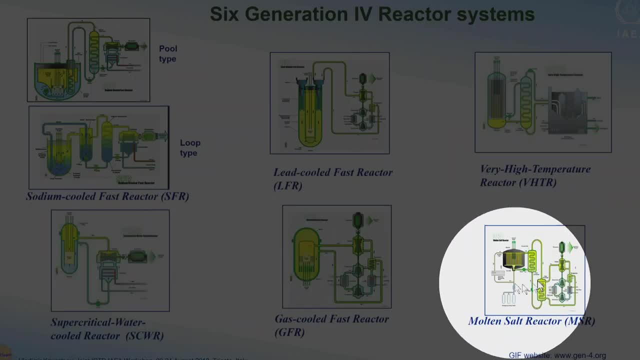 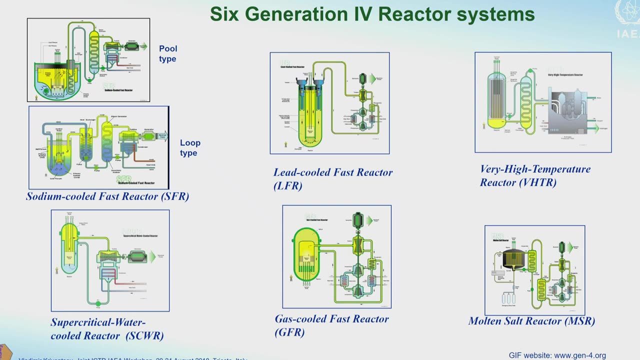 or of course it also can be designed to work in the thermal spectrum as well, but at least potentially it can work in the fast spectrum And molten salt reactors which could also work both in with moderator or in fast spectrum. I think Adrian will explain again in the details. 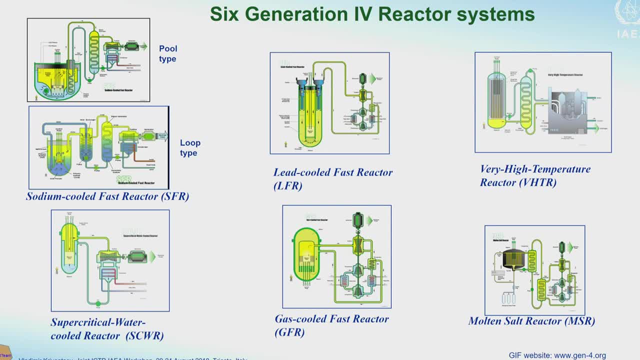 the concept and ideas behind those assistance. What I want to say here that this: most of the new innovative reactors are working in fast spectrum for the obvious reason that it provide give us a chance to develop the sustainable source of energy. Then we need to use fast reactor and 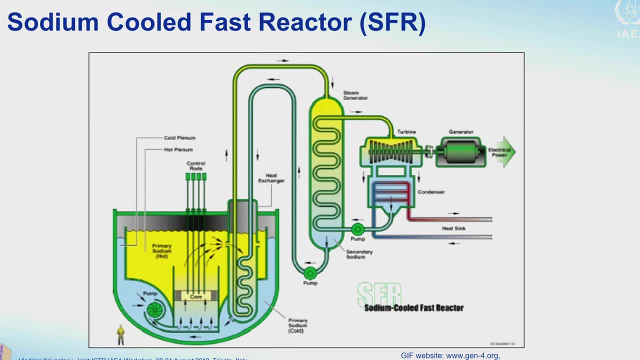 and breathing. Okay, now I think you know this famous picture and I'm wondering why GIF does not print T-shirts with all this type of the reactors like ISTP providing here. Konstantin, you maybe should. it's a good. 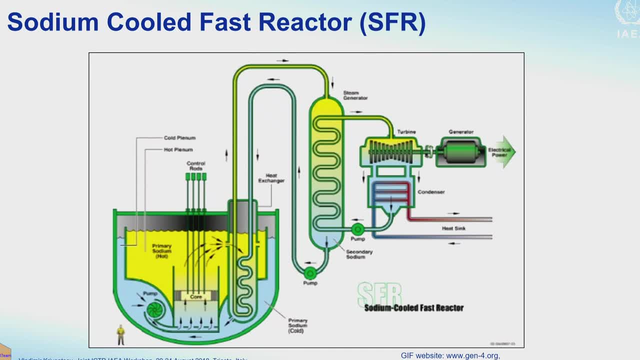 I would buy, especially if it costs five or six euro, like here And on the GIF, Evans would be. it's really nice picture and we get used to this and it reflects well. I don't want to put more attention. 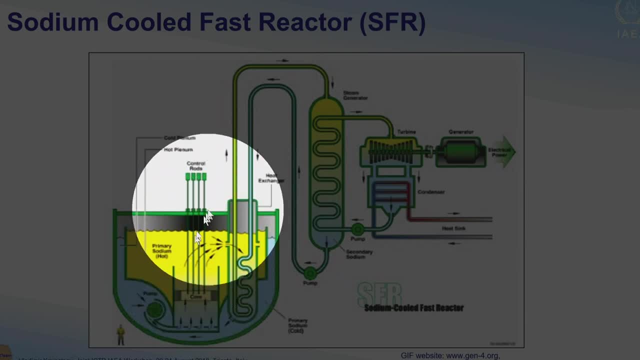 much attention on this. So you have a pool type- it's a big, huge pool actually of sodium- and then you have small, relatively very small core inside and you have electromagnetic or whatever pump, which, which, which gives the pressure to flow. 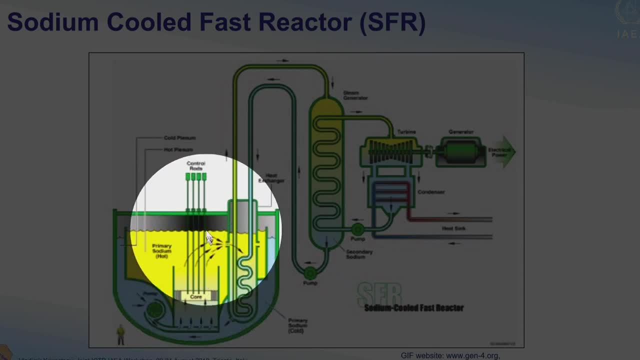 the cold coolant inside the cores. it goes here and then enters intermediate heat exchanger and after this heat exchanger you have again cold sodium entering this lower, obviously cold plenum. and it is how exchange works. 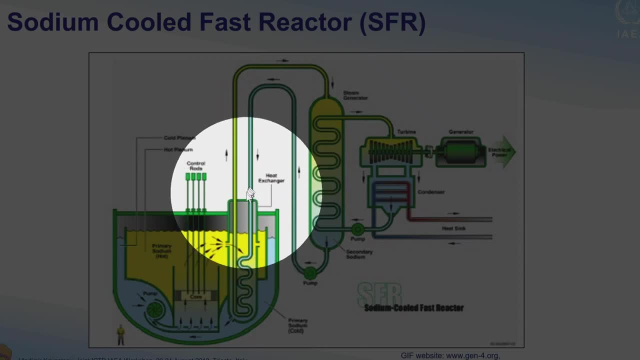 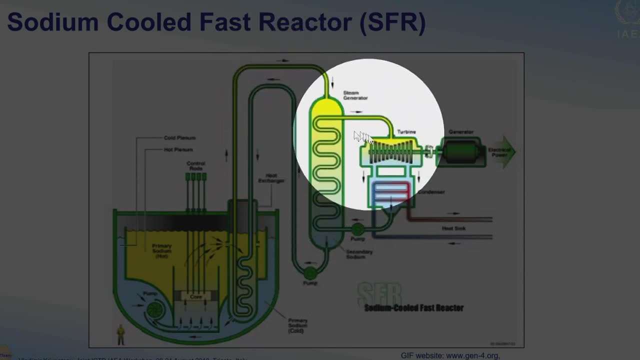 It has a lot of inertia and for some obvious reason, and then from the secondary there could, which is also sodium, it circulate to the steam generator and then goes from the steam generator steam goes to the turbine or could be other different. 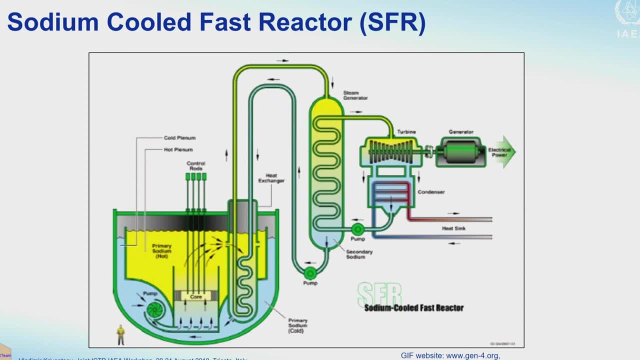 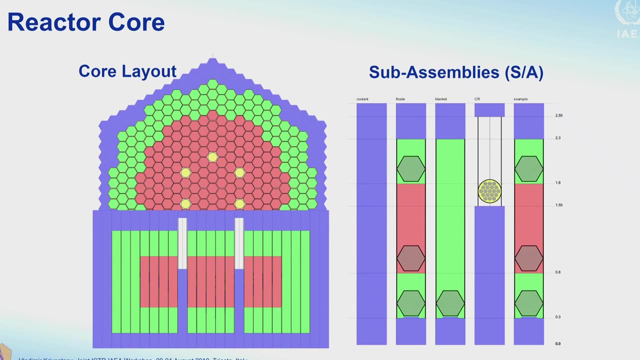 different systems. You know, of course, this concept and I believe, who knows this concept, Who doesn't know? Okay, everybody knows this concept. just I repeat it for the just for the consist, for consistency of this presentation. 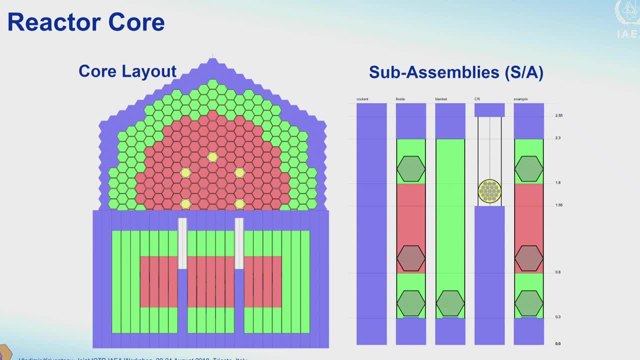 The reactor core is, of course, is one of the main, is the most important or, I know, very important component of the nuclear system and usually for the fast reactors or all innovative. only in Russia also for the pressurized water reactors. 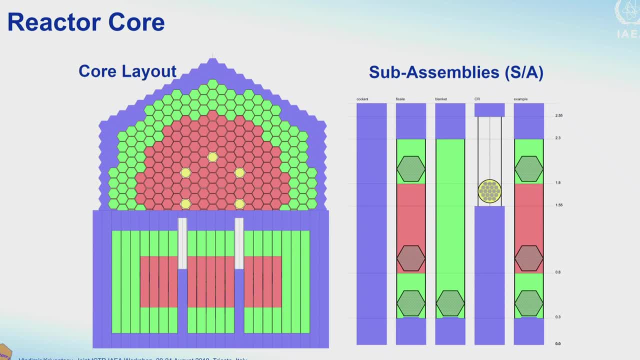 also as well. it consists of hexagonal fuel assemblies and we call here in the fast reactors, we call this sink fuel assembly, unlike in the pressurized water reactor, we call it road bundle. I don't know actually. 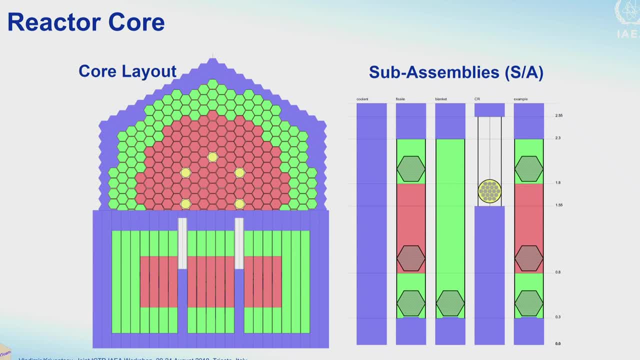 the source of discrepancy because I'm not native English speaker. Maybe if you have native English speakers here, they can explain. what is the difference between road bundle and fuel assembly? Adrian, do you know? Okay, I know only that mostly road bundles. 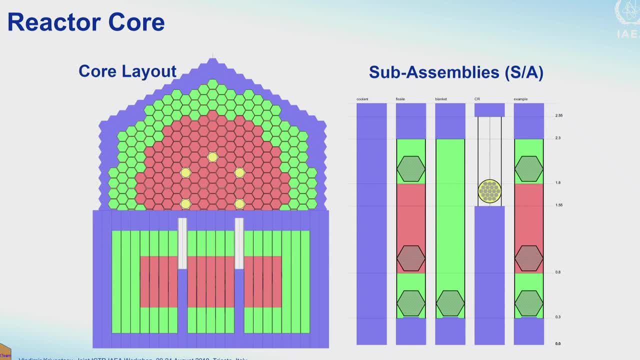 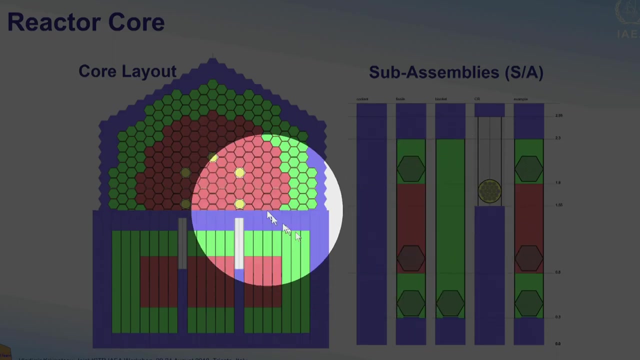 are for the pressurized water reactors and sometimes square square shape and fuel assembly is for the fast reactors with this hexagonal tube. Another difference also, and terminology okay, I will tell this later. so the core is actually the smallest cylindrical shape. 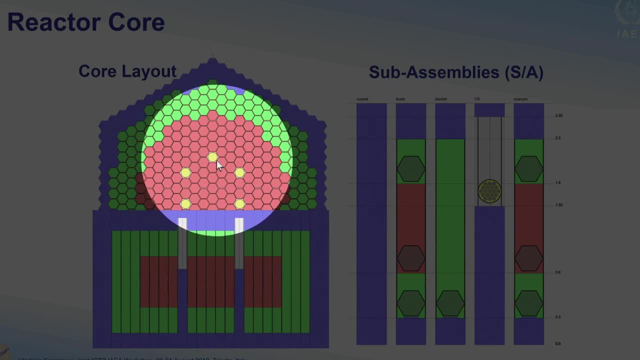 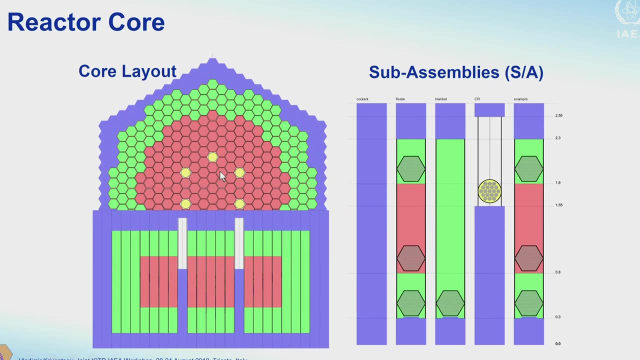 as much as possible, because logically you put it in hexagonal rings, but still you see that they're not perfectly hexagonal- to make cylindrical shape- because it's obviously cylinder is the best shape for this configuration and on this example, 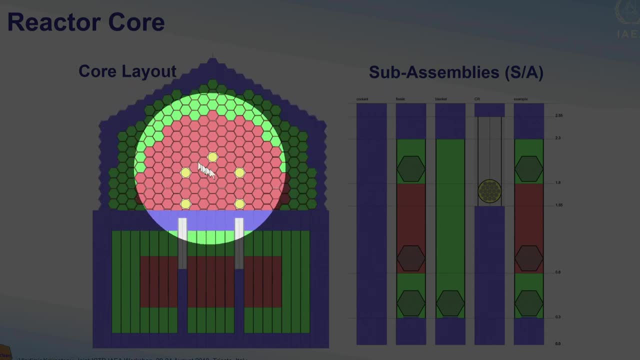 for example, you have different fuel assemblies. the red one is, let's say, inner core, or maybe just simply subassemblies where you have most of energy release, fission, and here the green. it could be, for example, 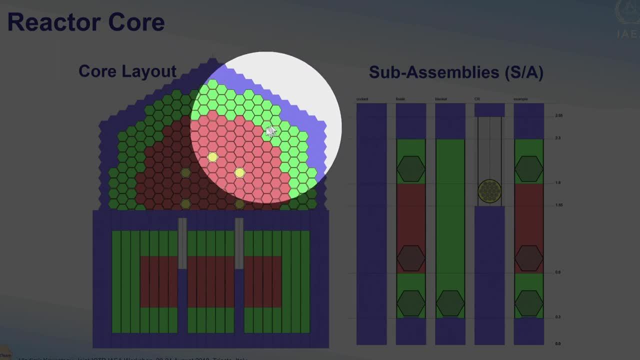 breeder area with fertile- or we also call it fertile subassemblies, which is used for the breeding of uranium-238 to plutonium, to convert it to plutonium, and then you have either shielding or something else. so this is the core layout. 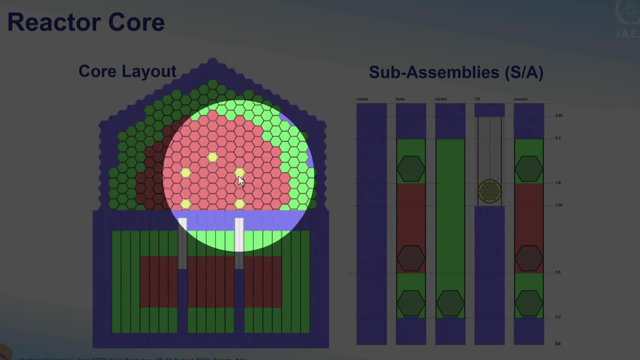 the standard, typical, very simplified, of the reactor, and yellow ones. it's a control road, a shutdown road, which I inserted there. If you look at this configuration from the vertical cross-section, you see that the red is the active core. 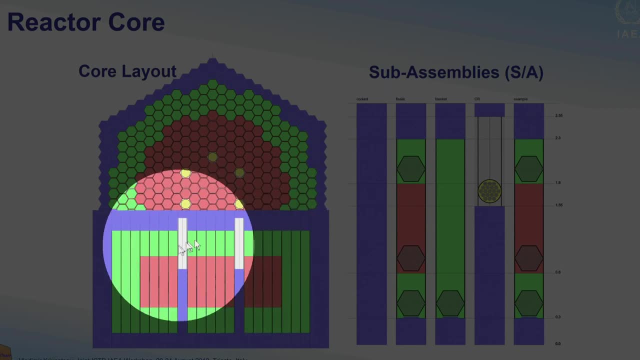 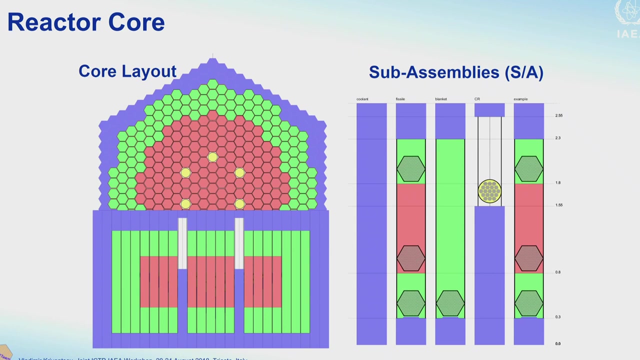 also a fissile core zone, then green could be also a breeding area. when you put plutonium, it's schematic, so it could be different types, of course, and this subassembly, so the reactor core, consists of the subassemblies of different types. 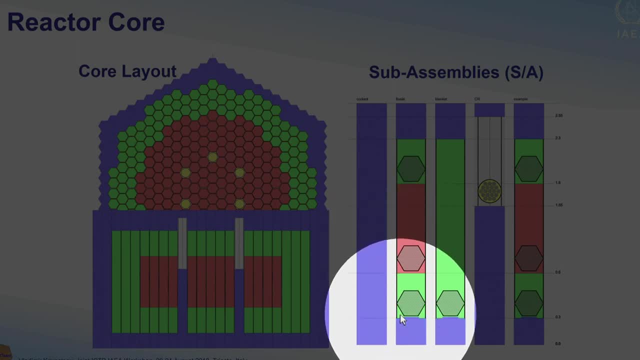 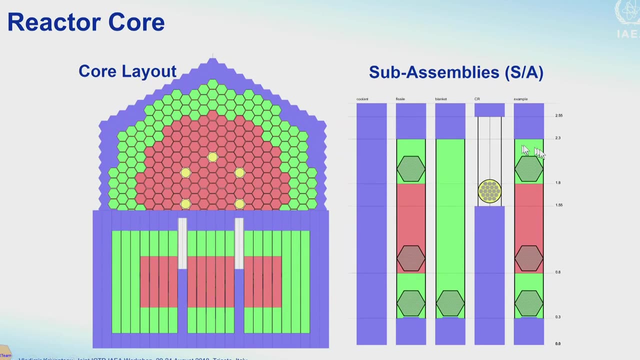 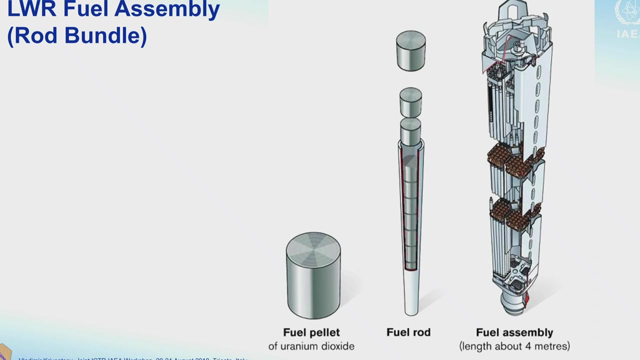 they're different from the inlet to the outlet and this gives you a little bit idea how the core is assembled. So let us compare again fuel assembly, which is in this case a road bundle for the pressurized water reactors. so you have here 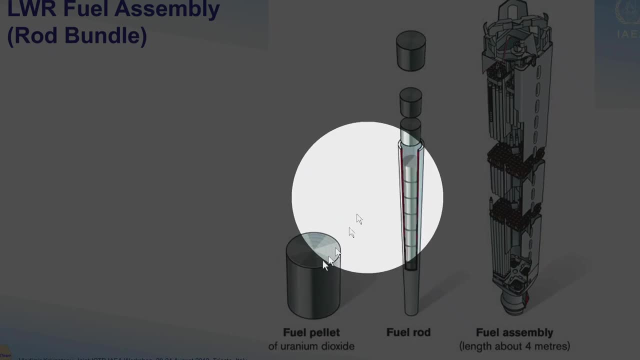 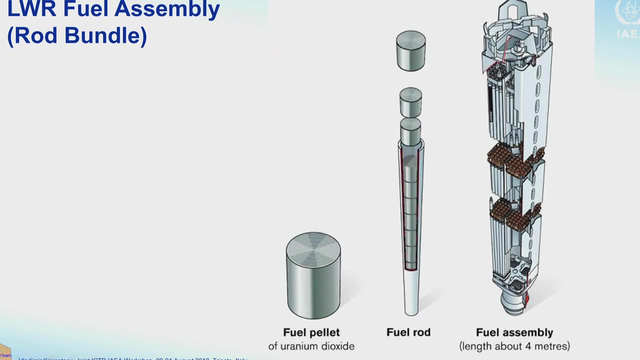 pellets which are inserted in the fuel pin, or fuel rod in this case. and another difference between water reactors and fast reactors is we call this thing fuel pin and in pressurized water reactors they call it fuel rod. Who knows the difference? 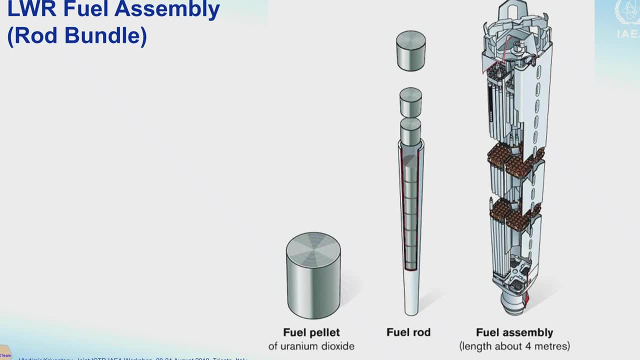 Do we have native English speakers here? What is different between the rod and pin? My understanding is that pin is smaller than rod. Well, yeah, and it is for the fast reactor. actually this fuel element. in Russian we say 12,. 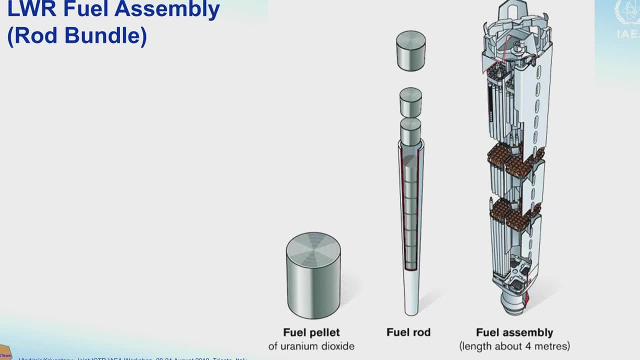 so it's a heat releasing element, fuel element, which is the same for both, but, however, in English you have rod and pin, Which is actually the same, but just be aware of the terminology, which could be missed, And fuel assembly, which is naturally. 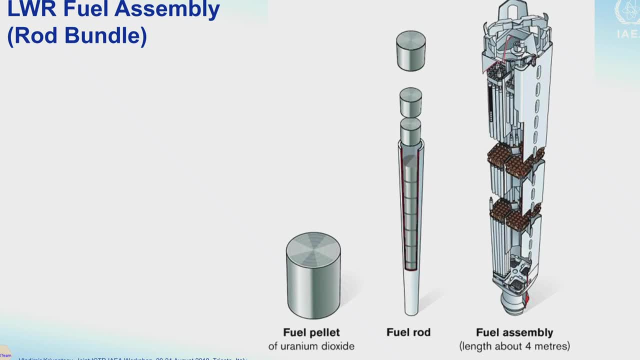 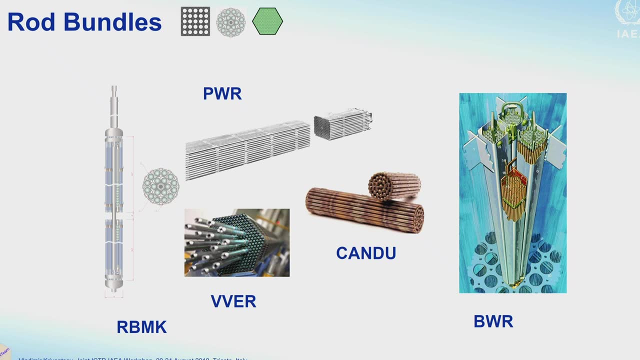 a rod bundle. in this case it's a huge in square shape and this is an example of the rod bundle of the water reactor And they could be very different shapes also for the. you see, there's several nice pictures, for example: 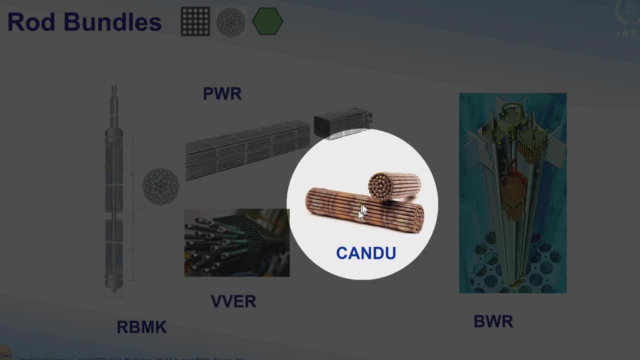 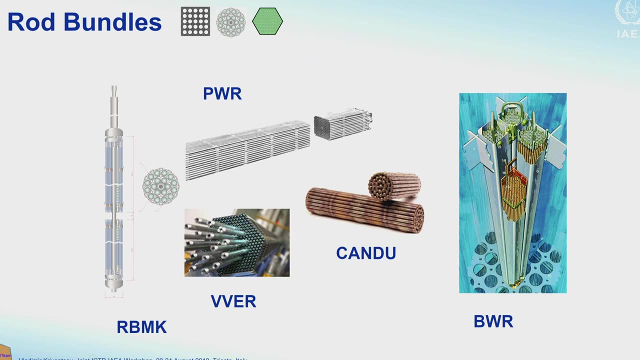 for the boiling water reactor. it's like this for the can do. it's really nice small pieces. I don't know how do they call. I forgot the name. this is not fuel rod, not fuel assembly, not rod bundle. how do you? 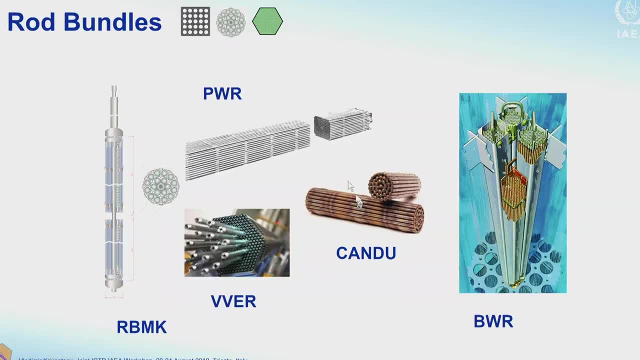 fuel bundle. this piece, I have it in my office. this shape, very nice technology. and they are horizontal. by the way, For the pressurized water reactor I say it's square. and where is hexagonal shape? even it's water reactor? 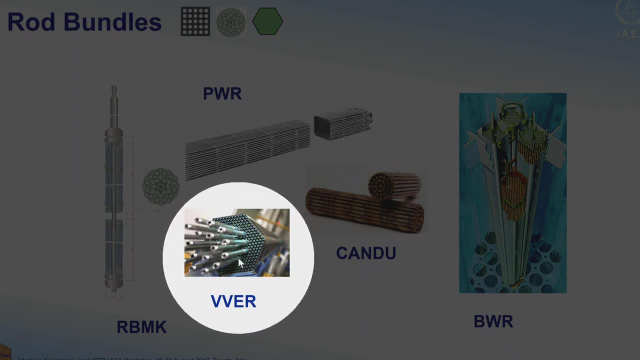 but still it's hexagonal shape historically, and it's, let's say, allows better relation between fuel coolant and structure materials. actually hexagonal shape, It's more effective, I would say, or effective, And RBMK is also. 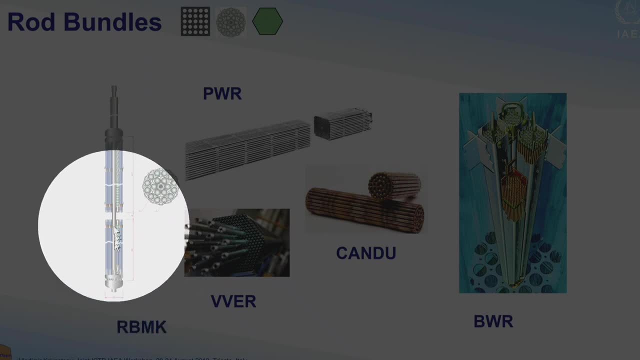 it's a Russian reactor which is doesn't satisfy the classification, but it's, which is graphite moderated and the rod bundle. here it's a channel. let's say, and this, this is not hexagonal, not rectangle. 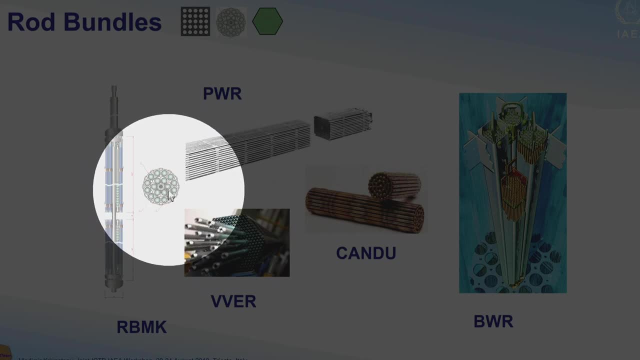 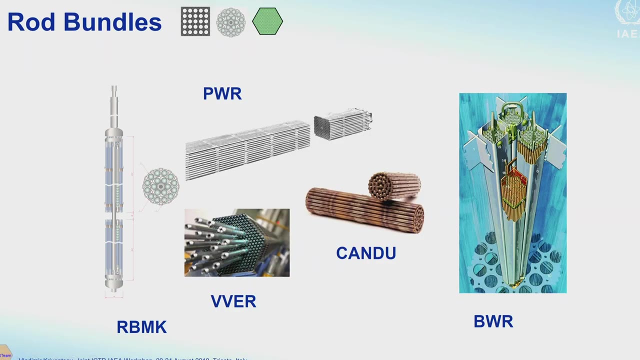 but it's cylindrical distribution. it's not triangle array inside, it's cylindrical distribution trying to fit the cylindrical shape here. So, as I said, the shape of the rod bundles could be square, hexagonal and cylindrical as well, like also in Kandu. 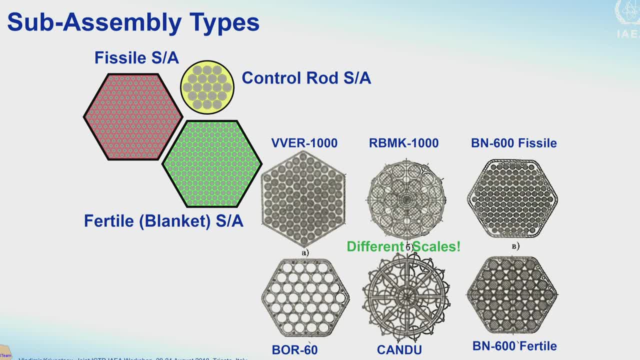 for example. you can observe So, and this slide shows again several examples- and to compare, They are not in the scale, so it's not actually the same size, but but the geometry you can see. So we 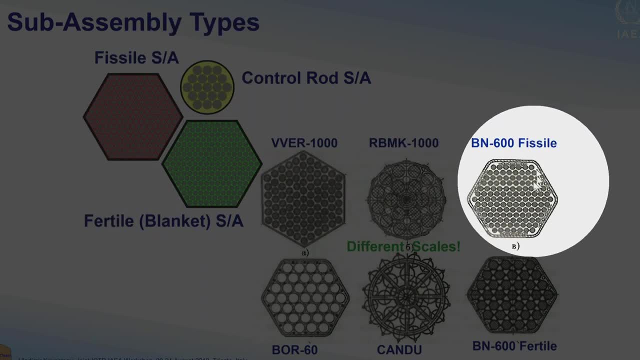 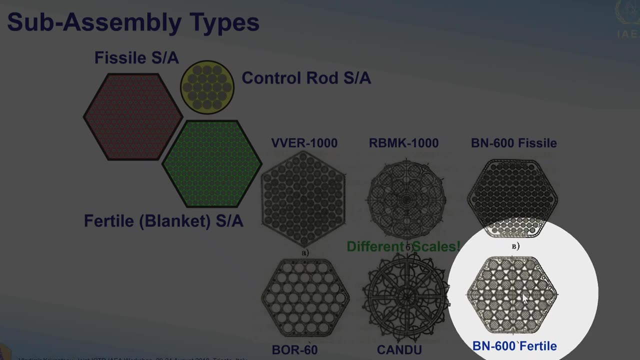 also we can have the in addition to the fuel subassemblies and fissile or fuel of fissile subassemblies. we can have fertile so-called subassembly or with where is a natural or depleted uranium, is converted, is breathed to the plutonium. 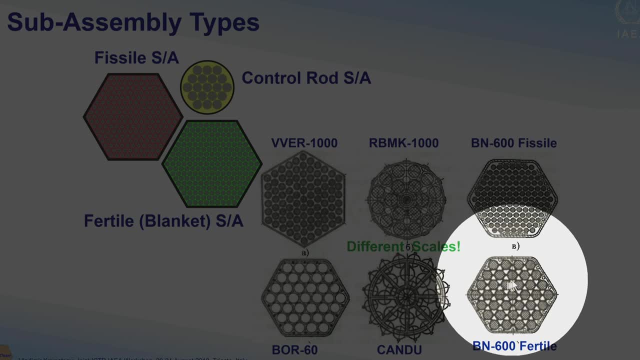 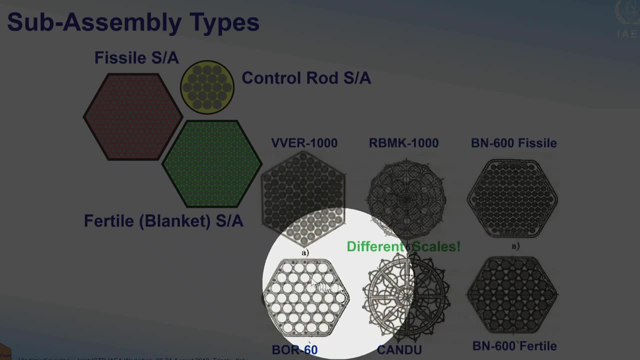 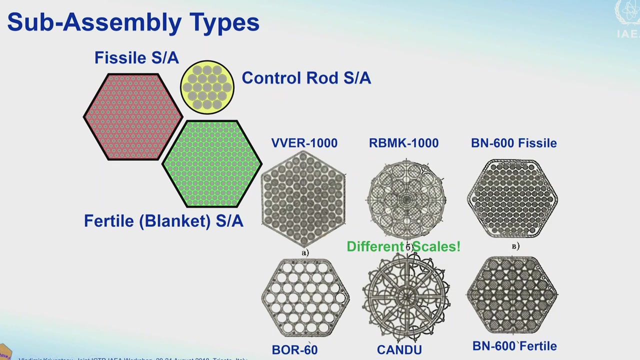 for example, which has bigger size pins or rods and other different side types. It's mainly for the fast reactors. you have hexagonal shape of the tube, of fuel assembly tube which is, and inside you have triangle array of the 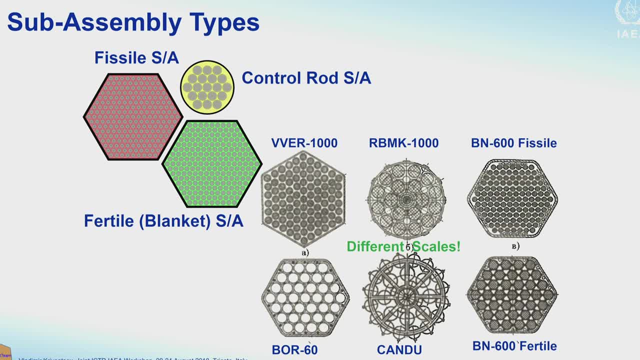 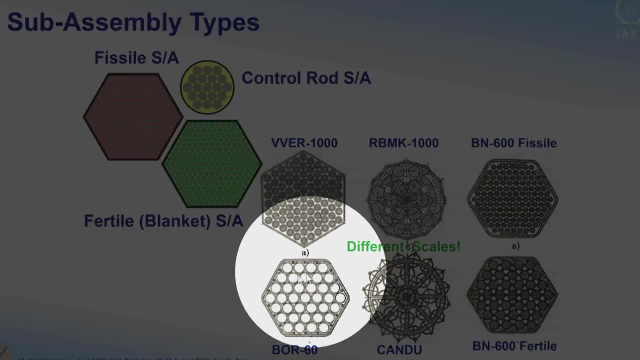 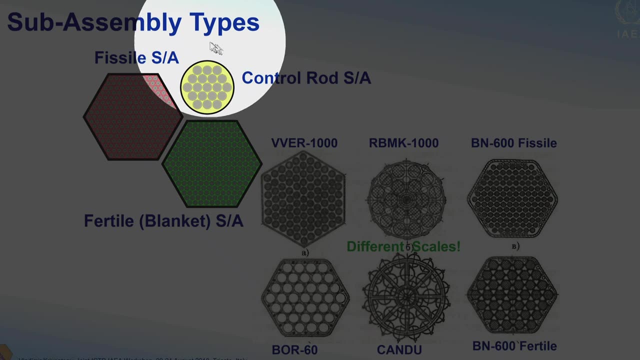 pins or rods, which allows better, more effective relation between the fuel coolant and structural materials in the subassembly. In addition, we also have several special subassemblies, such as contour rods and shutdown rods. that could be even. 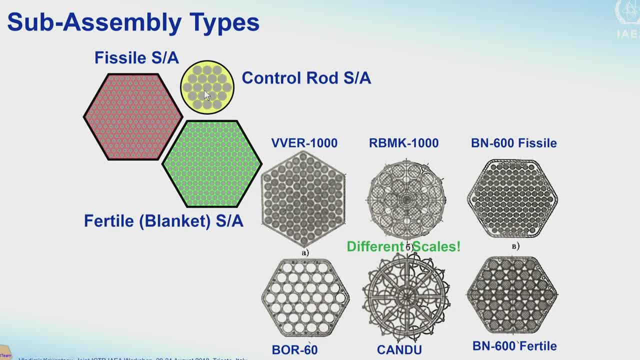 also cylindrical shape and either randomly, or I mean with different type distribution of thicker fuel rods or not, in this absorber rods in this case, for the obvious reason There also the reason of, of course, higher power density we have. 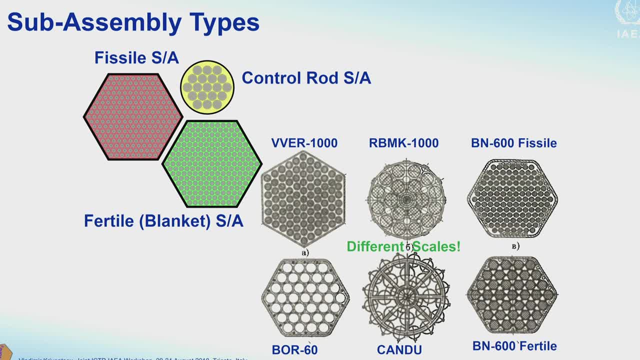 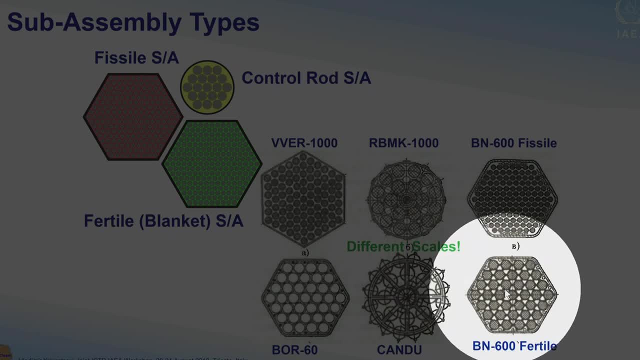 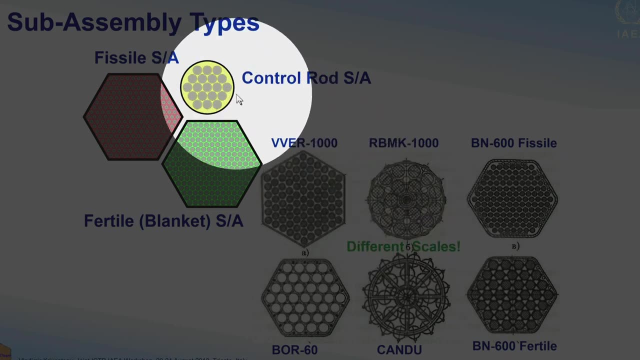 smaller fuel pin we should employ. So if it's release less power, so we can have a bigger, bigger diameter of the fuel pin. or also in case of the absorber material, like boron carbide, so we also 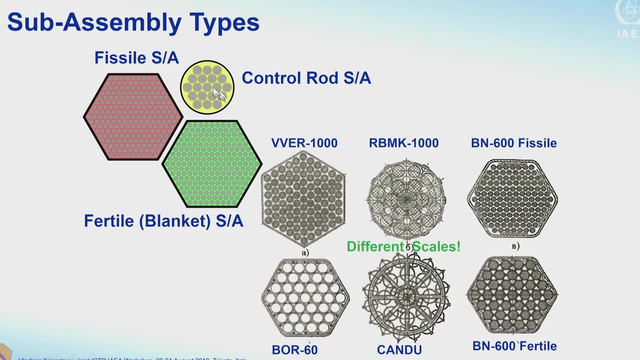 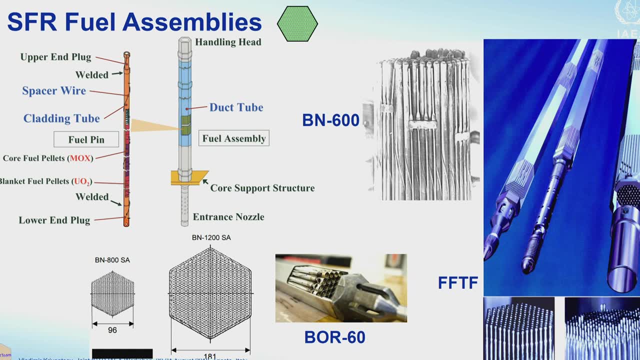 it still release some energy, should be cooled, but it could be bigger diameter. so we can- we can also save on the structural materials here. So, and this is several examples of the real fuel subassemblies with photographs. 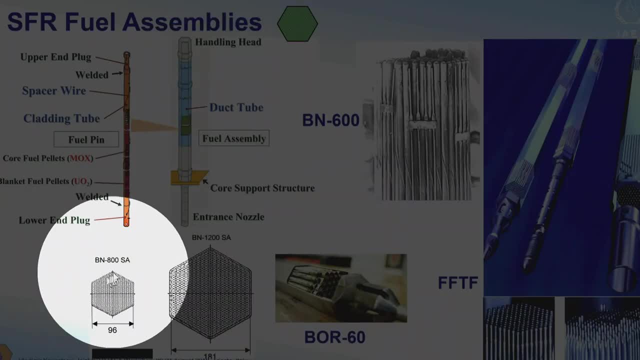 As I said now in scale, for example, for for BN800,. now, BN800 is a reactor, brand new, fast reactor. we call it brand new, but it was developing and designed since 30, you know. 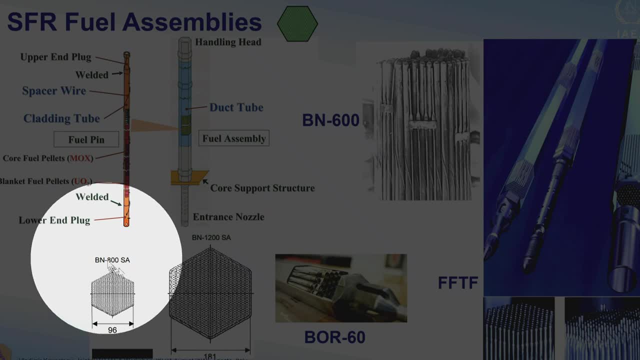 40 years. started design 40 years ago but in two years ago it went finally in operation and operated successfully in the Belarus nuclear power plant in Yekaterinburg. And you see this subassemblies. 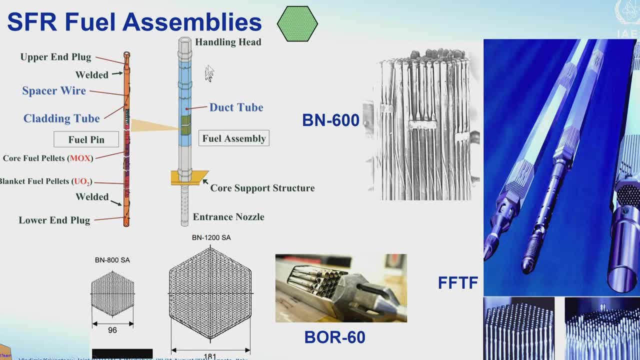 it's already photographed And there are different. so, as you already know that it's, it's combination of this, of the fuel pins, and this is real photograph from BN600, after irradiation you see some fuel pins. 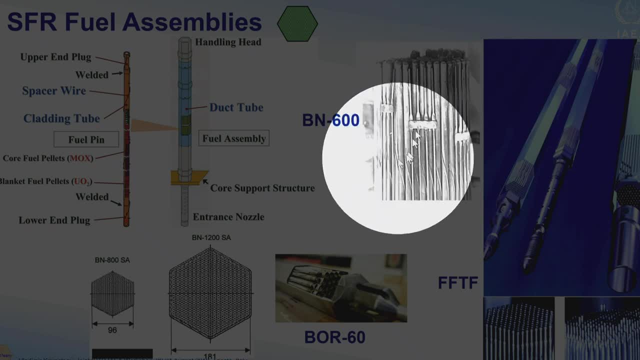 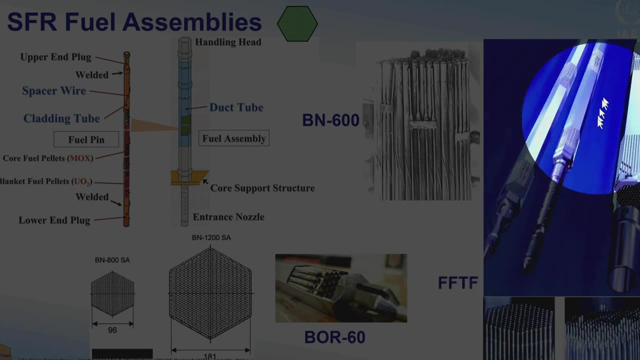 are elongated more than others and they deform it. and also is FFTF, which is fast flux test facility in the in the PNNL in the US. It's it's fuel assembly there. 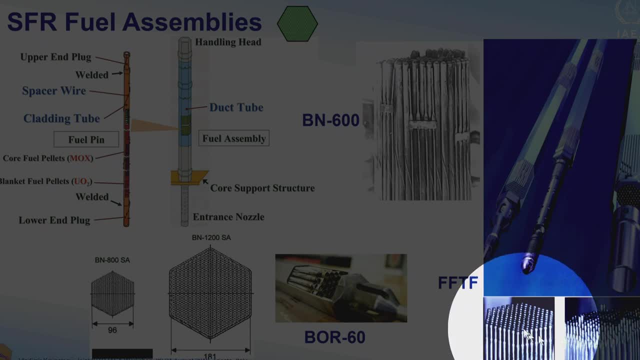 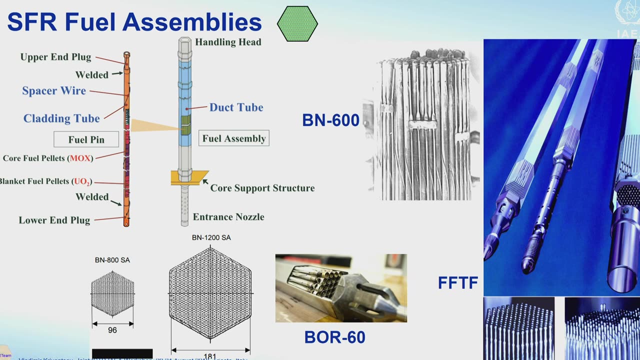 and also before irradiation and after irradiation. So, and one of the features of the fast reactors, as you know the subject, the fuel there is on the high burn up to to this high burn up. 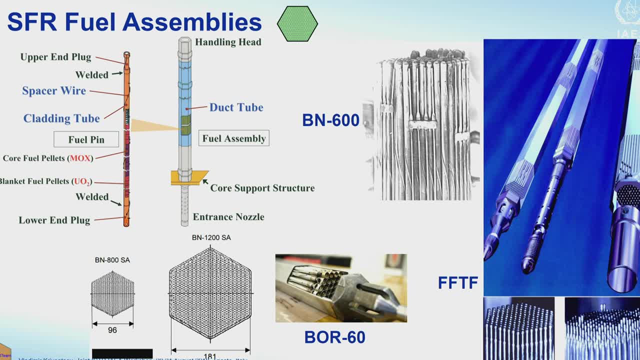 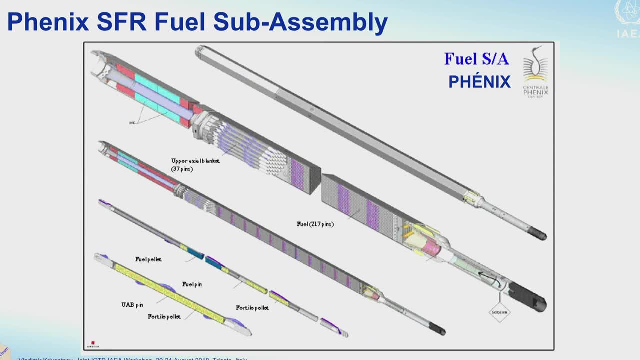 is high irradiation and that makes also huge damage of the structural materials and fuel and also for the coolant. even Coolant circulates or can be substituted. This is fuel subassembly. 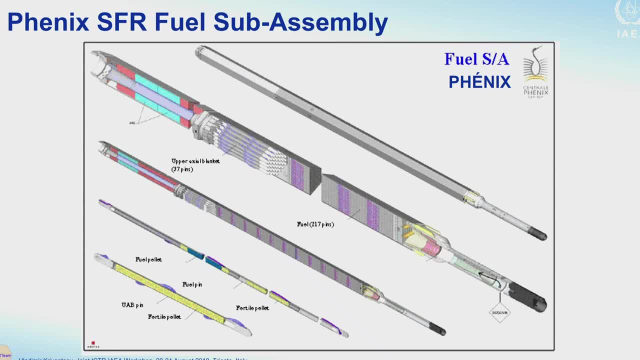 of the Phoenix reactor operated in France for several dozens of dozens of years and was shut down recently, relatively recently, providing in the final stage, several- they did several- experiments and some of this experience. 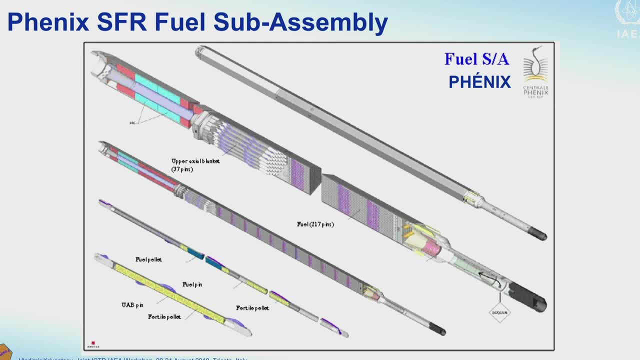 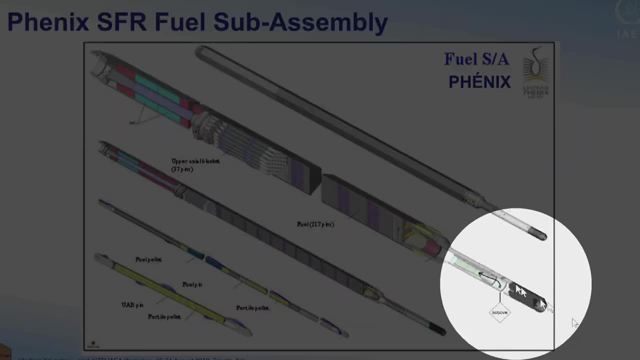 were provided as a benchmark test also for the IE benchmark research projects. So this is like more complicated, because they didn't didn't look very common but could afford. for example, you have the fuel pin. 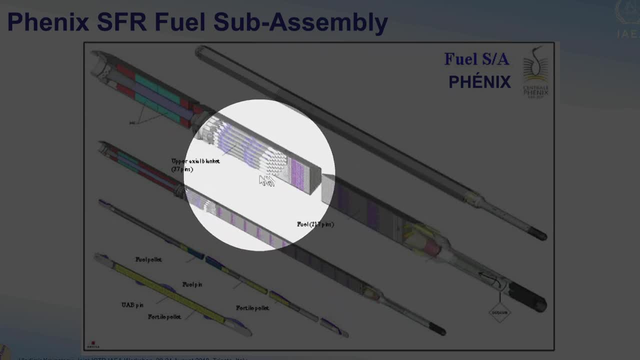 it's like usually hexagonal array collected here, but then in addition you have in the same hex scan of this tube rapid. they have breeder area, let's say vesicle tubes. 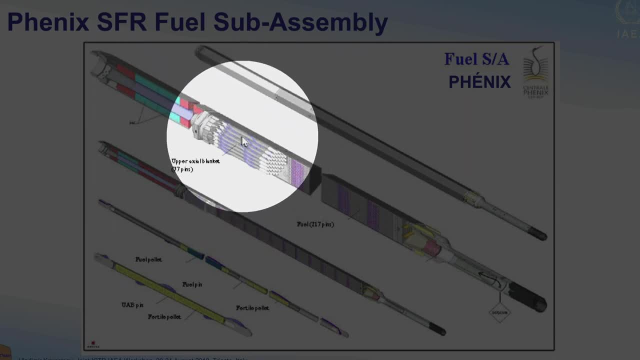 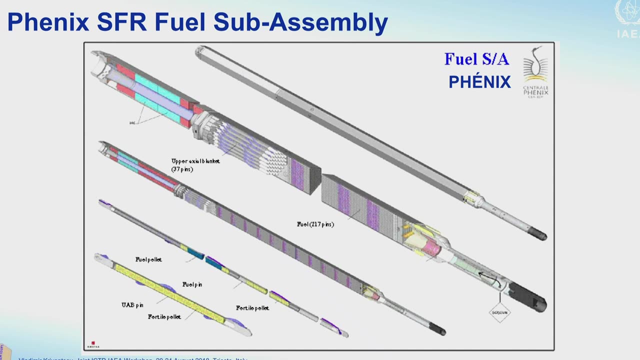 relatively shorter and this was breeding area in and in the axial fertile in the axial blanket. So they could be different shapes but still more or less the they follow the similar configurations. 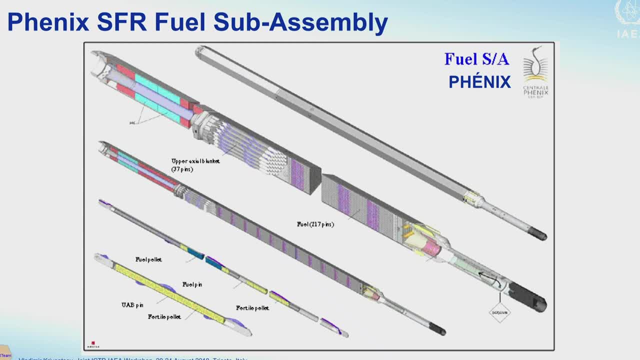 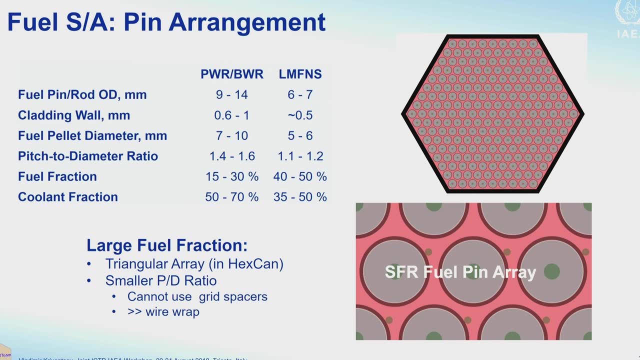 is a cylindrical square, sometimes for the for the water reactors, and hexagonal shapes with pins inside in triangle array, and this case they used to to give a space, the gaps between the pins. 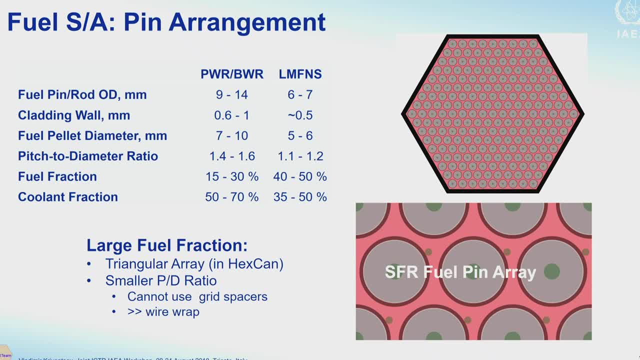 we use via assembly, we can use grids. So this slide compares the arrangement of the pins for the different. I mean for the more or less average average values or range for the. 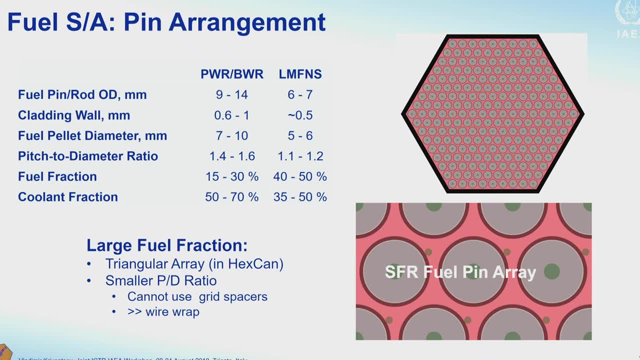 pressurized for the water reactors, both pressurized and boiling, and for reactors cooled with liquid metal. So liquid metal cooled fast neutron systems, LMFNAS. there are several abbreviations. 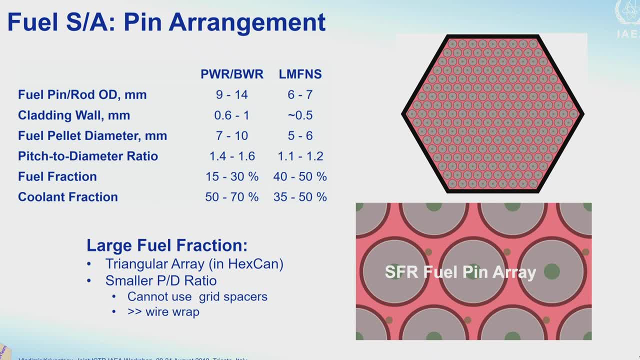 that sometimes you are lost there. but, and like SFR, LFR, LFR assumes different but general- is liquid metal cooled fast. neutron systems. neutron systems because we want to include. 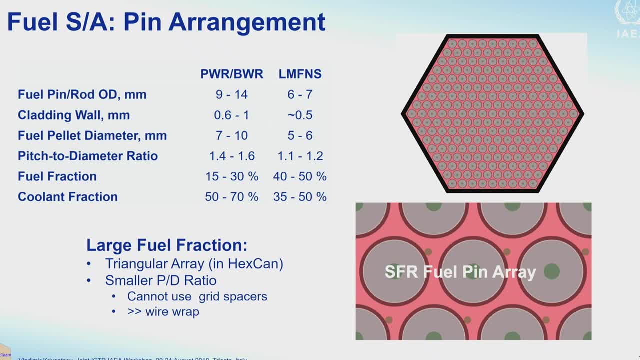 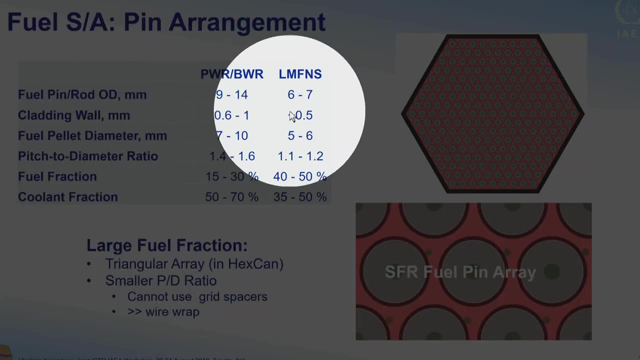 not only reactor, but reactor plus reactor, which we call system also, and it's not necessary include fuel cycle, but could also include reprocessing facilities, and so that's why we have this terminology. 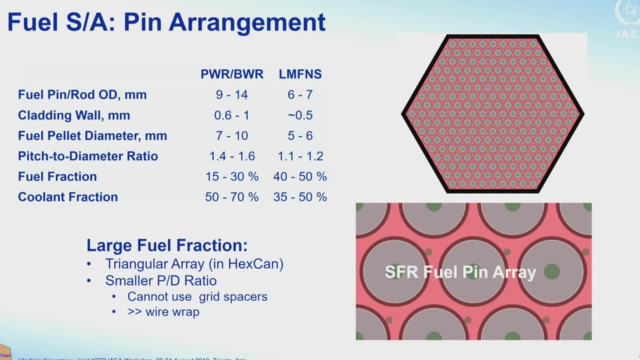 a little bit not okay. So what we can see here? the fuel pin or rod diameter is essentially lower than for the for the water reactors that means the area, if you have. 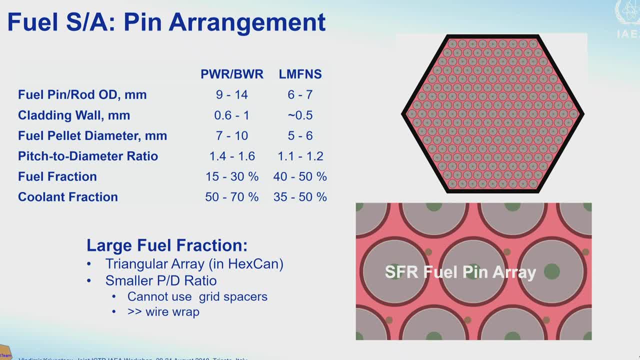 two factor of two in the size, so in area you have more or less four. so area of the cross-section of the fuel pin and pellet as well is four times lower. 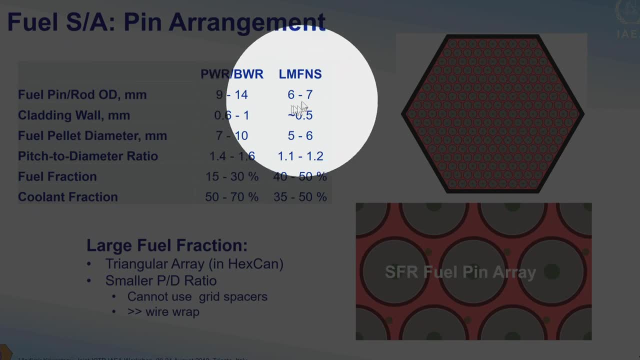 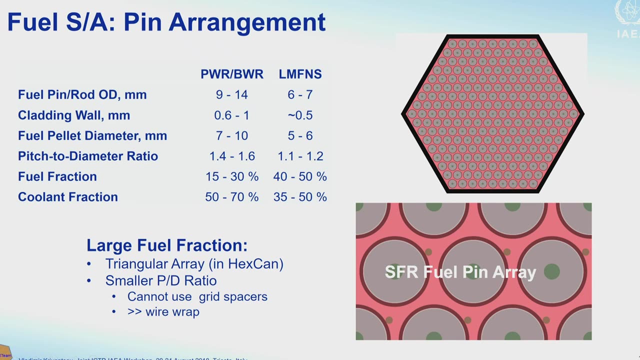 than in in in water reactors. so the cladding is also smaller. the more most of material will go to the wall, and the is already too thick, so normally it's about: 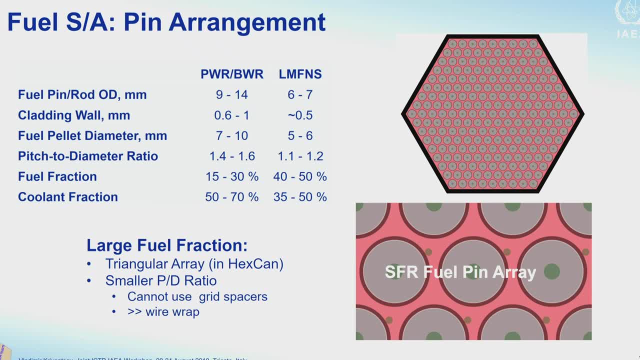 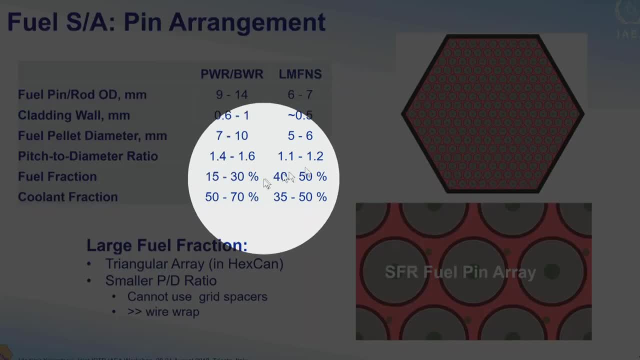 0.5 millimeters the thickness of wall, and that why the structure materials for for the wall are very important in this case, and and the array of the pins is much denser. so 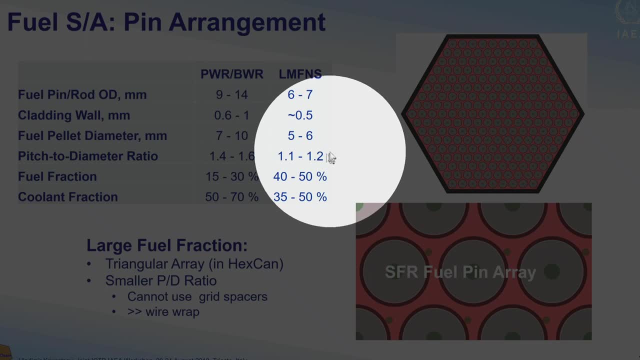 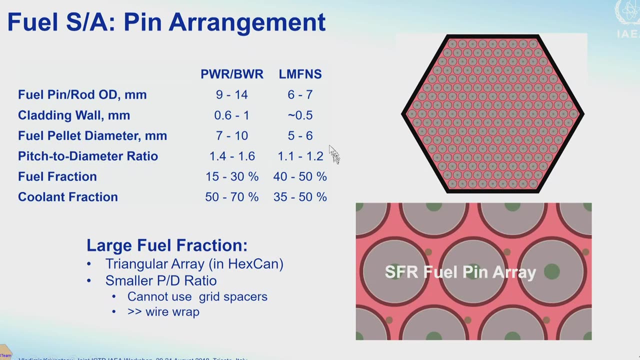 if for the water reactors you have 1.4,, 1.6,, more or less this interval, so 1.1, to 1.2, because we want to have more fuel and to reach the 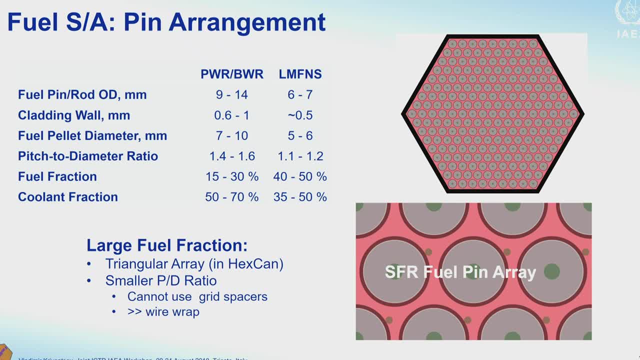 more power density also as well, which is because of the flux, as I believe Massimo explained it- why we need much higher neutral flux and it results in much higher power density for the 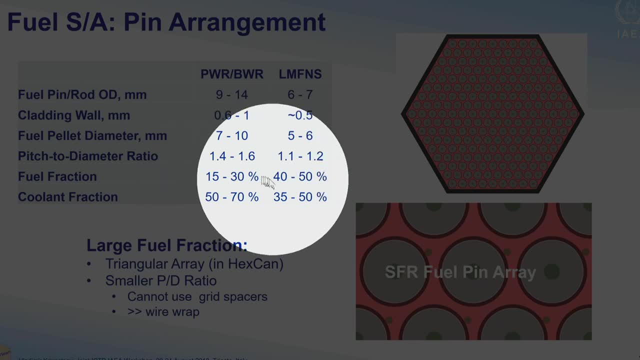 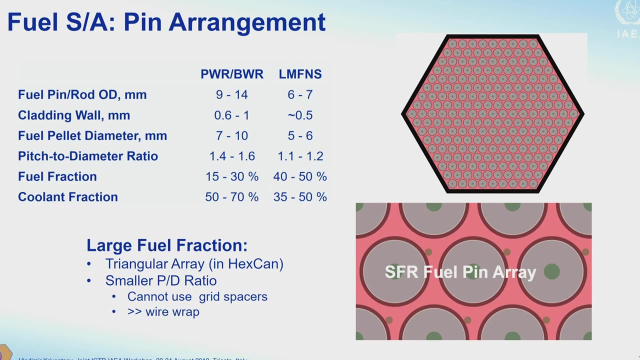 fast reactor to be more effective. and then the coolant fraction is: we need better cooling or to provide some cooling possibilities, which is better? because the coolant fraction in such geometry and for such reactors- 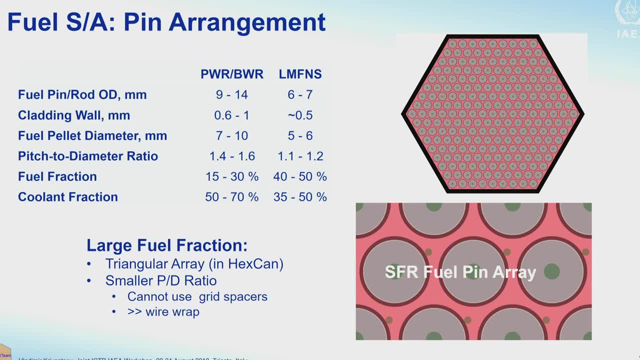 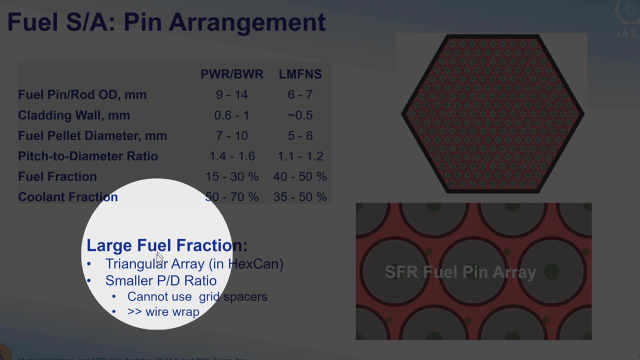 is much smaller. so as we want to reach the larger fuel fraction we have, we arrange it in the most, let's say, compact way, in triangle array, in hex can tube, and we want smaller. 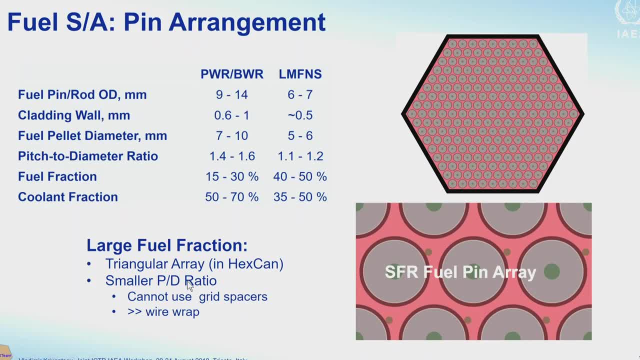 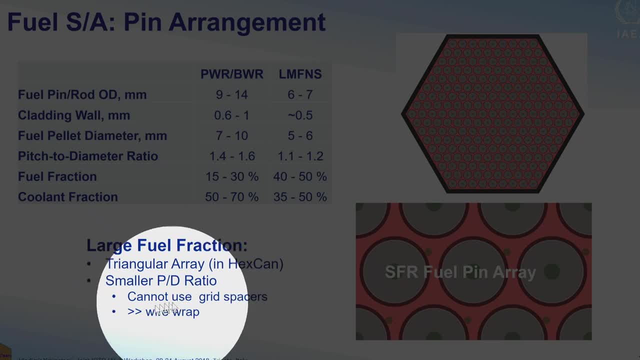 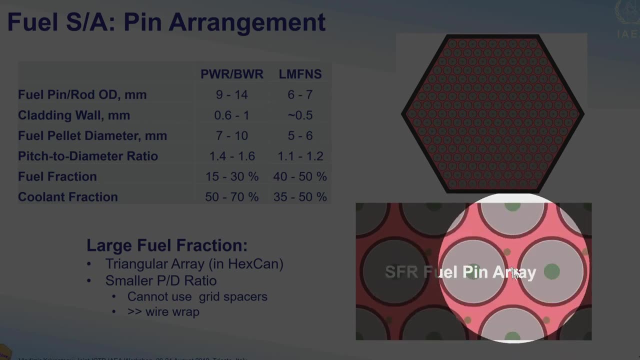 pitch to diameter. excuse me, that gives us again higher fuel fraction. but in this case we cannot use grid spacer and using wire to to to control or to keep to to keep the gap. 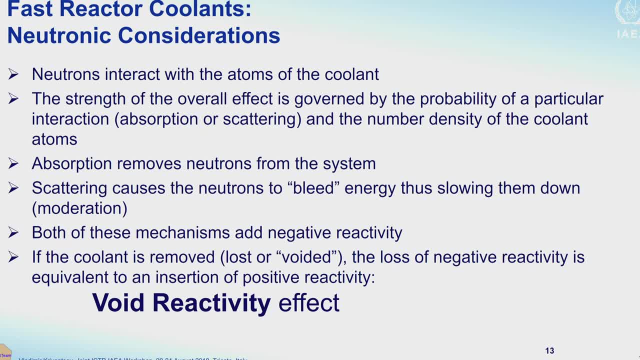 between the fuel pins inside the reactor. so now again, let me repeat basic facts: why we need, why selection of the coolants for fast reactors is like this. so we know that neutron interacts. 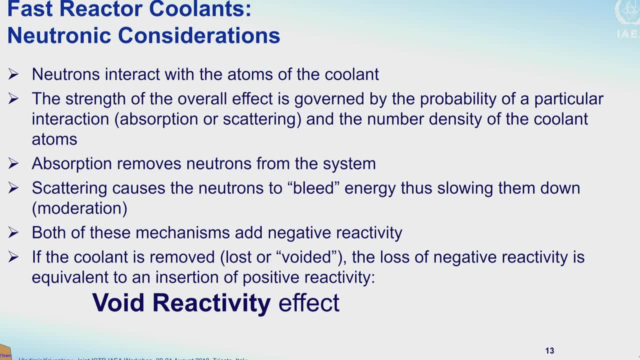 with the atom of the coolant and the effect of this. which coolant is governed by the probability of a particular interaction? is absorption of scattering, and how many atoms of the coolant you have in your system? 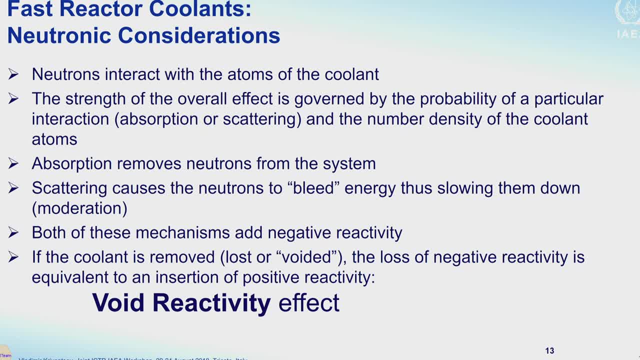 absorption. remove completely removes neutron from the system. scattering it's more or less results in moderation and all this mechanism add negative reactivity. so that means if you have, if you. 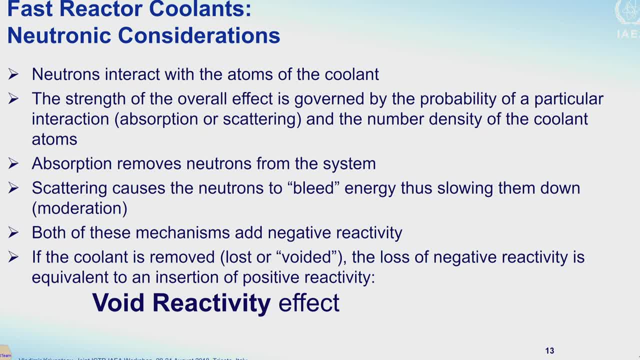 have coolant, your reactivity is decreasing if you don't have coolant, or it's voided, as they say, actually evaporated in practical. so you have positive, positive reactivity effect and 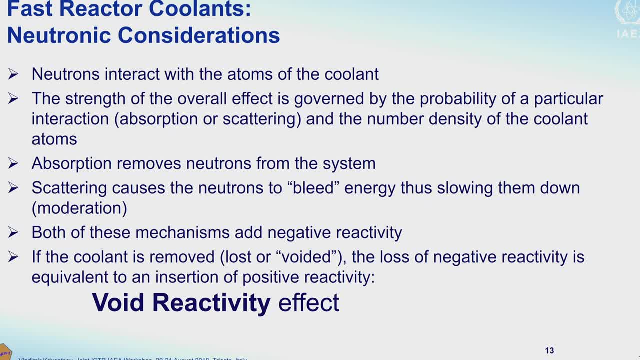 this is very important thing to be considered in the fast reactors. we also say that that the probability of the this positive void reactivity and the probability of the accident that will result. 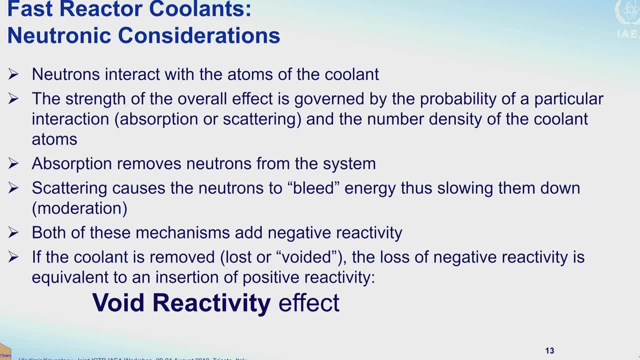 in positive release of this void reactivity and power excursion that could damage the core. it's because the in fast reactor fuel arranged as core arranged is not, is not in it's. 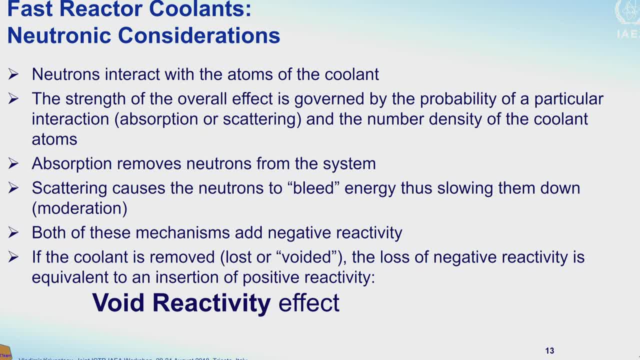 most critical configuration means if you have a fuel and you rearrange again the coolant and other components. if you remove the coolant and for, for instance, compact the fuel, it will be more critical than 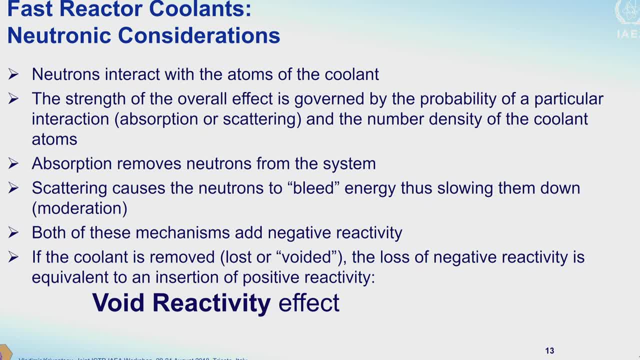 standard configuration, unlike in water reactors, where in water reactors as water, if you remove water, it's less critical configuration than with water and that the general from the general consideration is, as reactor core is not in. 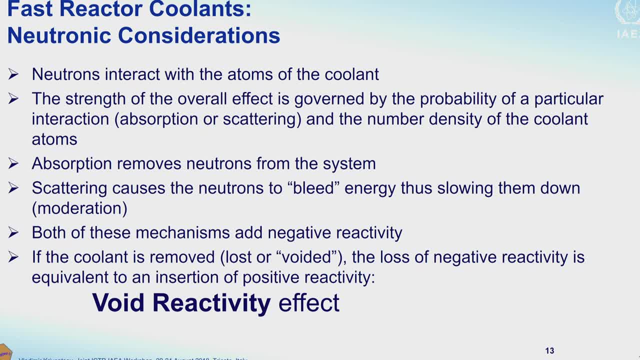 it's most critical configuration: the, the, the the might be situation, what it will be more critical than it's a normal and then we should control and take care and make, take measures. 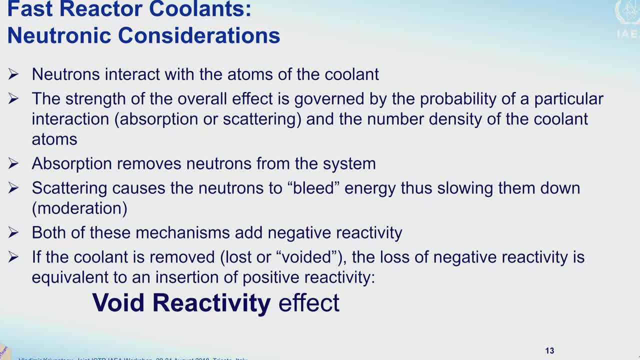 that the core will not go to the more critical configuration as it for it's normal condition and void reactivity effect. it's just sink, as the designers were fighting for the years, and there are several solutions. 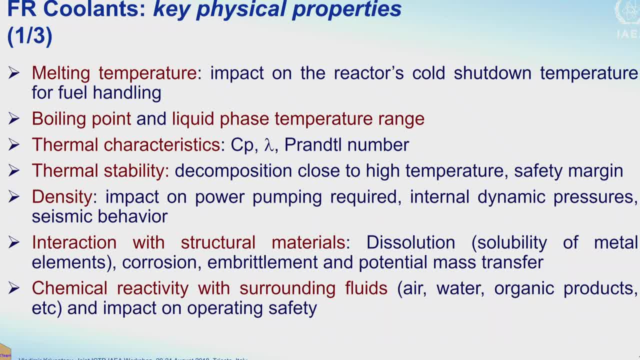 but there is no actually ultimate solution, at least for the sodium cold fast reactors. for the others, like molten salt, it's not a problem, because they have different. they don't have fuel assemblers. 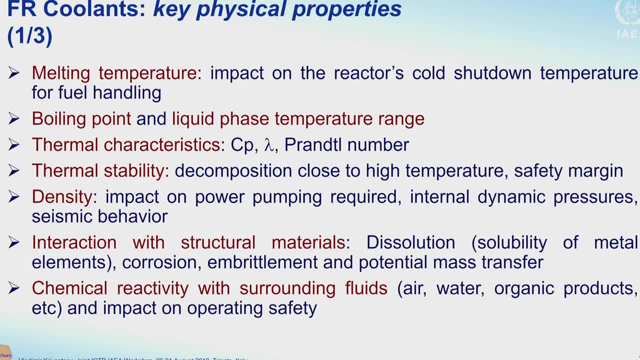 fuel rods, fuel pins and even rod bundles. okay, thus, for the, of course, the coolants, we have a several key physical properties which we should consider when we selecting the coolant. 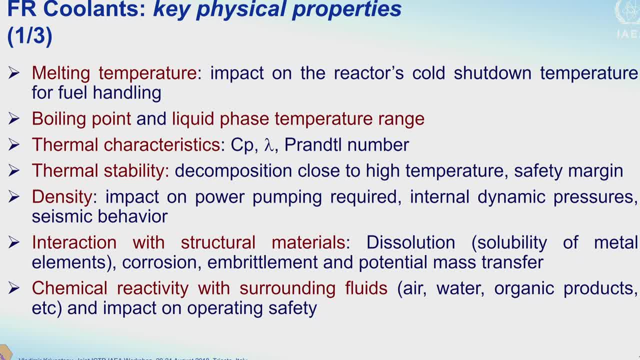 for the reactor. so melting temperature: this is parameters that should reflect that we we cannot freeze. we should avoid at least freezing of the coolant in the reactor. so the higher melting temperature: 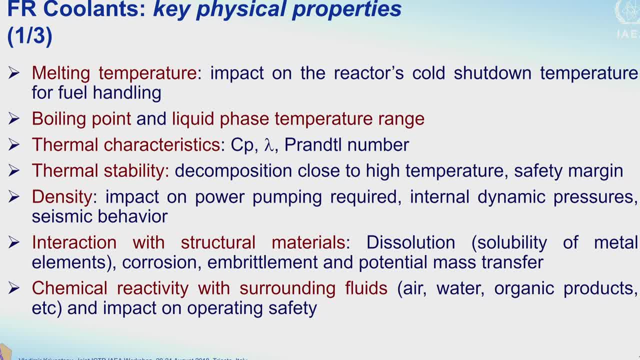 then we should keep the reactor, even if it doesn't operate in this high temperatures, like for the lead, for example. another thing is the boiling point and liquid phase temperature range. boiling point means that higher boiling point. 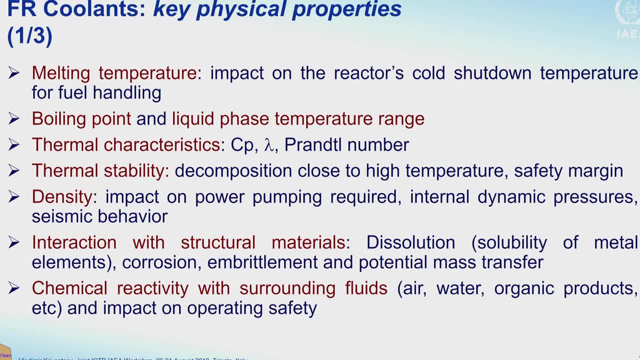 is better for us and because we can reach higher temperatures. plus, we have a range of the temperature. so, for example, in the water reactor you heat up from 270 to only 30 or 50,. 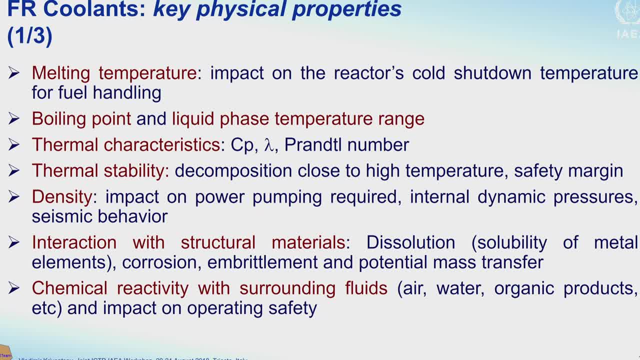 maximum degree C you can heat up water in the reactor. for the sodium cool reactor the range is much higher, at least 150, or sometimes slow, it can be even more, and that that 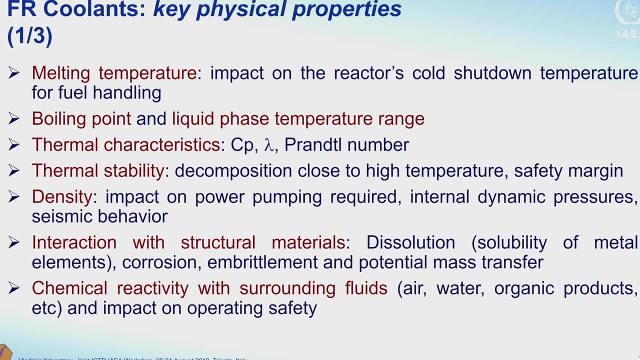 that allows you to remove more heat from the same, in the same configuration with this coolant. boiling point is also important because we don't have, we don't want to reach the boiling. that's why. 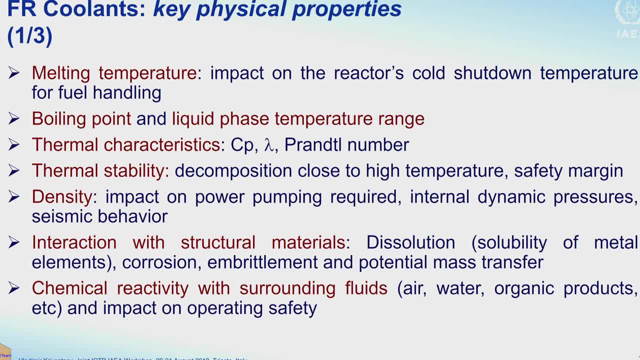 lead is, from this point, is better than sodium because the boiling point is higher. it doesn't boil and sodium could boil in some conditions. of course, thermal parameters like heat, capacity, conductivity- this lambda- 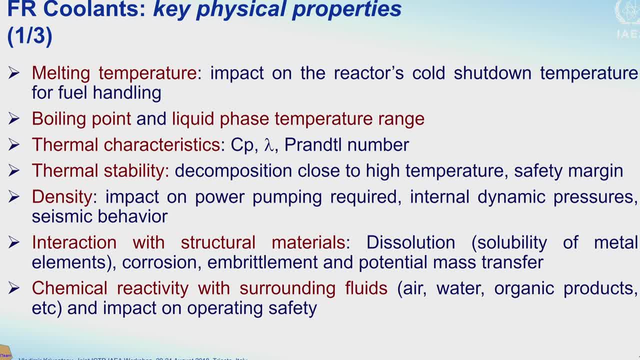 is conductivity. in different countries we use some for the conductivity we use is a lambda, okay I? I believe it's from Greece. lambda in Greece. which letter do you use for the conductivity of the materials? 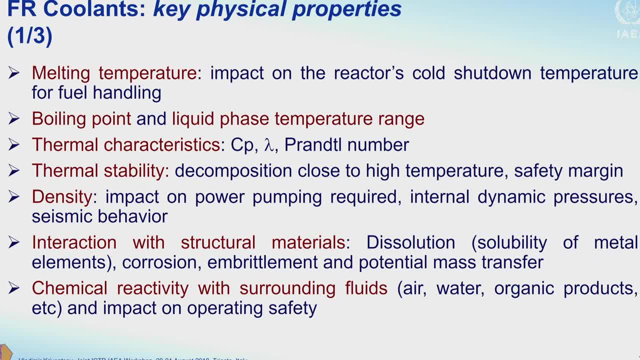 no, Greece is not here today. how do you which letter you use for conductivity in Greece? how do you which letter you use for conductivity depends on the path of Greece, okay, but 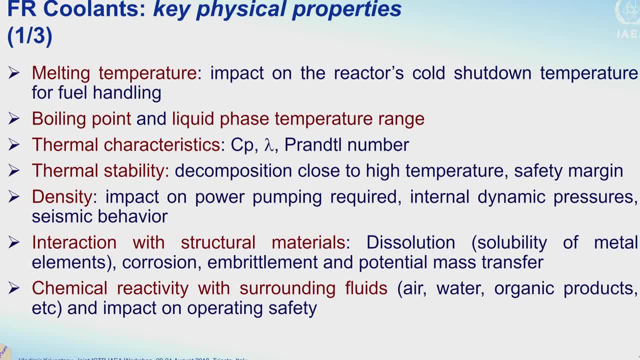 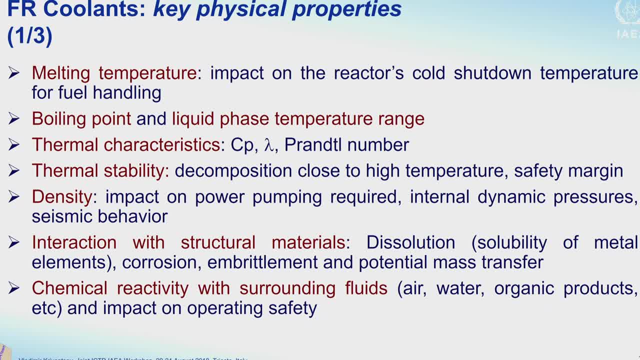 yeah, yeah, yeah, yeah, because, yeah, OK, yes, interesting, interesting message. yeah, yeah, yeah, yeah, yeah, yeah, yeah, really interesting. well, do you say, I see, yeah, thank you. 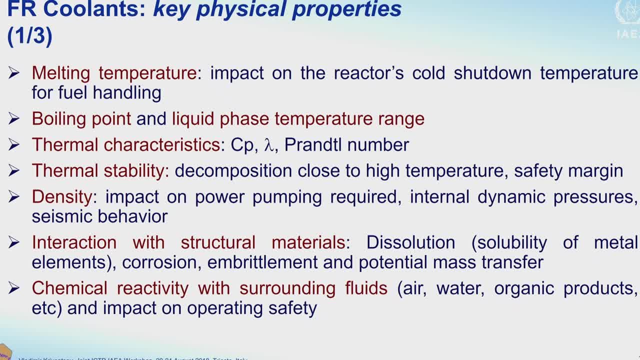 Puerto, who, and, and I am, I am. you can find very interesting facts, I mean, who is orange, and so on. Ok, another important feature- I mean parameter characteristic of the coolant- is the thermal stability. but this is more or less for the designers also. 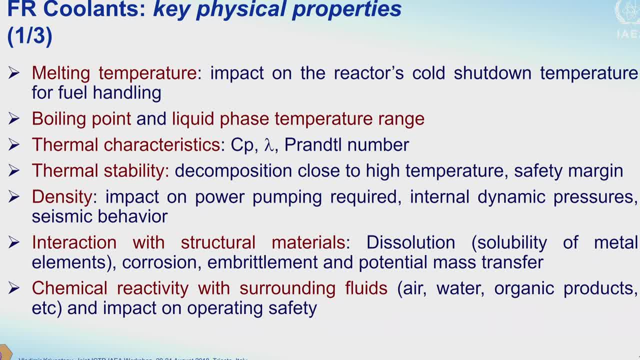 And density. Density is very important, as you understand already. it impacts how need, because the pressure drop, how much power you have to spend on the pumps to pump coolant through the core, and also not only density itself but dependence of the density of temperature, the height of the expansion coefficient. 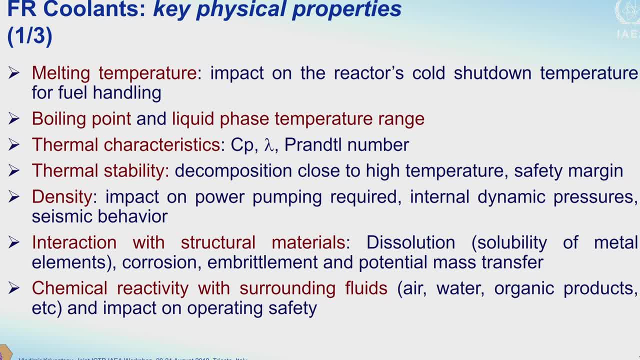 If you have high dependence, you can't rely on the natural circulation. so it provides you higher natural circulation power, which we want to always to use, to be systems, to be passive, and interaction with structure And materials. this I don't touch because it's already, it's a little bit. 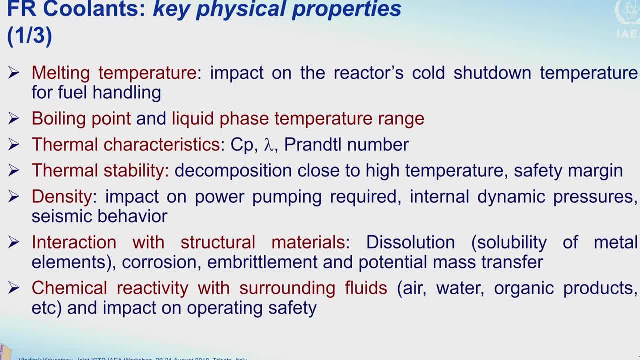 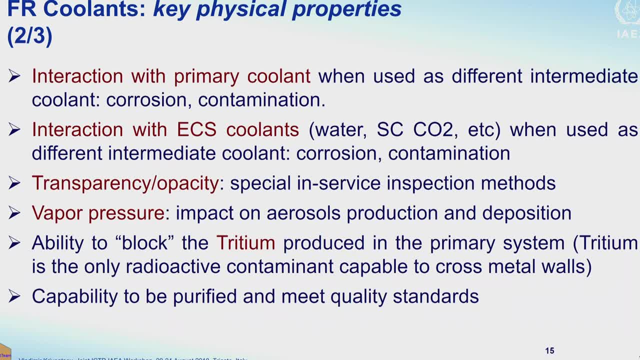 not on thermal hydraulics, which is connected, but not exactly, and chemical reactivity with surrounding fluids. That means that, ok, let me consider another. this is another key physical properties. it should be what is important. interaction with primary coolant when used as different intermediate coolant. 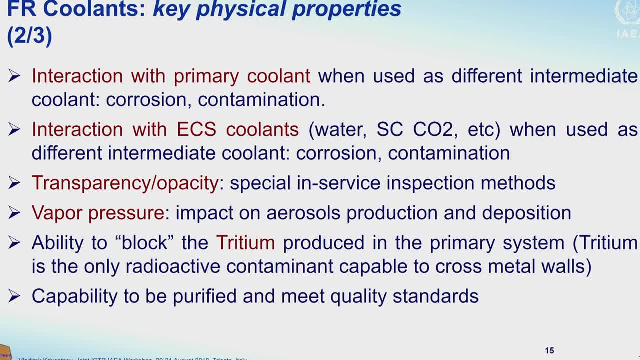 for example. So ok, this is interaction. if you have another coolant in the secondary loop, they could probably, in case of failure of tubes or something, interact, and it's also important. So that's why you don't. you cannot put water exactly. 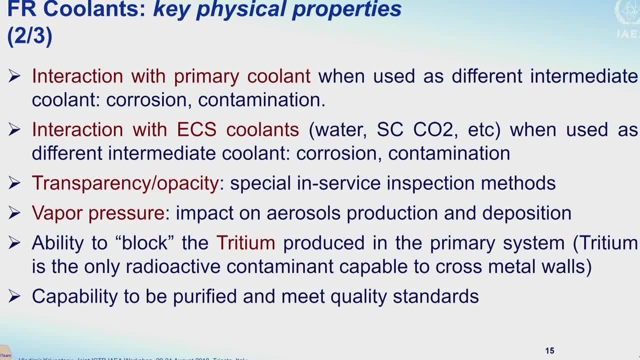 in the intermediate heat exchanger in sodium fast reactor Interaction with other coolant. ok, this is something not very related to the thermal hydraulics features, but this is general feature parameters of properties of the coolants which we should take into account, Like, for example, transparent. 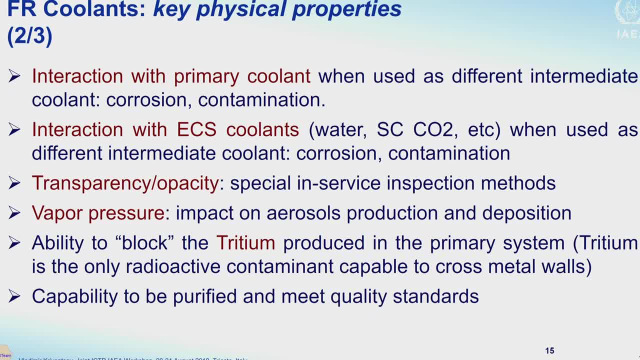 is good because it allows us easy in service inspection. so vapor pressure also, it's depends how you, ok, but it's how it's communicated, the surface communicated with the gas inside and several others I would say. 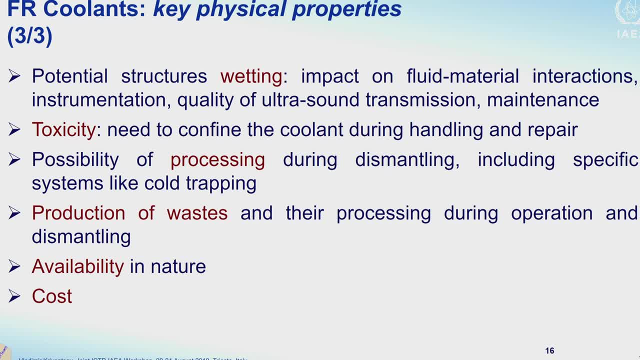 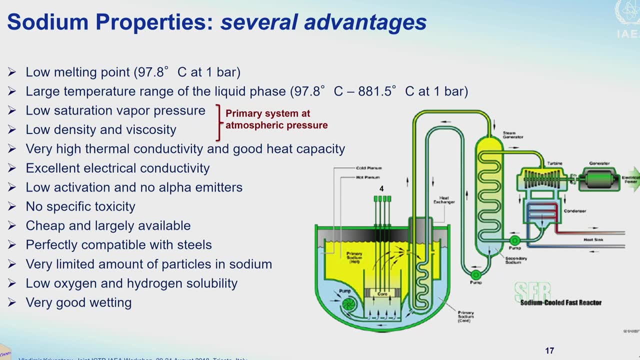 Which already Christian explained all this, so I will skip this- and availability in nature and the cost. also, We were discussing the cost of lead. yesterday Christian found lead for 2 euro per kilogram. I was able to find only for 8 euro per kilogram. 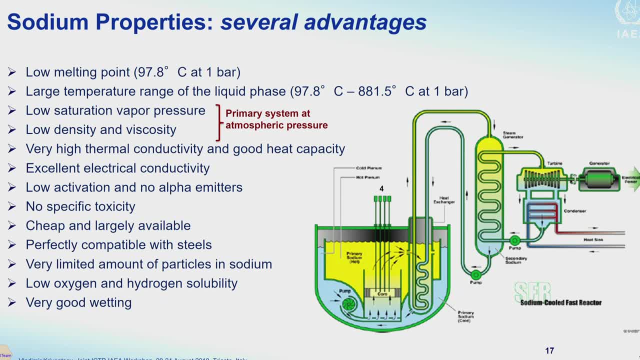 for my weights, for the, for the diving. On eBay it was all already used lead. I hope not from your. I'm sure it's not from the lead-cooled reactor, because we never seen lead-cooled reactor in nature and also artificially created before. 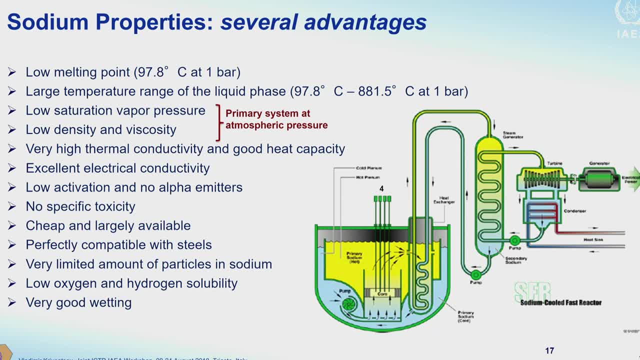 Ok, now we go to the sodium, and sodium comes first because it's most mature technology and, as you know, the first nuclear reactor that generated electricity was cooled by sodium and it was fast reactor EBR-1 in the US. it was very little electricity, but still it's a fact. 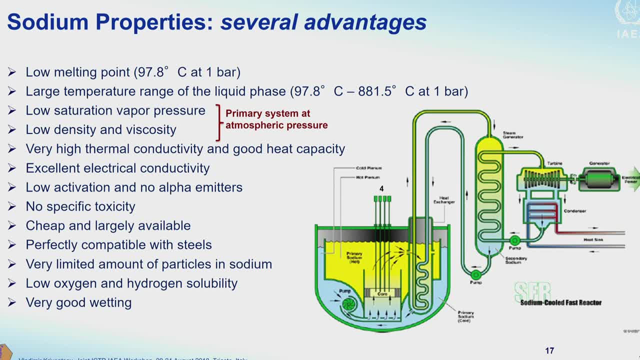 So sodium was and fast reactors in general, and sodium were considered as a coolant and type of the reactors from the very, very beginning of the nuclear era, I would say. and the reasons is obvious, because sodium has low melting point. it's about 100 degrees C. 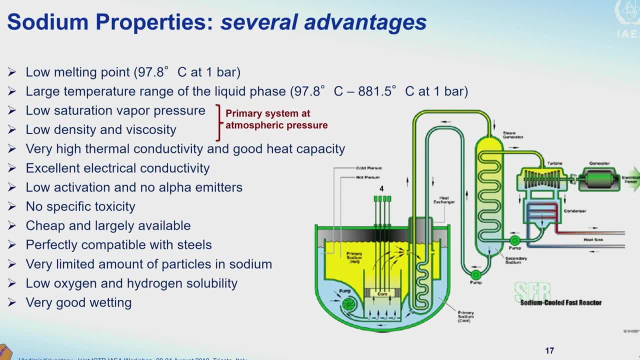 at atmospheric pressure. so that allows you don't need to spend a lot of efforts, let's say, or make some features to keep it in the molten conditions. And it also has a large temperature range of the liquid phase. it's about 800 degrees C. 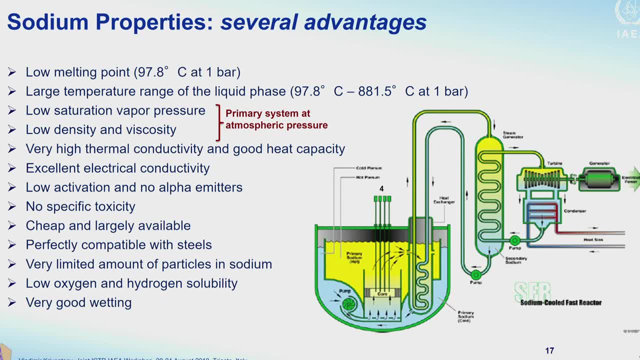 then imagine that you have a huge range to heat up. In practice, of course, we use much lower. it's 150 or maximum 200 degrees C. It's heating in the core, but potentially you have like almost 800 degrees C. 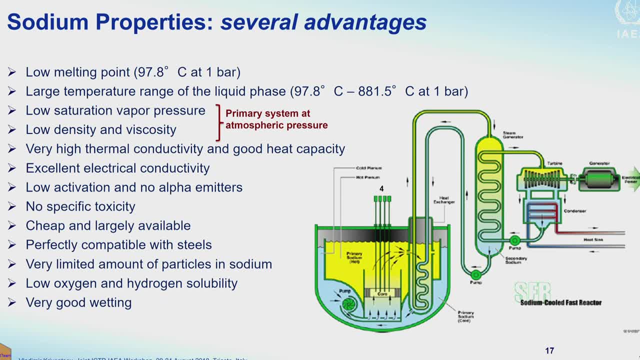 And also it's for the accidental condition. it's very important. It has a low saturation of vapor pressure and low density and viscosity and that allows us also to at least saturation to keep primary system at atmospheric pressure. so there is no potential energy in the core. 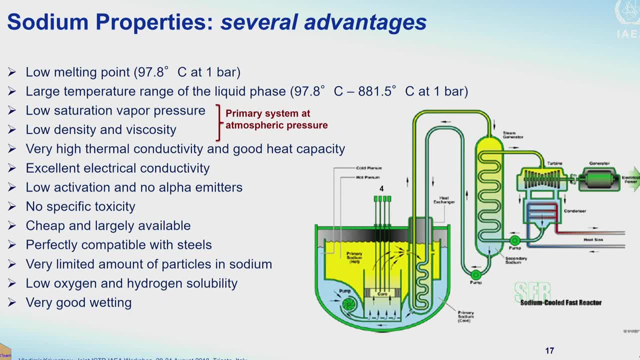 And of this kind of compression collected in the coolant which can be released in case of the accidents. So sodium has also perfect, very high thermal conductivity and good, relatively good heat capacity, which is a few times less than water, but still very good heat capacity. 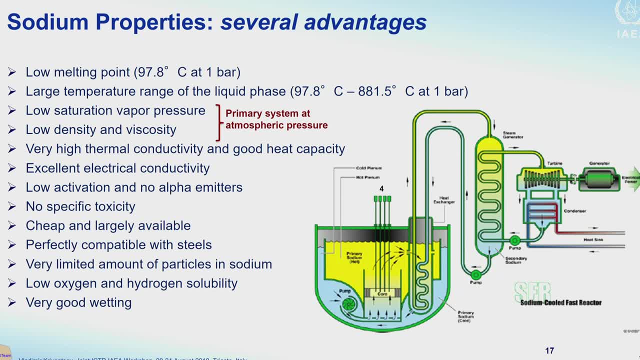 Some other features which I maybe skip here Also. it's not written here, but it's available as you will know also, and we observe it in this- salty water. sodium is available, widely available and easy to extract from from from the elements in nature. 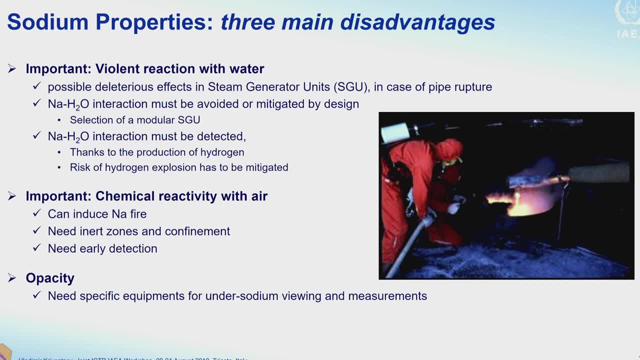 However, with sodium we face three main drawbacks. It's to its violent reaction with water and with air. So with water you say that it's you always. should you all know that this is violent interaction with water? 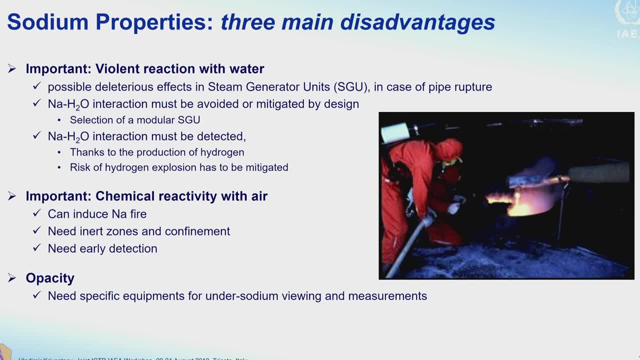 in many cases, But different also in simply for this reason we cannot make intermediate heat exchanger with water. we need additional cycle, either with sodium or maybe with other, with other material and coolants which are not interact violently with sodium. 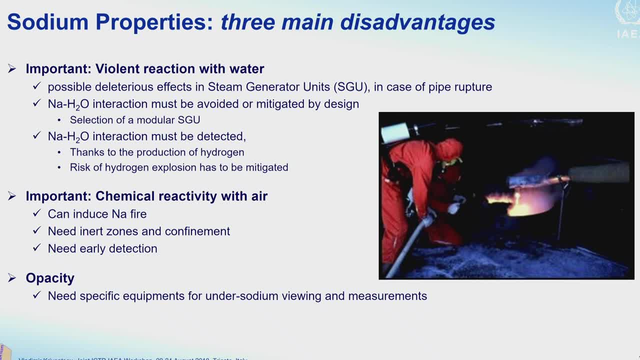 And that makes a lot of complications and chemical reactivity with air. that can initiate the sodium fire, which is actually not. if if you look at the sodium fire, for example on Monju, they have a museum of the accident. 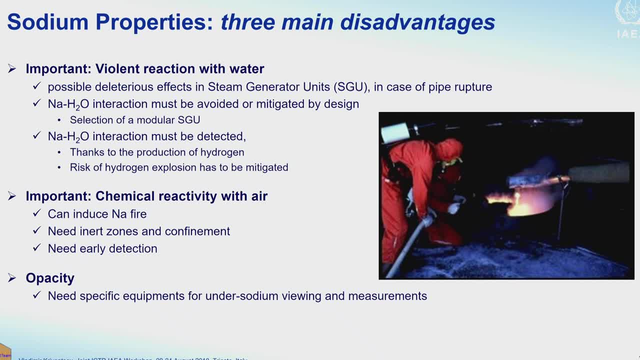 and which happens, the sodium fire, which happens in 1995,, I believe, and in that case it was sodium leakage that resulted and sodium interacted with air and it was sodium fire. maybe not that actually stopped this Monju program. 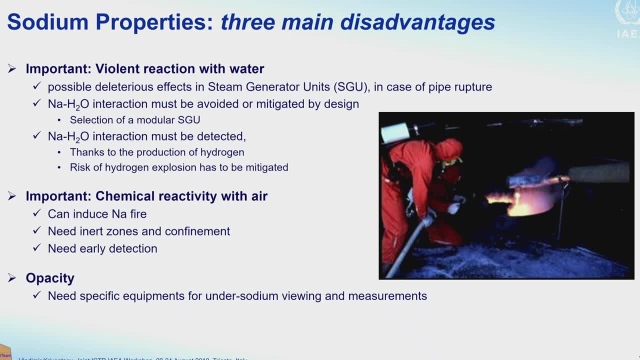 and affected a lot the Japanese program of fast reactors and. but in that museum I saw it was examples of sodium fire. It's really a very, very small fire. If you have your lighter it's much bigger, I mean. 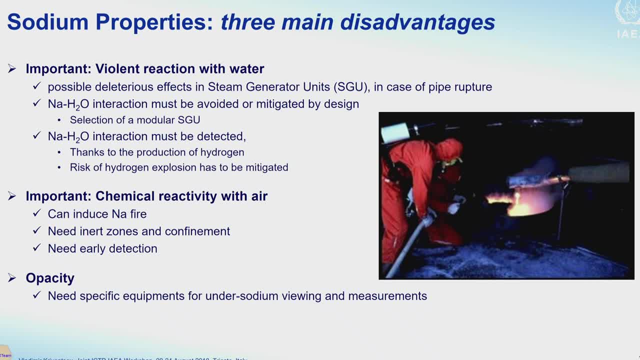 comparison And if you imagine the fire of the gasoline or or other you know materials, it's it's very small fire, but still it's essential and also it can be initiate. it doesn't need any external initiator. 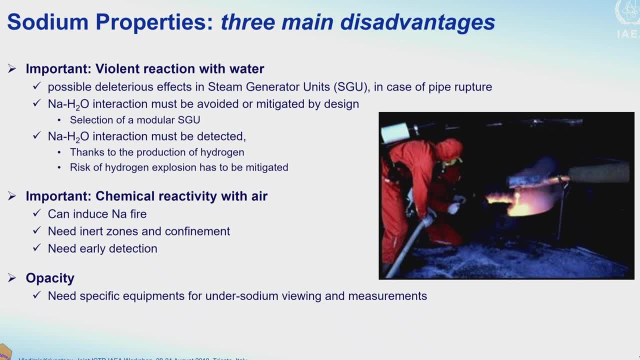 or ignition. It can go and for the several conditions which is can be easily reached, it can be ignited automatically in the sodium. That is a problem that we can do And also the sodium is not transparent. that it makes 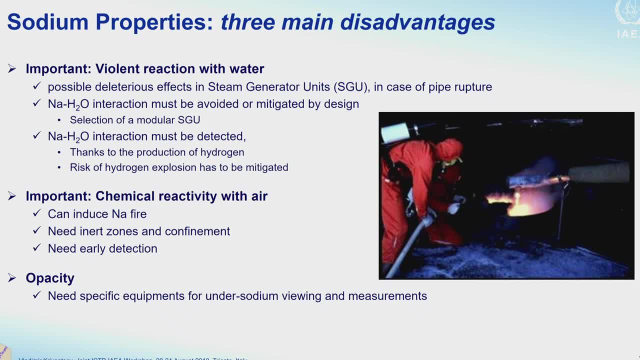 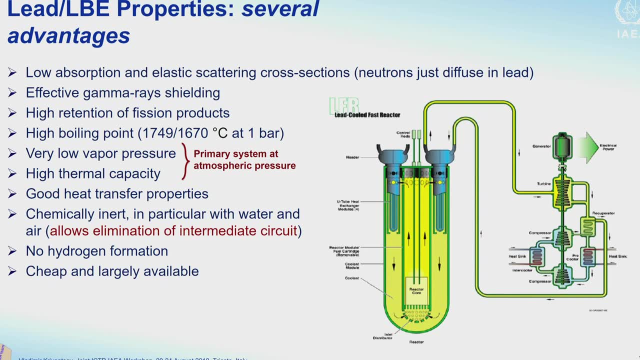 but it's smaller. Then we need special measures for the in-service inspection, and so on. So, knowing the disadvantages of sodium, people were thinking how to how to replace sodium with maybe better coolant, In this case lead or lead bismuthotectic. 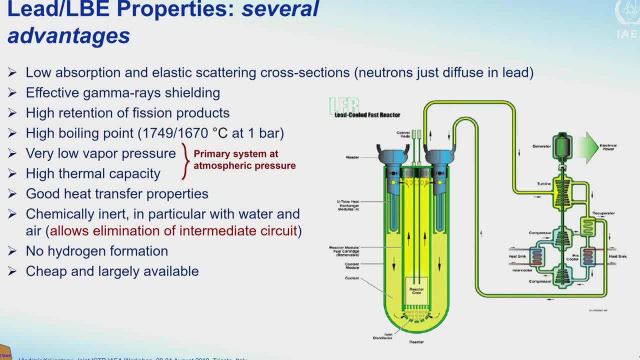 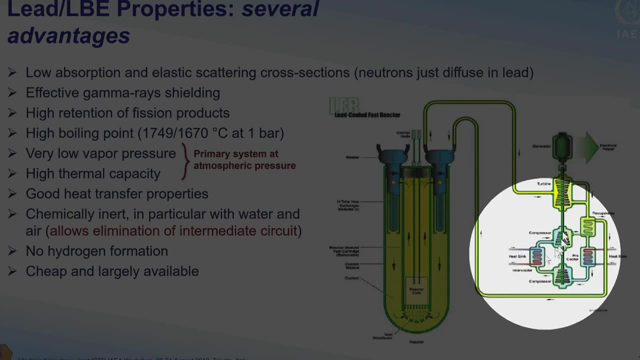 were proposed as a coolant. and you see, since we don't have problem with violent reaction with water or with air, so we can eliminate intermediate heat exchanger and inter-secondary loop. So we have only two loops here, so water can go exactly. 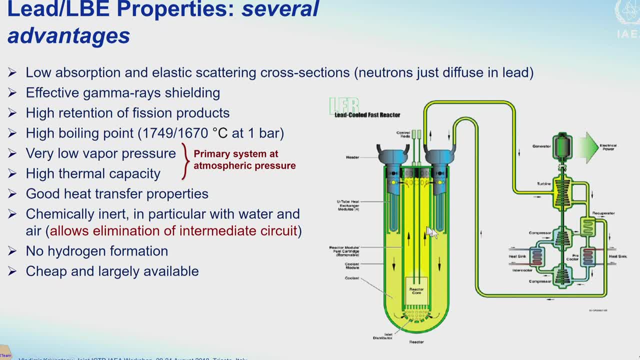 directly or gas, for example, to, to to the inside the reactor vessel, which is could be also loop type or sorry, pull type or loop type, and that is very good. Main reason why we use lead: 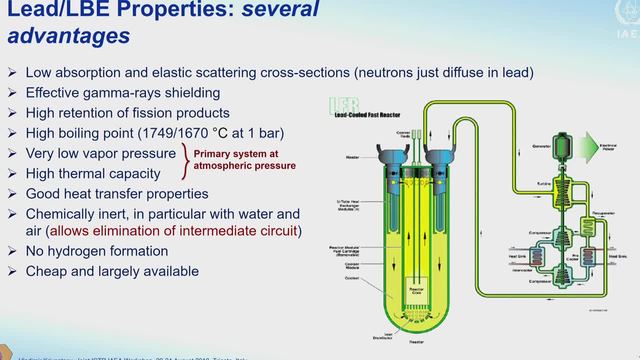 There are also neutronics. parameters are fine. Also with lead you have high boiling point. It's much higher than also even for the sodium, So about 1700 degrees C for the lead and even higher for. 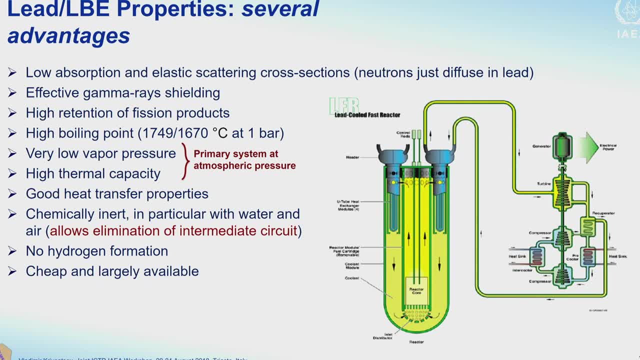 also a little bit lower for the lead bismuthotectic. Again, it's low vapor pressure and high thermal capacity and we can keep primary system at the atmospheric pressure because of that. So no potential danger from the. 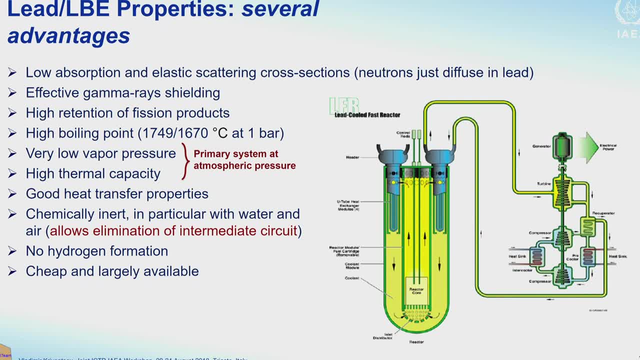 from the energy of compression stored in the system. It also has good heat transfer properties- Not that very good as of sodium, but good enough to be good candidate for the coolant- and it's chemically- relatively chemically inert with water and with air. 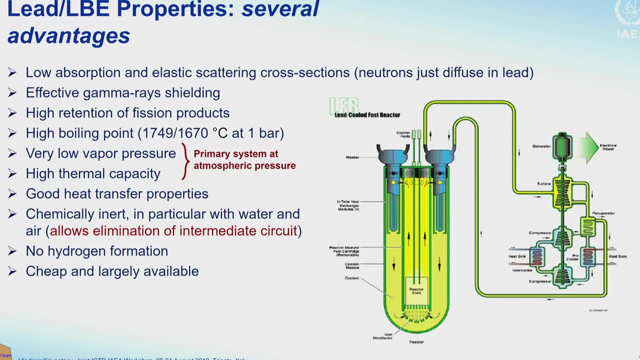 So that's main two drawbacks of the sodium I eliminated. It doesn't form a hydrogen, unlike sodium, by the way, and it's cheap and largely available. On the bismuth, for example, we say the bismuth is not very available. 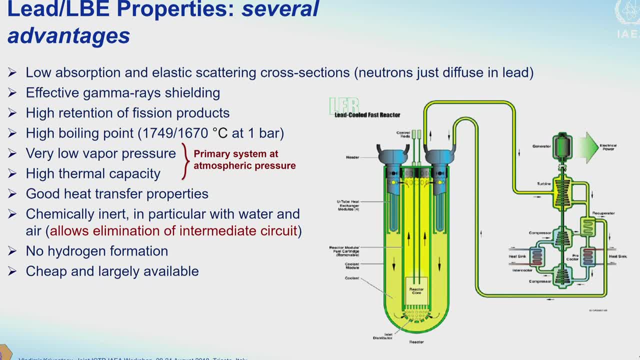 only few suppliers, but I will give- I don't know myself, but I will give you also comments on Tashinsky, who is a lead bismuth was used, by the way- experience in the old type of the Russian submarines some success. 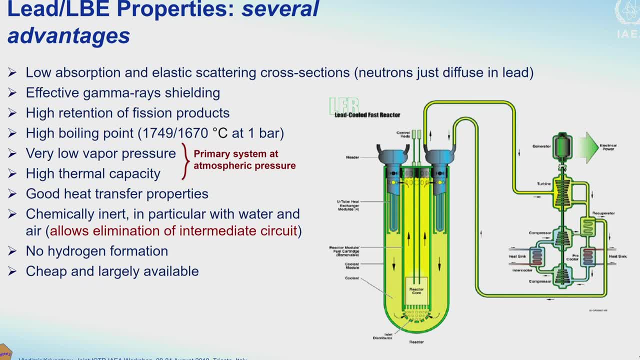 and as a grandfather of the lead bismuth reactor, Georgi Tashinsky explains that bismuth is not very available because nobody needs it. Once you will have it by demand, they will definitely deliver as much bismuth as necessary for this. 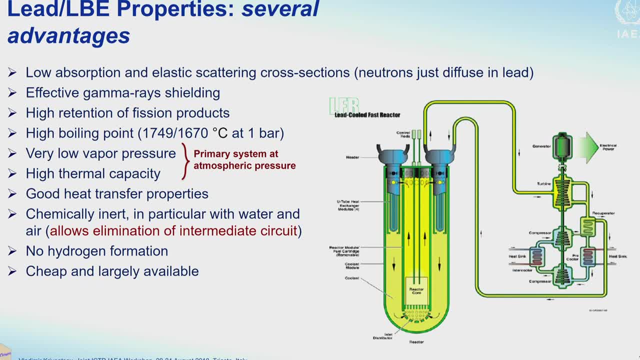 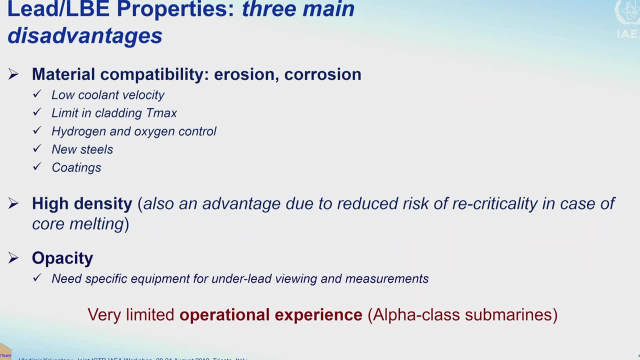 So it's not a problem, at least from his explanation, and so we say that both material are cheap and largely available as well. However, with this lead and lead bismuth, we have three again main disadvantages. So first of all, 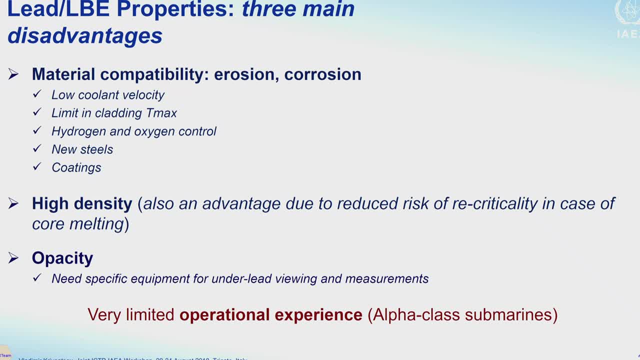 it's compatibility, erosion and corrosion. So let me confirm that if you have there is an oxygen concentration, you have to control very carefully the oxygen concentration in lead or lead bismuth tactic, because if you have a lot of oxygen it will form the oxide layer. 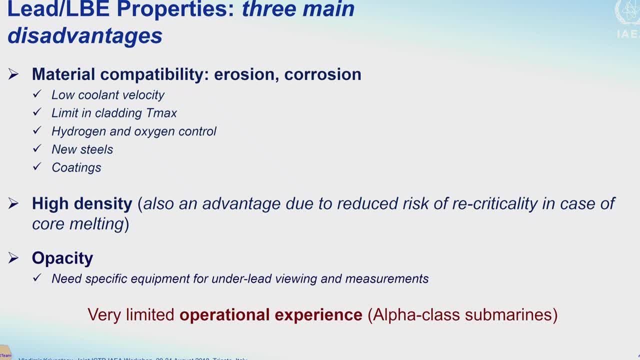 which we want to avoid, And if it's low oxygen it will eat metal from the steel or maybe other metals from the cladding, And also we want to avoid Then to operate for the operational range. you need to keep the oxygen concentration within very narrow limits. 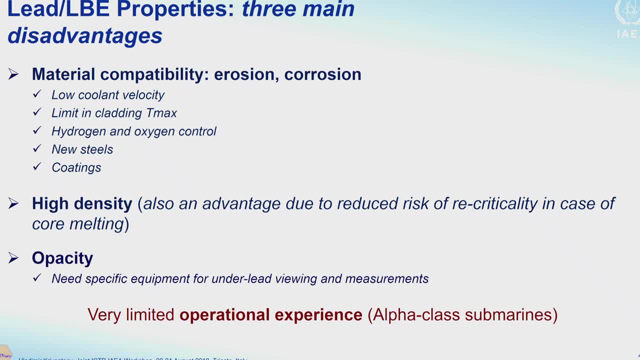 And this range also depends on the temperature. Let's say, for the low temperature you have, I believe, you have one range, and for the higher temperature you have another range. So you should, let's say, in the startup. 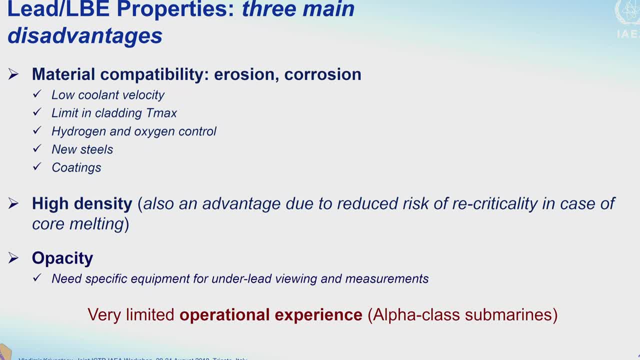 you should keep one control, one concentration of the oxygen, and for the normal operation it's higher. This is very difficult and pretty complicated And this problem is more. this range is narrower for the lead, pure lead. So for this reason, 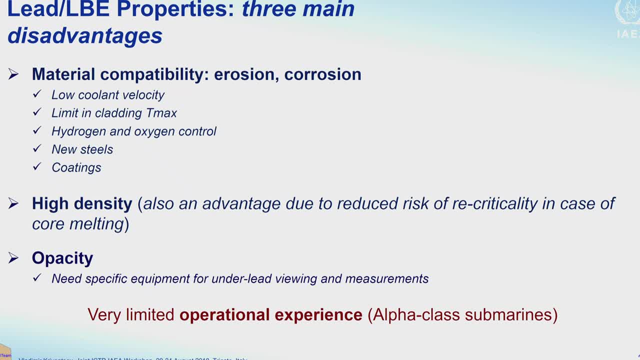 lead bismuth tactic is considered better And but still it's one of the main problems. Also, both have very high density, like 10 times more than water, And then it's for the pumping and for the. you know. 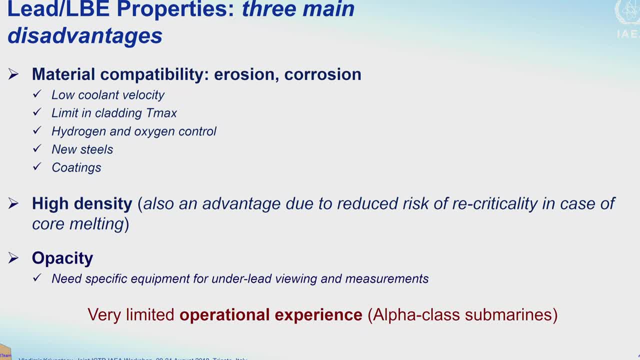 for the managing is this huge amount of this heavy metal. It's very complicated, but it also has an advantage, For example, like local roads could be sorted from any side, or because they can flow up. And let's say: 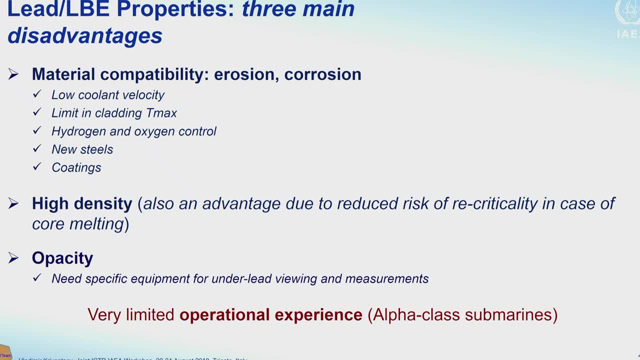 density of this, of the lead, lead bismuth, is compatible with the density of the density of the fuel uranium oxide. And then, as the pieces of fuel can float, they don't float up or don't collect it on the down. 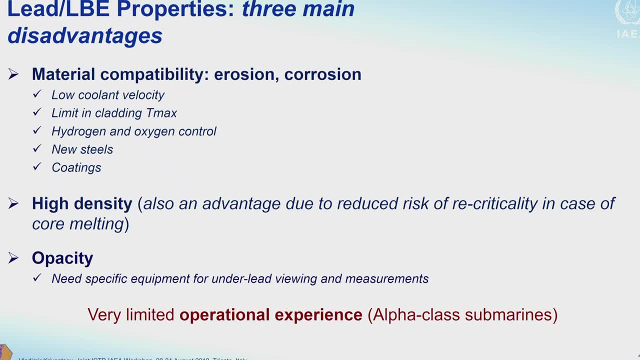 down in case of the accident of the zone, but of the active core, But then can be more or less mixed within the reactor going. I'm talking about this core disruptive accident, core meltdown now, So that is also somehow could be benefit. 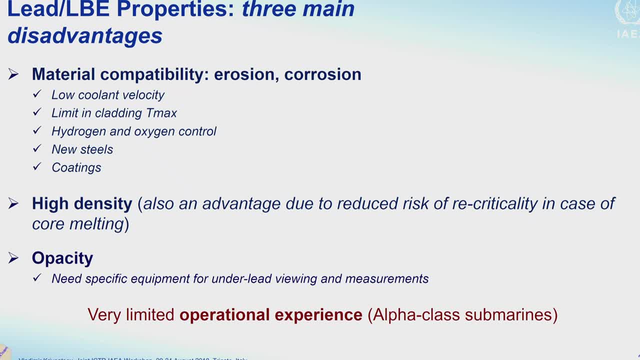 Again, opacity is zero. You need special measures for the in service expansion And main difference between lead in this coolant and sodium coolant, as that we need we have, as with sodium we have like 460,. 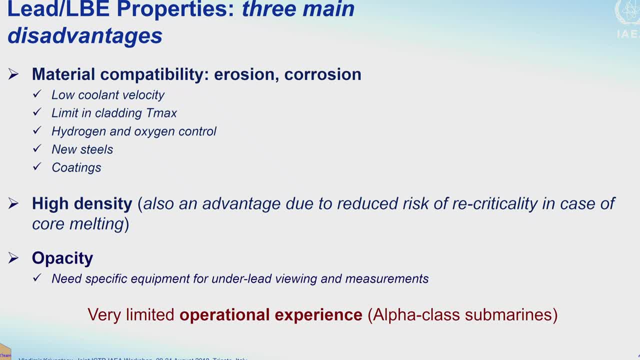 approximately years of reactor years in operation And with mature technology which was developed in many, many countries with lead and lead bismuth, we have very, very limited operational experience. However, since this big interest to this material, 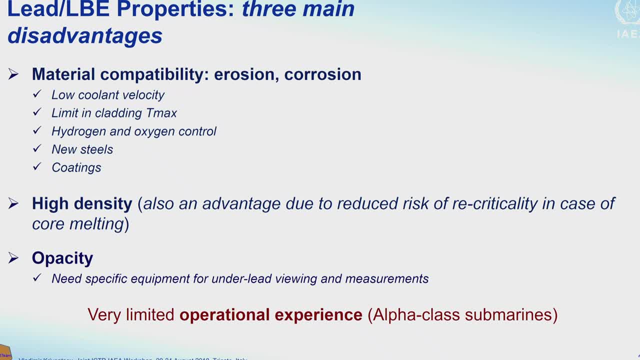 in last 20 years. we have also many, many experiments on lead and lead bismuth in different countries And we have a huge database on properties. already- And actually when we created in the IEA, we were producing the. 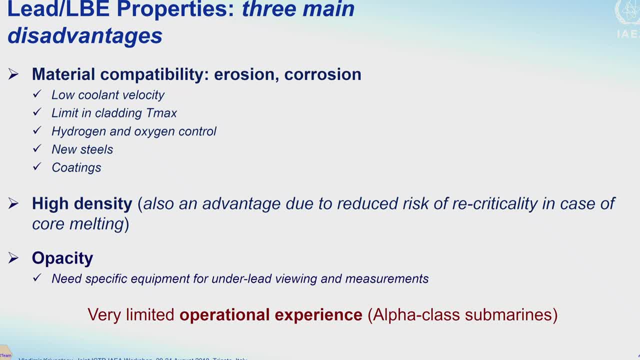 data online database on the on the experimental facilities for the liquid metal Fast neutron systems, We learned that actually the number of facilities devoted to the sodium is approximately the same as number of facilities devoted to the lead and lead bismuth reactors. 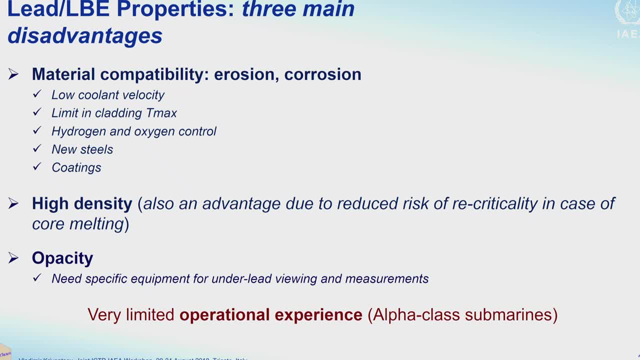 Of course they are sometimes smaller and they're new, I know- but in numbers they're the same. It shows a growing interest to this coolant and we know there are many enthusiasts who are trying to. 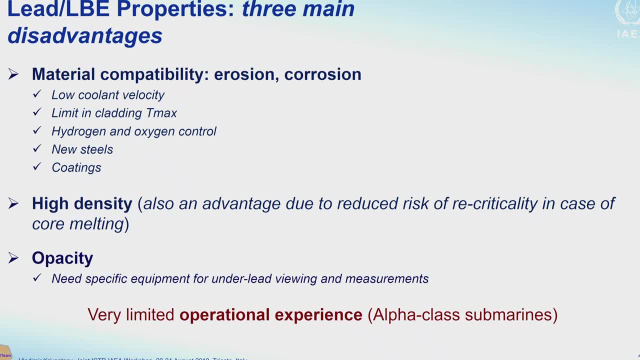 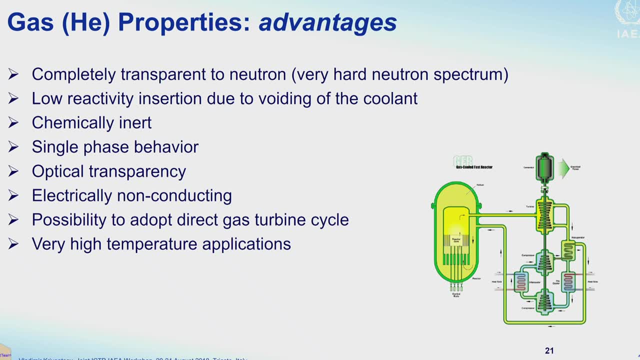 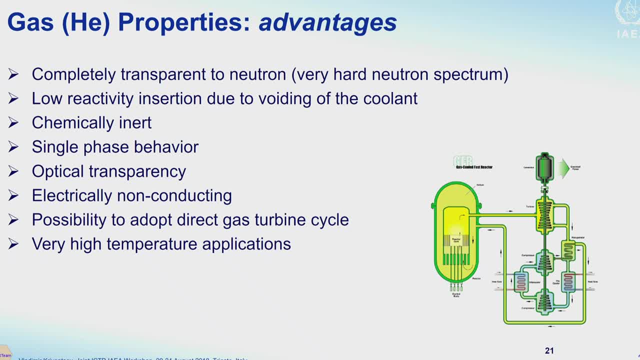 in this case helium. Okay, from neutronics points it's very good and also it has no like reactivity: low reactivity in certain due to avoiding of the coolant, chemically inert and 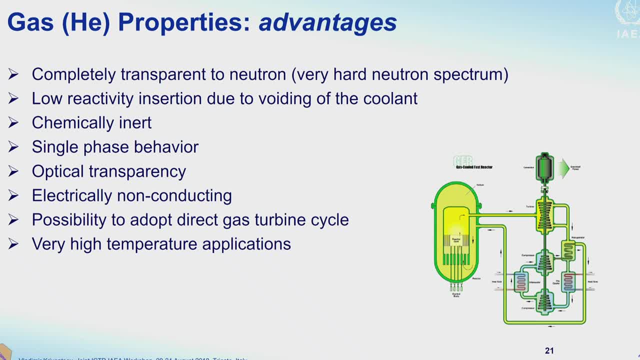 it's single phase. it doesn't doesn't boil because it's already, let's say, evaporated and the boiling temperature is minus 260, something in Celsius if you calculate close to Kelvin. 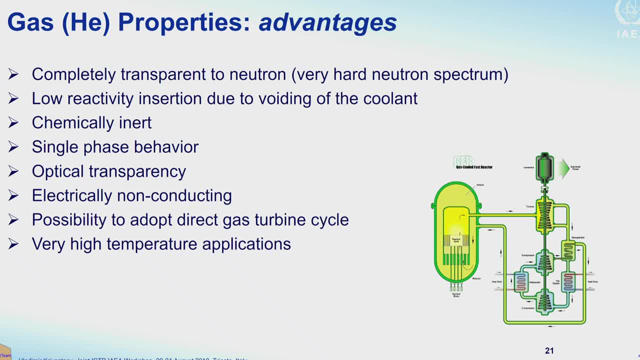 It's very transparent, easy to control, not conducting electric electricity, and you can also adopt direct turbine cycle, so maybe without any intermediate loops, and it's useful for the very high temperature. 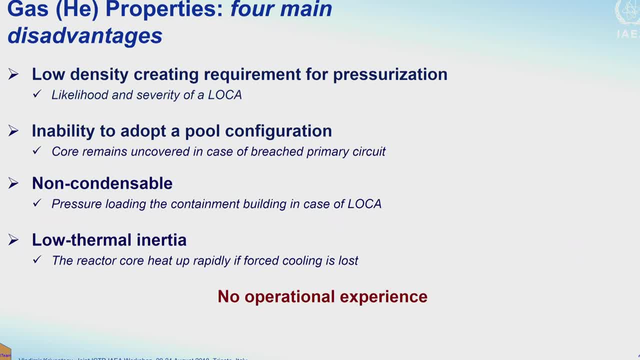 applications. However, there are also, as usual, disadvantages for this. So, since it's low density, you have to to remove the heat, you need to pressurize it and you need to work with very. 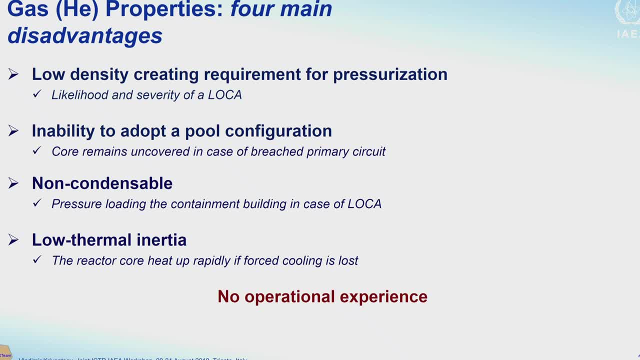 very high pressure and- and this raise the question about this- see, then you have huge potential energy of compression stored in the coolant and, in case of, of of, if you have, I don't know. 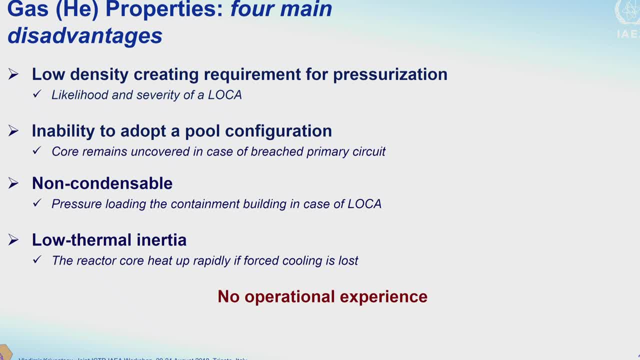 piping breaks or something it's very, becomes more probable and very severe loss of coolant accident, Of course, the depending on the configuration and it's also lower thermal inertia the problem is. 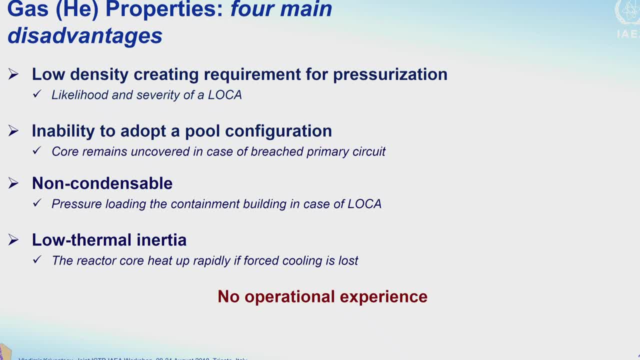 how to remove decay heat, because the density of heat in the normal conditions, let's say if you have high, if you have helium atmospheric pressure, it's very difficult to cool down this system. 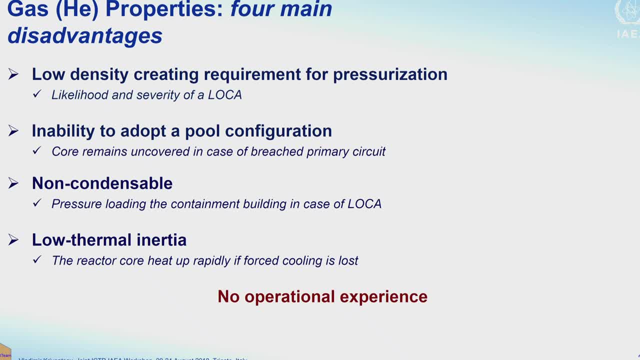 even it can survive higher temperatures, but also this is a big problem and to to be solved. and and let's say conductivity or heat cap- okay, I'll maybe later show- and this is not condensable. 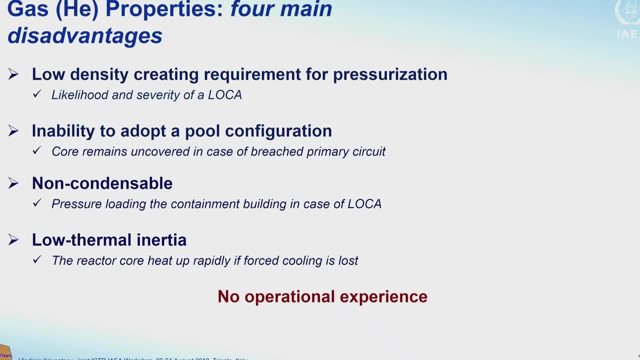 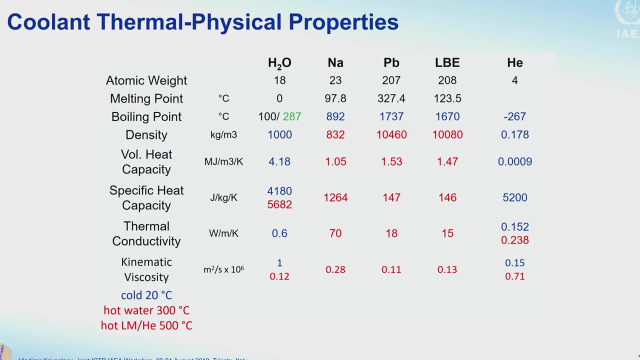 but I will not touch this low thermal inertia I and there is no operational experience at all with this type of reactor. now this table, excuse me. let us compare some basic physical properties. 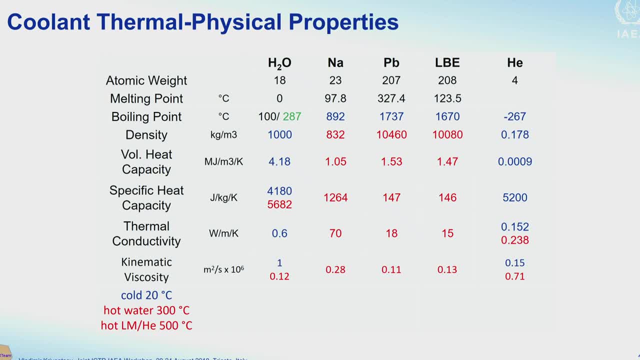 which is, which are essential for thermal hydraulic calculations, for example, and we say here, for example, the boiling point. so for the water you have this range of operation and we compare it with water. 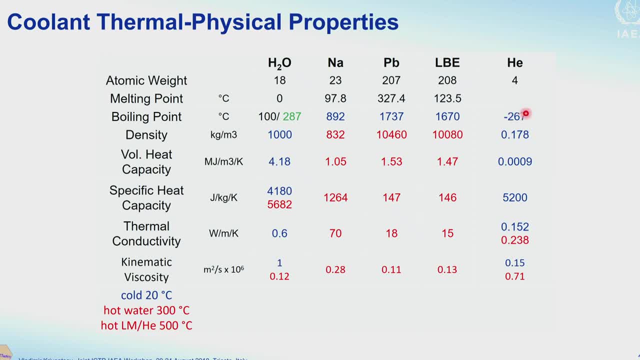 for sodium is much higher. for all of them, helium is already boiled or evaporated, as I say, so it's no problem for the density. so water is, sodium is smaller, the same density a little bit. 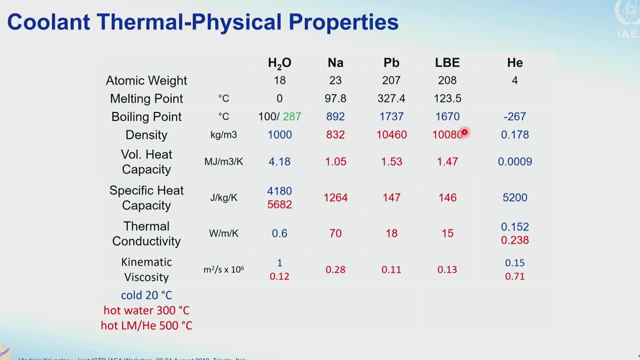 less than water. however, lead- and lead is 10 times of that- has low density, atmospheric conditions, very low density. that's why need pressurization and if you have a look at this specific heat capacity. 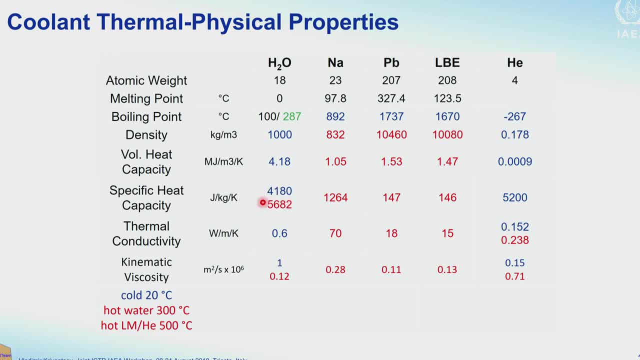 so water is always the best, it's it's per kilogram, and sodium is the second best. and lead and lead. this not lower, lower, but this specific it's per kilogram. but 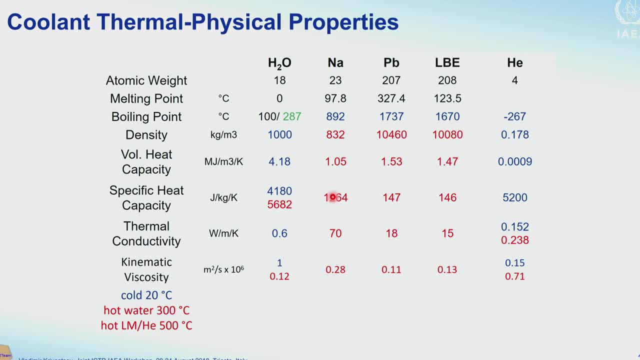 we usually per kilogram, but per volume- how many volume you need to remove- and you look at the volumetric heat capacity per cubic meter, you will see that still water is the best. but 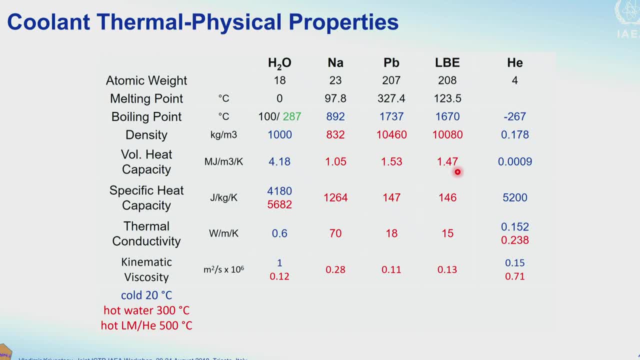 all other three are also very good. it's only, let's say, three times three, four times less than water, which is very good already to remove, but also you should consider that with density. 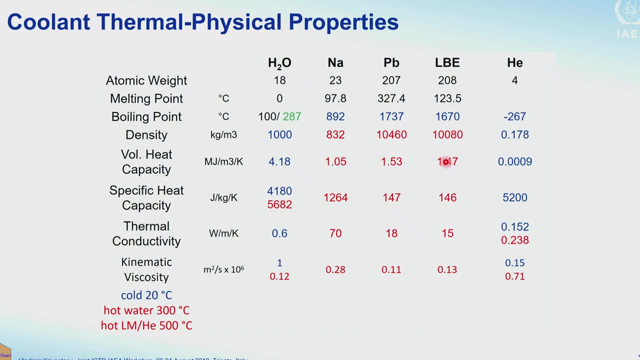 the same volume. it's three times less than volume of. so to remove the same heat you need volumes by time of, with flow rate of course, three times higher than normal water and thermal conductivity. 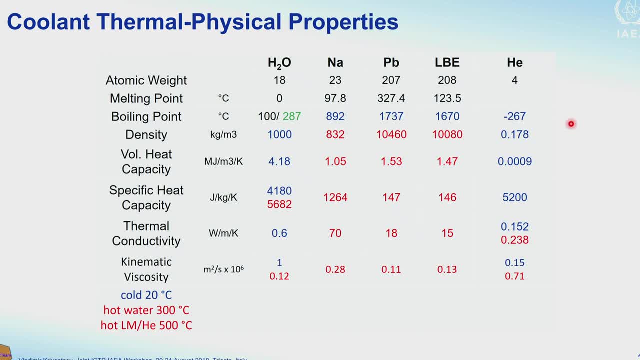 but also if you look in the temperature range. you should. you should understand that with water you can only- okay, we cannot do- enter water with 100 degrees C and release it in 287, it's. 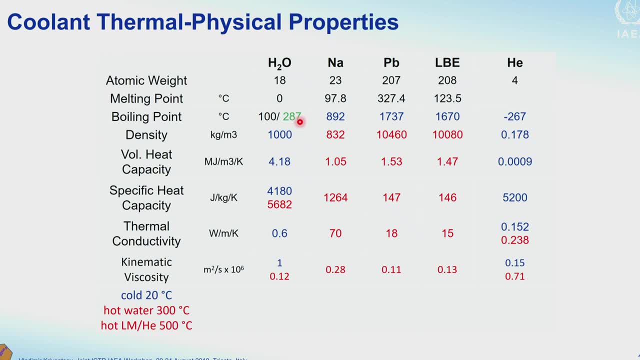 let's say impossible, but we can boil water. it's good, also like heat capacity. I mean it's a good way to remove the energy, but we also want to avoid boiling for this problem. but 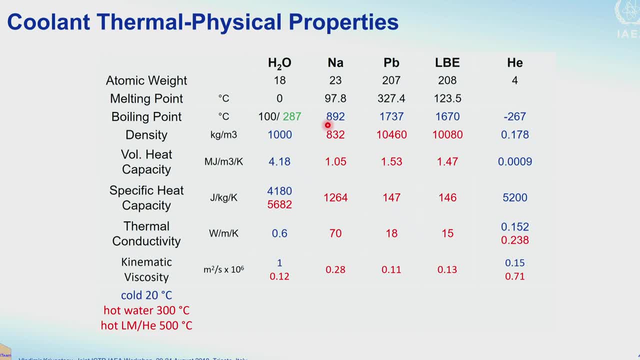 for the liquid metals we can heat up in a much higher range that allow us integrally to remove more heat, potentially more heat than with water. okay, so for the thermal conductivity here. 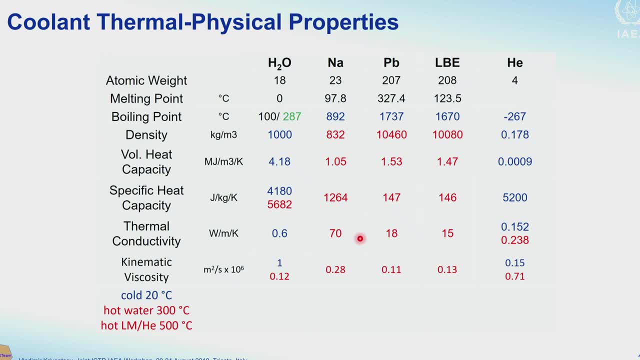 the liquid metals are very good, especially sodium, which is the champion in this case, and we have very low thermal conductivity for helium, which depends also on the pressure it's in the case. 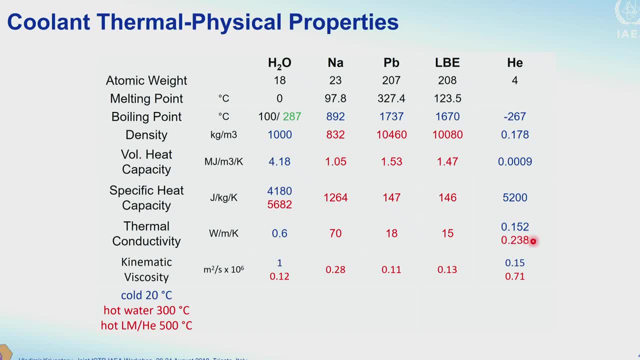 of the low temperatures and high temperatures a little bigger, and kinematic viscosity is very close in all, but it's also important that the lower viscosity less. less energy we spend for the pumping. 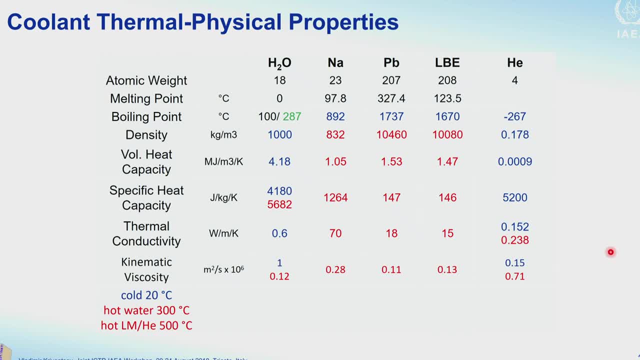 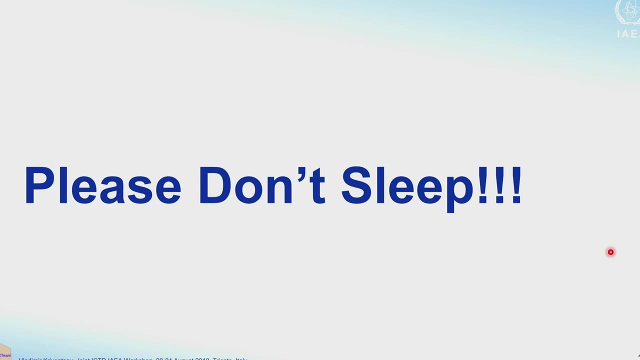 of this coolant through the whole system, for example. so, and this, actually those parameters are basically defined, the way of calculating and how we calculate it and what we can do. 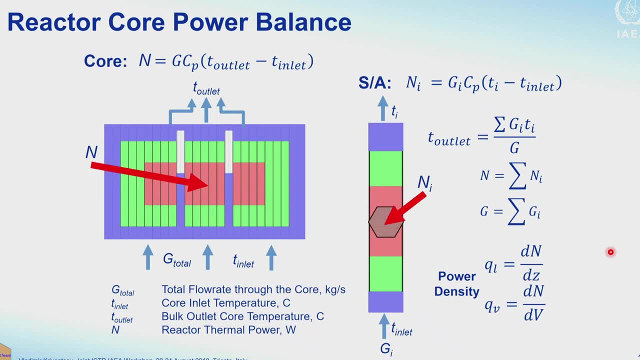 it's not for myself, yeah, not not for you. so now we come directly to the basics of the thermo hydraulic calculations, and in fact it's very simple, especially in steady-state case. 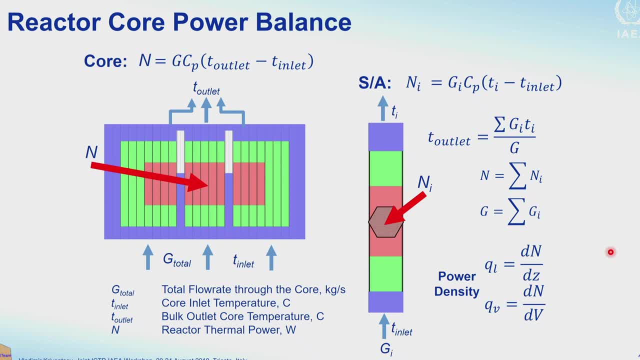 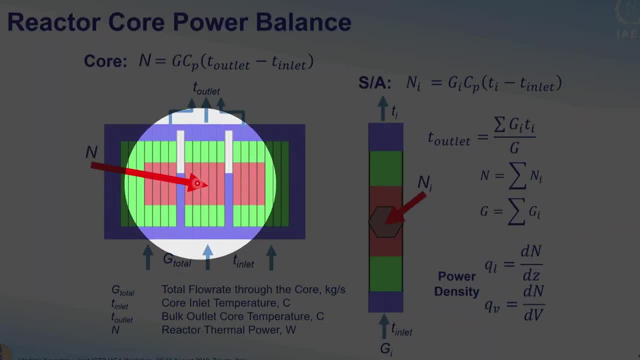 normally you can calculate by hands, as all all reactors were was done for the all reactors. so you have this coolant entering through the inlet into the core with flow rate. 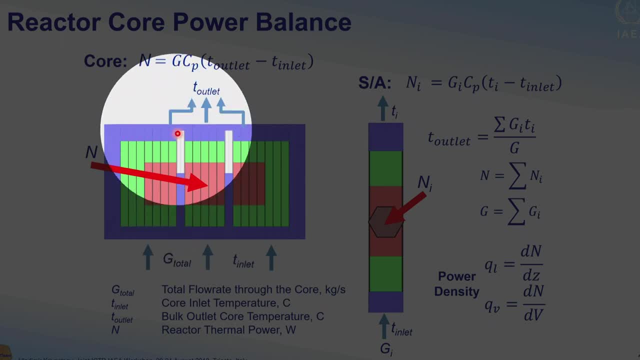 and inlet temperature, where coolant is heated up and it leaves the core with outlet temperature. that's the basic balance for this you can, then the power released is can be really calculated. 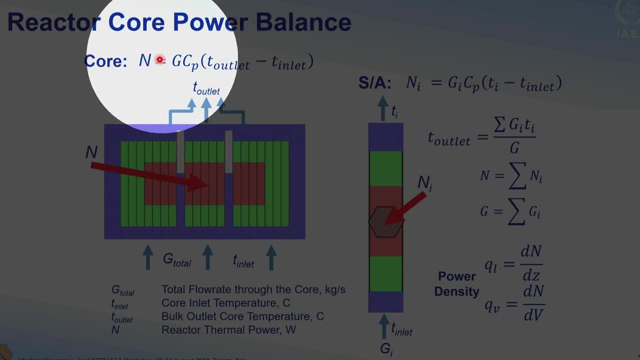 or outlet temperature based on the power can be calculated. flow rate of the coolant through the core. this is heat capacity of the coolant and the temperature difference or heating between the outlet and inlet. 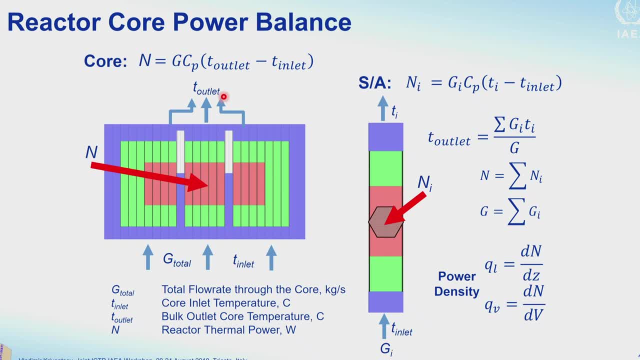 and since in the, especially for the fast reactors, all fuel assemblies are separated in one, in one tube, hexagonal tube, or it's like channel, so the same relation is valid for the. 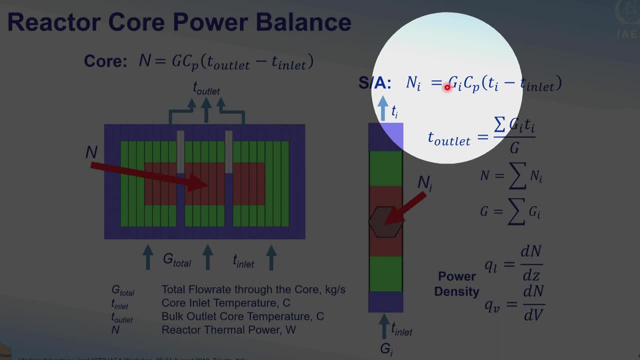 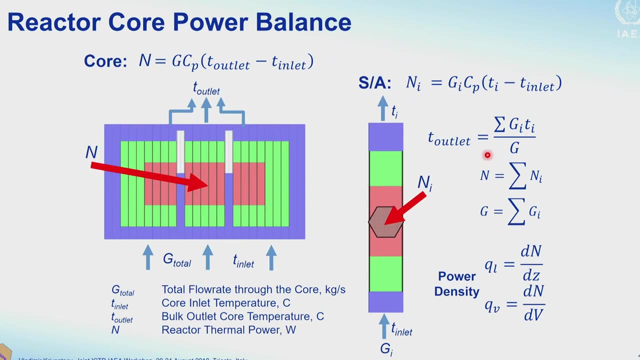 power and inlet outlet temperature and its flow rate and heat capacity. there, with this formula, then we can of course very quickly calculate all. I mean all parameters. so if you know, 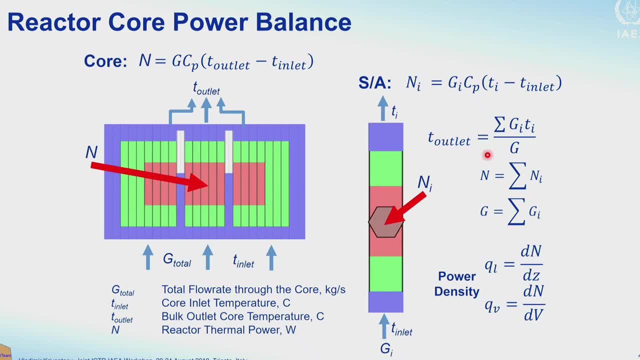 the inlet flow rate. if you know the distribution of the inlet flow rate via sub-assembly, sometimes we have uniform temperature distribution of the outlet, so we can simply calculate with our hands. 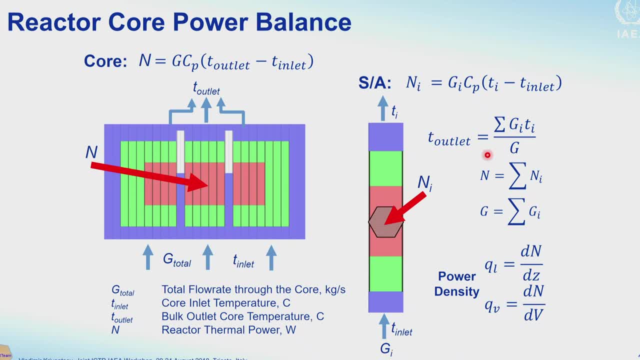 all these parameters, and this case is inlet and outlet temperature, and we can also calculate distribution, of course, because it depends on the height, if you know the power distribution in the sub-assembly. 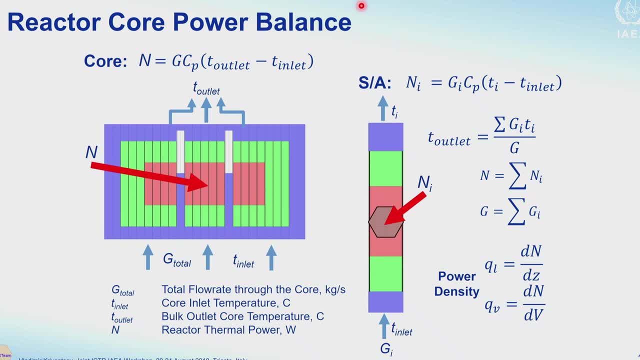 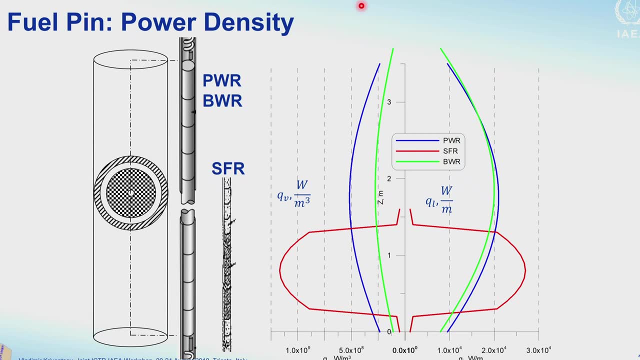 then the here just several key parameters that are considered and you should understand and take into account. so on this slide you see the typical power distribution for different for three types of the reactors. 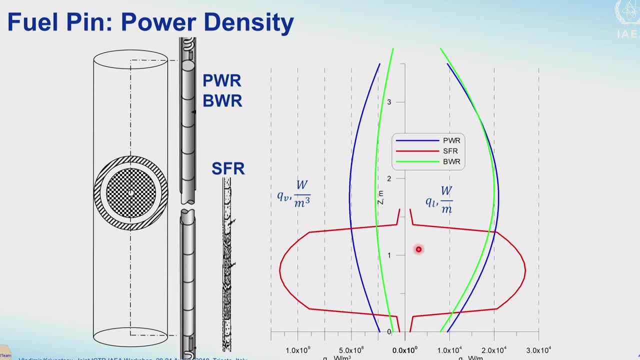 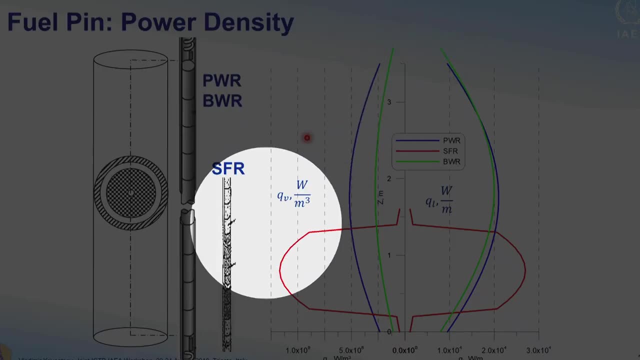 one is PWR pressurized water reactor and sodium cooled fast reactor is red and boiling reactor is green. So as you of course know that the fissile part of the core of the fast reactors and especially sodium fast reactors. it's very much shorter, it's about one. 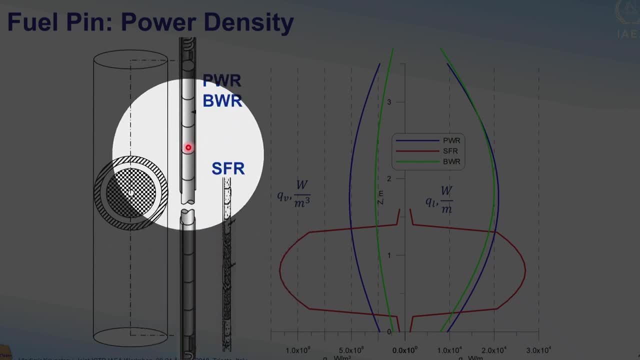 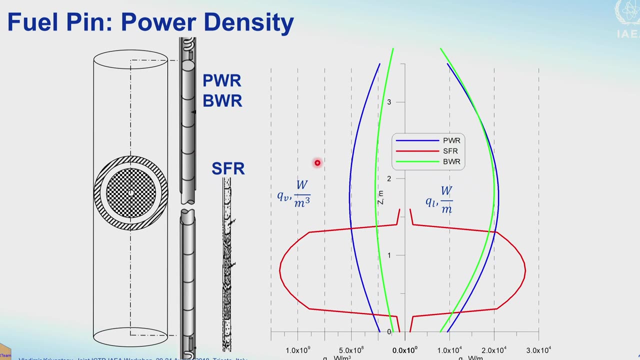 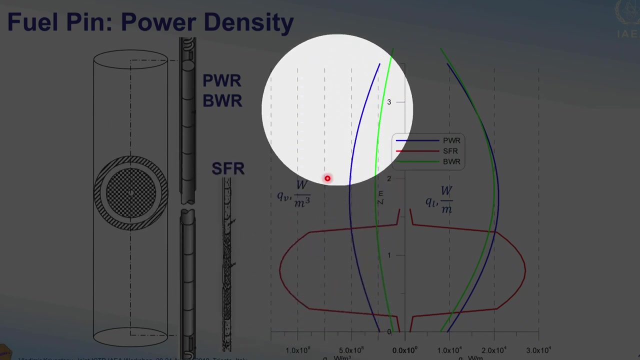 meter only, while for the PWR BW boiling water reactors you can have more than two or three meters core head. That's why we have like this type of distribution. And so on this side you have volumetric, volumetric power density, and here is a. 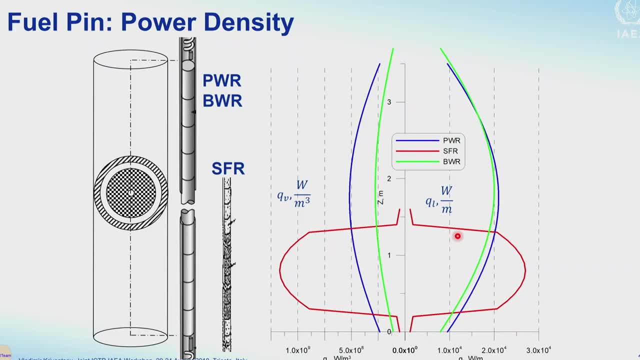 linear power density per meter of the pin. So you see, in this case, field pin of the SFR is much shorter and power density as a result is much higher. to release the same Well, we need to integrally release. so you should know how many pins you. 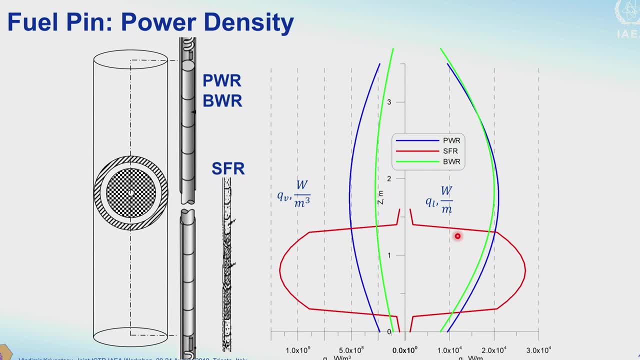 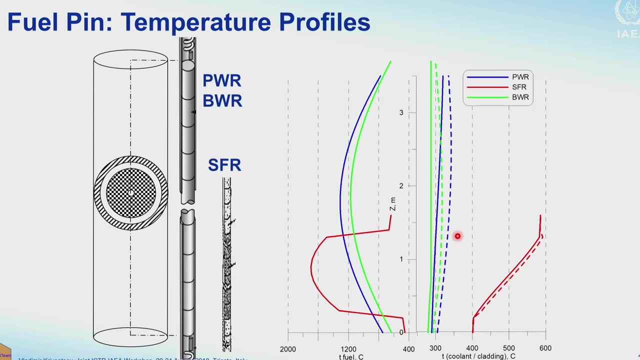 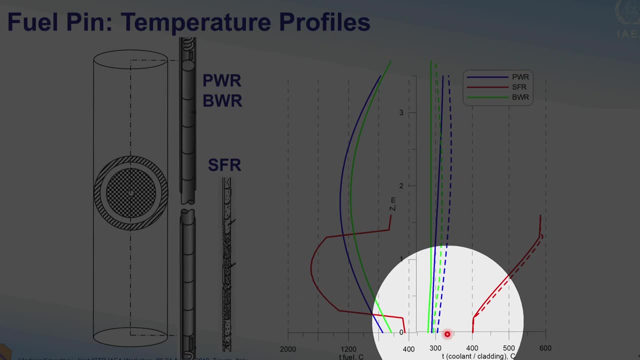 have And pin is also much smaller and smaller. It's half on diameter, so it means quarter of the area and volume of the fuel there. So as a result you have the temperature profiles like that You see in water reactor. the heating is very in both. even in boiling it heat ups and then goes constant. of course It's very. 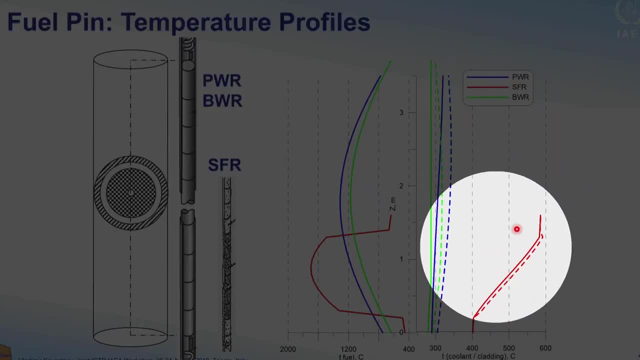 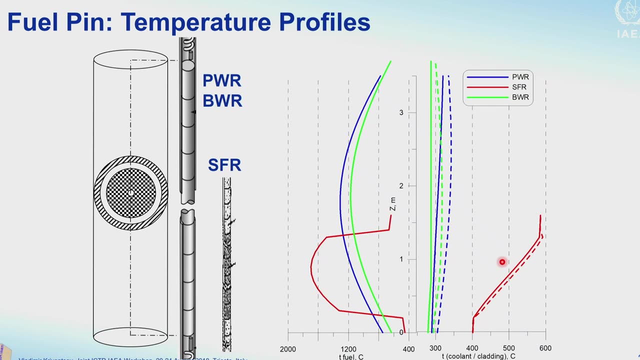 small heating, while in sodium cooled fast reactor you have pretty huge. okay, it's 200 feet approximately. now it's usually it's a little bit lower, like one hundred and fifty, But this feature also to have higher power. density is much and also fuel temperature. 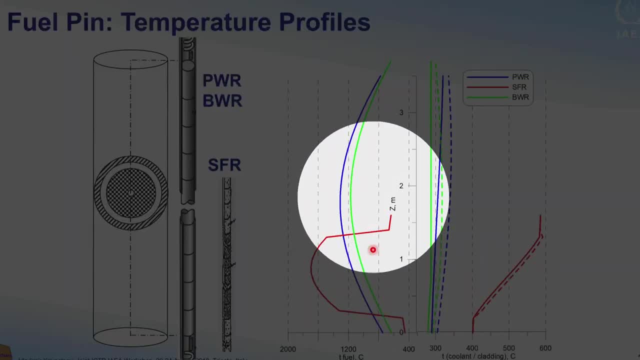 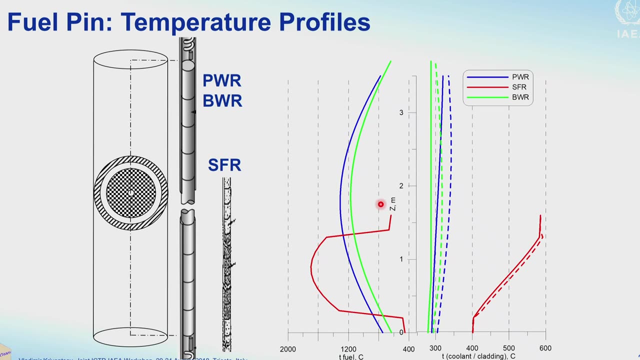 is the same, remains, okay, nearly the same maximum fuel temperature, And that is a big benefit of the sodium cooled fast reactor. Actually, we can with this temperature difference. it's not only to increase the efficiency, because higher temperature means that we can. 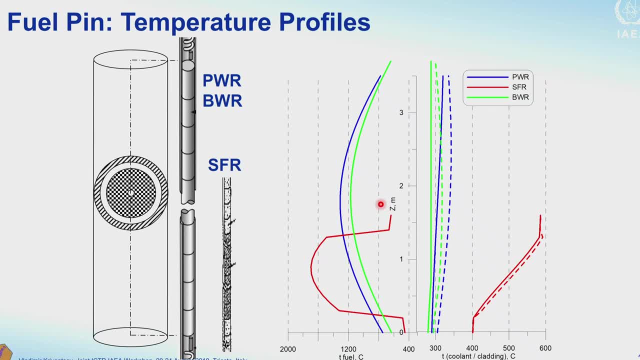 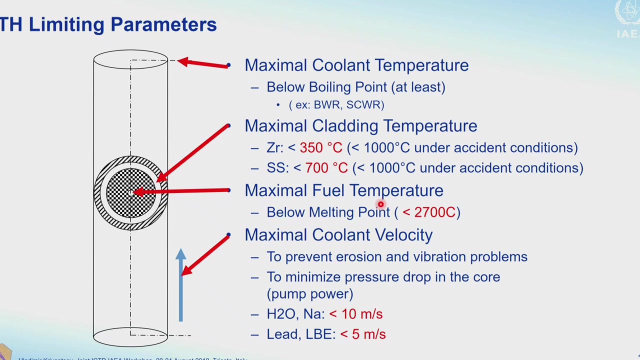 have a lower power density. It's not only to increase the efficiency, because higher temperature means that we can have a higher power density. It's not only to increase the means- higher efficiency to produce electricity- but also that with lower amount of sodium, we can remove more energy from the core because we have high temperature range. and then okay. 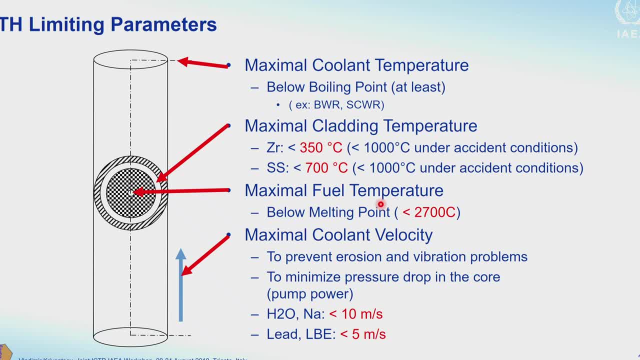 normally we require it from you if the designers decided to such type of reactor, a new type of the coolant or something, not from you, from some hydraulic calculations, it's to make sure that you calculate the maximum possible temperatures within the system and make 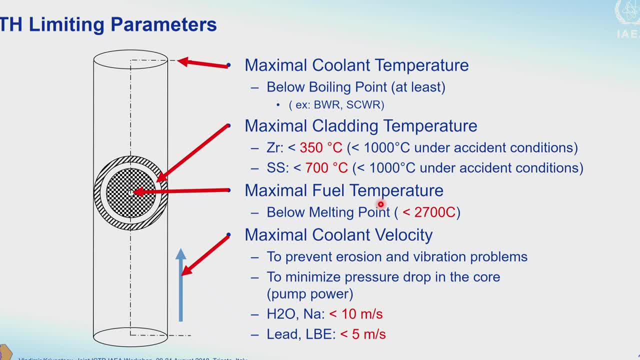 sure that maximum coolant temperature should be at least below boiling point, or also some limited parameters, For example. sorry, maximum coolant temperature should not exceed boiling point, for example, or some other could be. So maximum cladding temperature is also limited, For example. 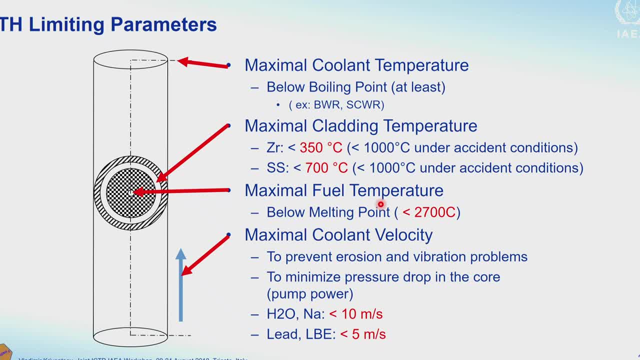 for zirconium, which is used in the water reactors, it should be like less than 350 degrees C, and for stainless steel it should be less than 70 degrees C, and usually we require less, even to have a margin and the and in case of transient calculation. in any case, this temperature should not exceed 1000 degrees C. 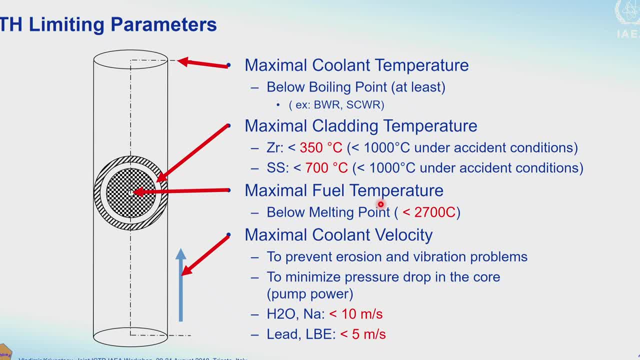 otherwise you will have a cladding will fail and you will severe accident conditions. So maximum fuel temperatures you calculate should not exceed melting point. That is the main and the only parameter. but you should also leave the margin for this. Coolant velocity should not exceed some. 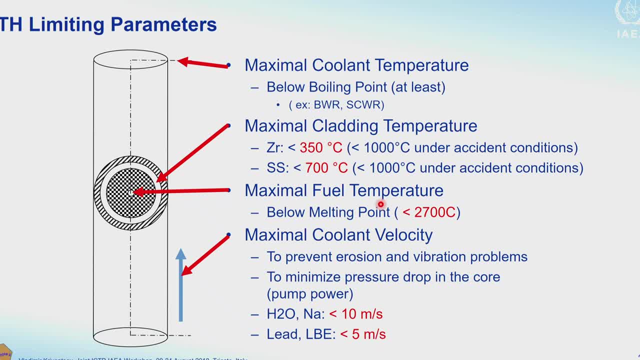 maximum and its maximum, which is used to prevent erosion and vibration problem, and also, you should think, to minimize- refused to minimize- pressure drops in the system which is dependent on the square, from the velocity of course. so for water and sodium the limit is said meters, but it's a maximum limit of 10 meters per second and for the heavy, 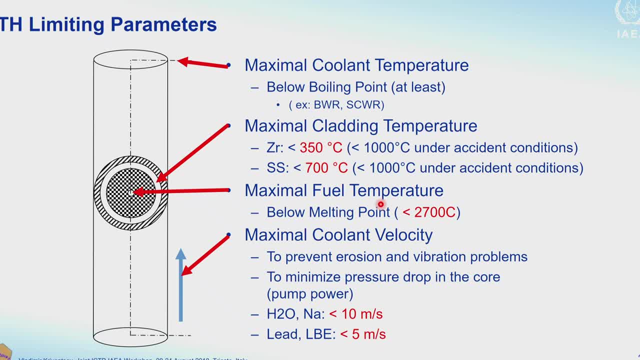 metal it should be. the velocity should be less than 5 meters per second, However, normally was even higher for sodium. for sodium we could have five or seven- actually limited parameter, and for lead it's two or three meters per second maximum to avoid this erosion. so you 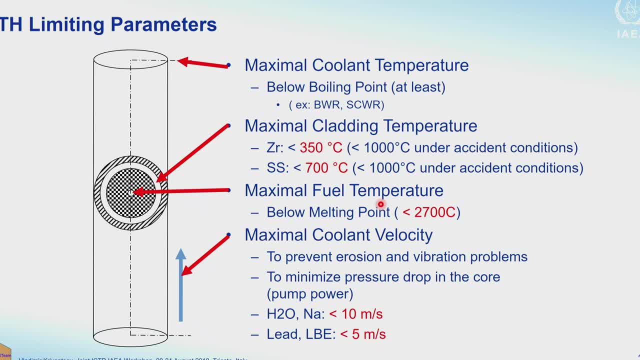 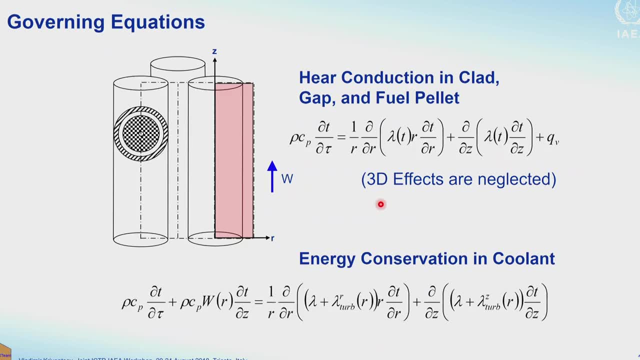 should control and you can play with parameters. of course, higher flow rate, you can remove more heat and then, but- but you should look at this in the balance and how we calculate all this. it's also governed by a relatively simple equation of energy conservation in this case, and he is energy. 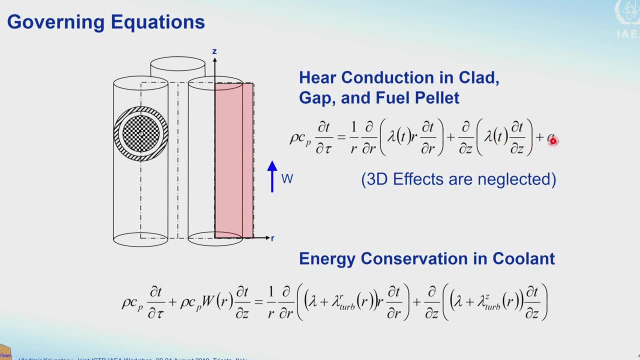 conservation for the or heat conduction operation, in this case for gliding gap and fuel pellet, and for the you calculations. we would neglect this transient term. usually we also neglect this because of the lens and the distribution. we couldn't also neglect, neglect this X Excel distribution also, then to calculate the temperature. we. 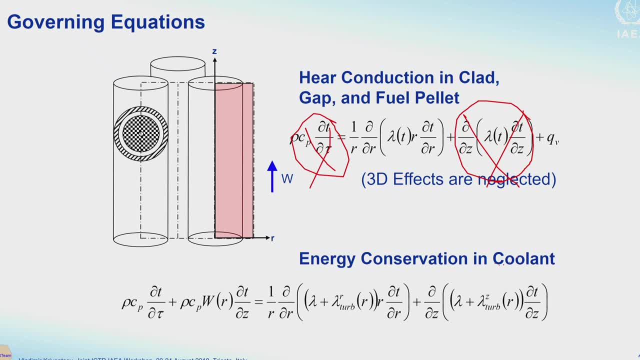 need only solve- even it can be analytically solve- simple equations in coolant. we have a little bit more complicated equation. also here we can neglect the transient term, energy conservation for the coolant and we usually. we also can neglect this Excel distribution because it's much lower terms, and the radial 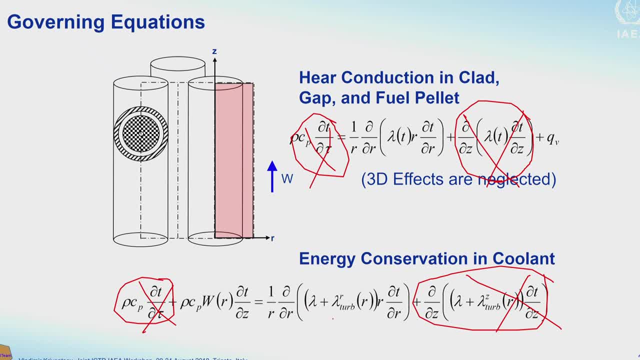 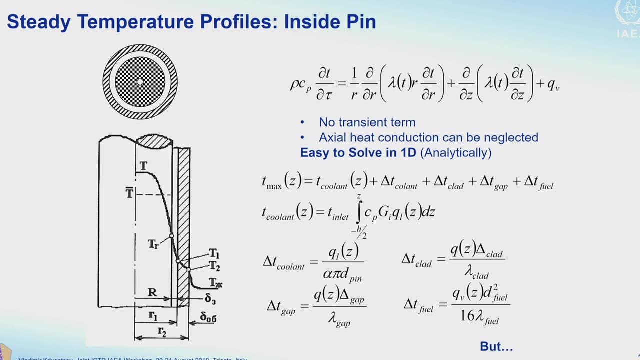 distribution. but we should solve this equation, which is cannot be solved analytically. but we have simplified matters like using heat transfer coefficients, like I will show you again. for example, if it's from this very simple calculations, coolant temperature: here, to get the temperature of the wall you need heat. 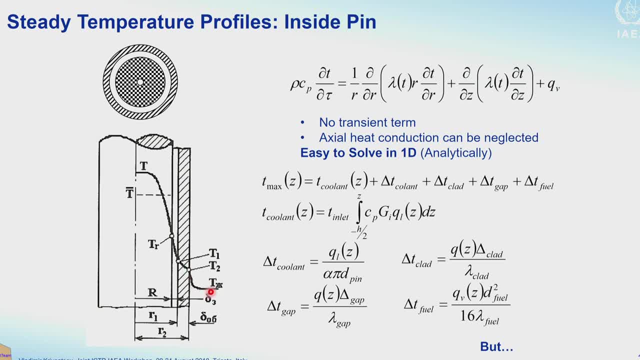 transfer coefficient- we don't need to solve this completely- the energy location and again, in simplified one-dimensional effect case. then we can simply calculate the temperature difference between inner and outer wall of the gap here. Then you should calculate temperature drop in the gap between fuel and cladding. 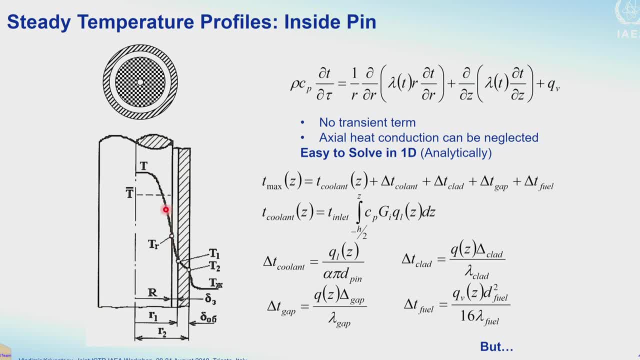 And then it's parabolic distribution of the temperature inside the fuel period. So all can be easily. it's analytically also calculated. if you know heat transfer coefficient, Where is the heat transfer coefficient here? Okay, this is alpha also for heat transfer coefficient. 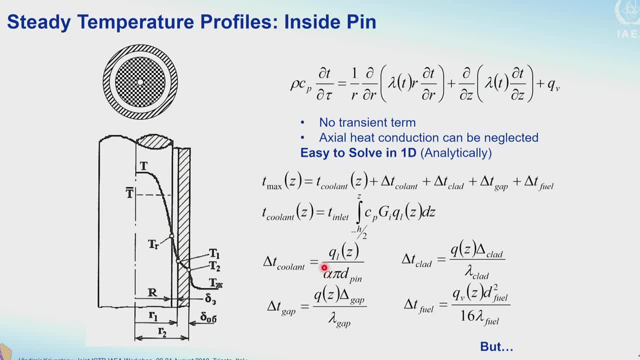 In Russia we use Greek letter alpha, Normally in English it's H also. So if you know heat transfer coefficient, okay, you can create immediately temperature on the wall. Then if you know parameters of cladding, you can calculate temperature difference on cladding, and so on. 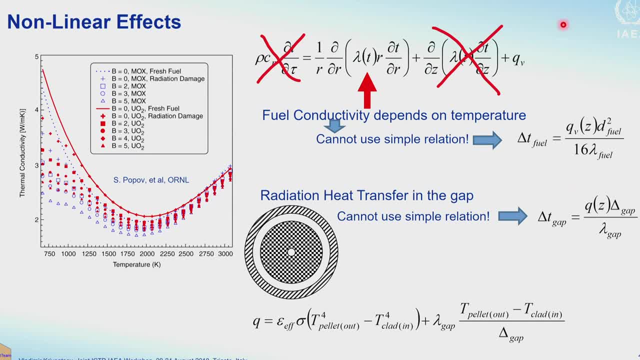 And this looks very simple, but there is complications Because, first of all, the heat conductivity of fuel, for example, depends on the temperature. So it makes this problem nonlinear And you can- You can not use this simple relations as I was showing on you. 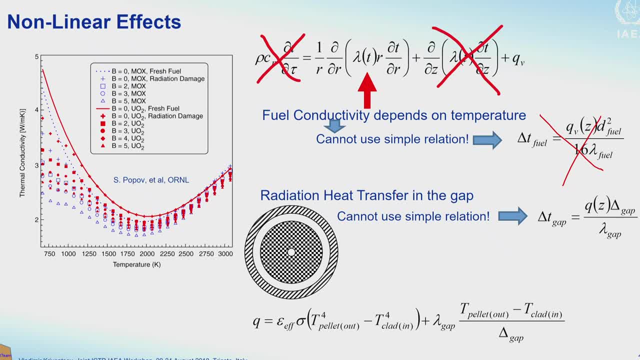 Not valid in this case because of nonlinear character And also in the gap you have irradiation heat transfer between the walls of the gap. That means you also cannot use the simplified formula here, but you should solve nonlinear, nonlinear equation of the irradiation heat transfer. 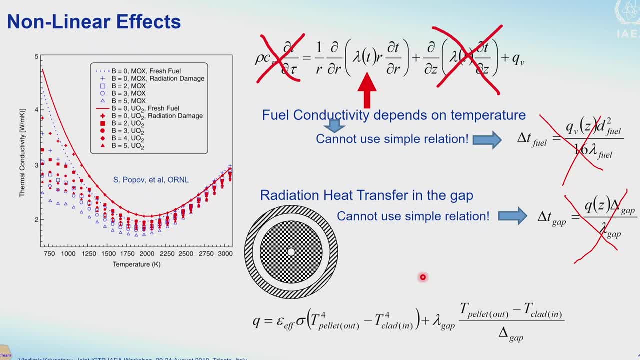 plus delta 10 gap to get this, Which is also possible of course, by, let's say, you can use iterative process to solve here this. But here to solve this you have to integrate this, because conductivity depends on temperature. You cannot solve. 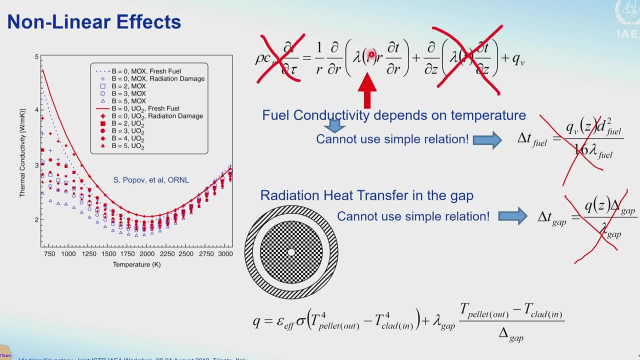 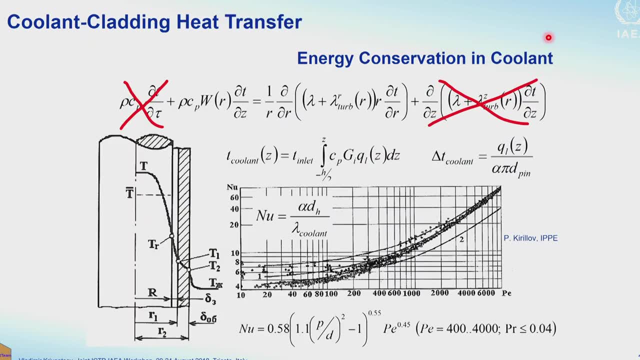 And the dependence is nonlinear. If you had linear, you could solve analytically, but in this case, no. That's why even this simple calculation can be made by hands, with some assumptions and so on. We need some numerical, Okay, and then, as I saw, you don't need to solve. for example, 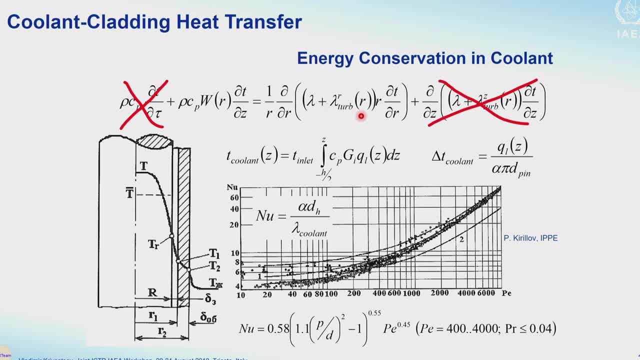 for the simple case as energy conservation equation in the coolant, It's enough to use heat transfer coefficient, and Lucid number would be applied, and with good Curiously, let's say using this Lucid number for different. There's a huge range of materials you can get. 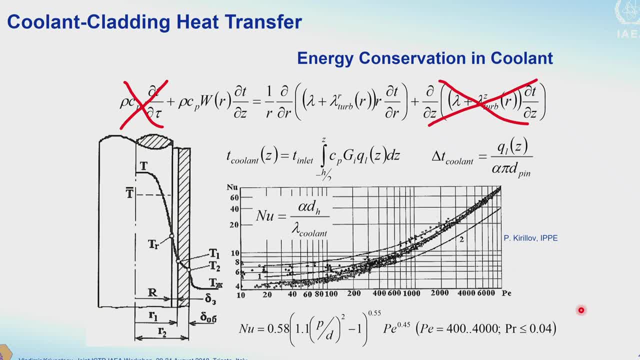 The temperature difference between coolant and cladding wall. Also, since, for example, the sodium conductivity is very high. this difference like 10 or 15, 5 degrees C, so it's not as Even if you make a bigger error, it doesn't affect at all. 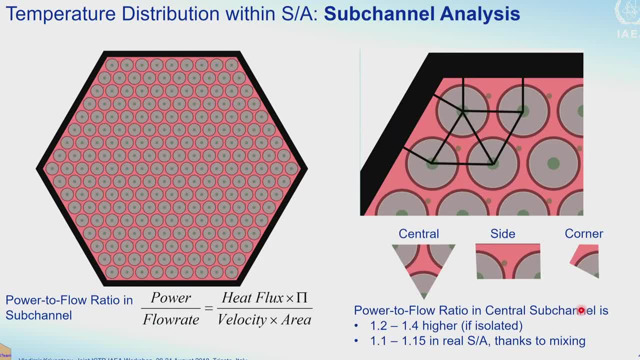 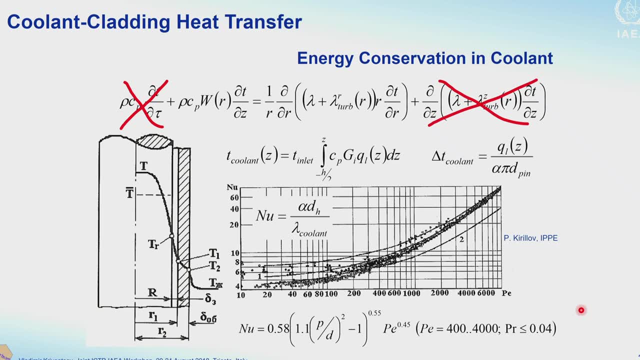 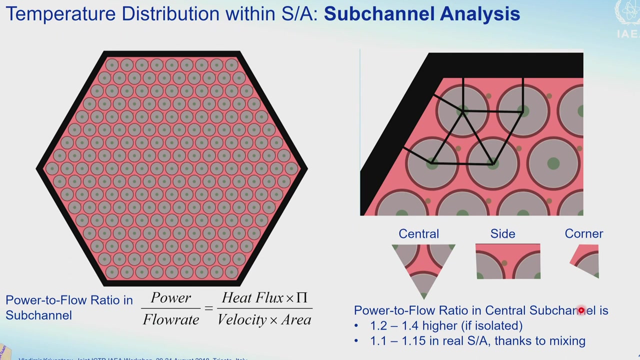 Many doesn't affect significantly. This is Okay. but to solve more accurate, more precise all these things, normally this equation cannot be solved analytically, and then we have to use the numerical methods to simulate this. Okay, this is for an ideal pin. 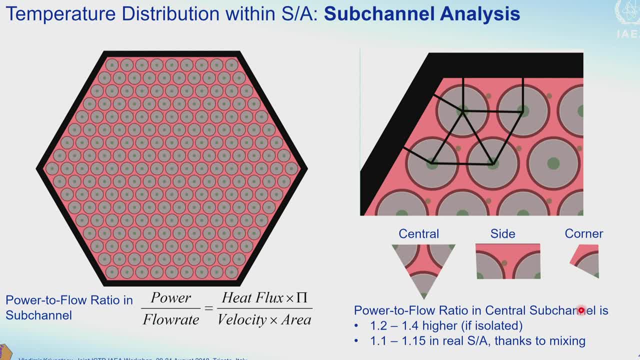 in this ideal hexagonal array of pins. But in practice we have kind of those pins are collected in the hexagonal tube and it makes this task of finding power and maximum and lower temperature distribution a little bit more complicated. because if you look at the peripheral area, 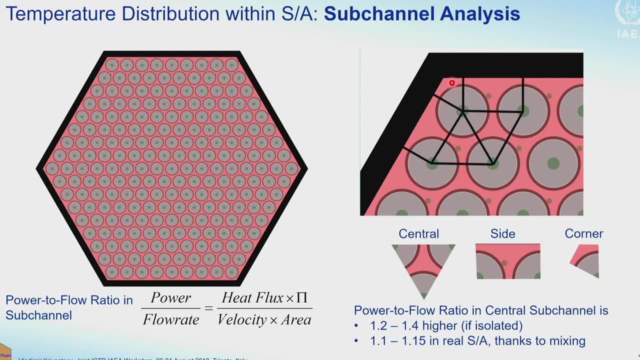 you have so-called smaller channel. for instance, depending on the parameters of the gaps here, you can see that this is gap is very small and it receives the corner gap, but it receives 1 sixth of all power Here. this is relatively bigger flow area. 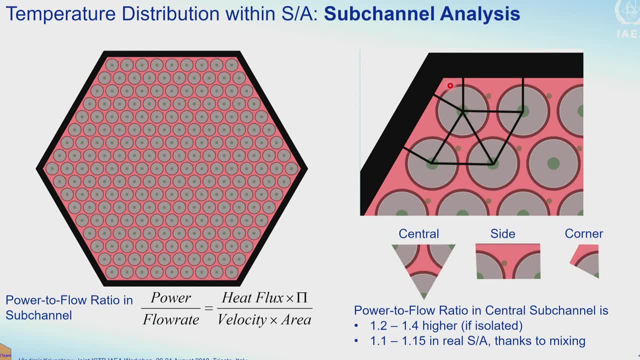 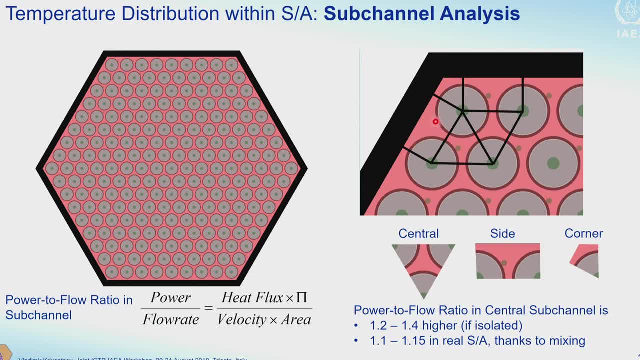 And vice versa. for example, this area of the side sub-channel is much higher, even if it receives more energy. So during this balance, we can see that power. I mean this. So what we need. what defines the heating in such a system? 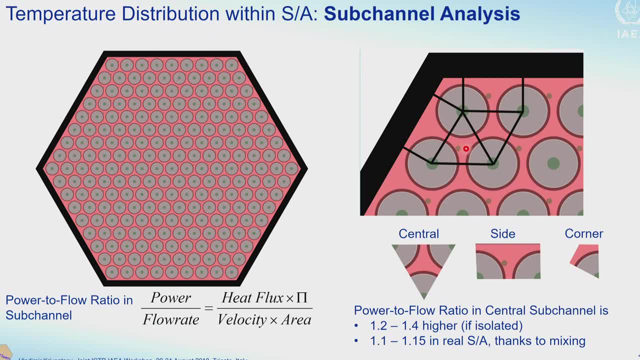 it's how much power you give, it's how much power you give, it's how much power you give and how much flow area you have, or flow you have, and flow defined by flow area as well. So in case of the relation between ratio power to flow, 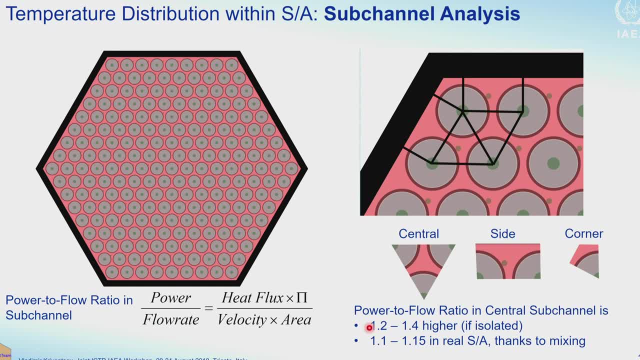 So in case of the relation between ratio power to flow, in the central sub-channel it could be 1.2, 1.4 times higher than in peripheral channel, but also thanks to the mixing, because you have a mixing conveyor, it couldn't be lower. 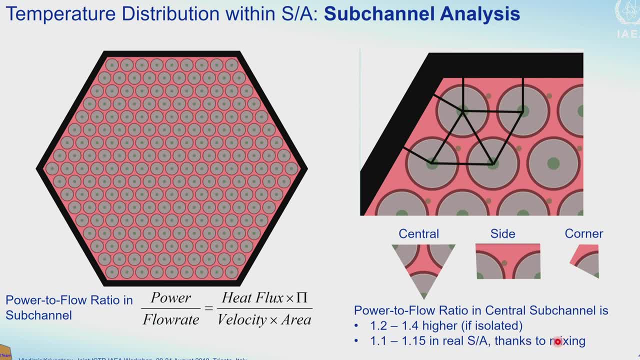 But still the heating in a central sub-channel. But still the heating in a central sub-channel, But still the heating in a central sub-channel. the central sub-channels of the sub-assembly is 10 to 15% higher than heating in the peripheral sub-assembly. 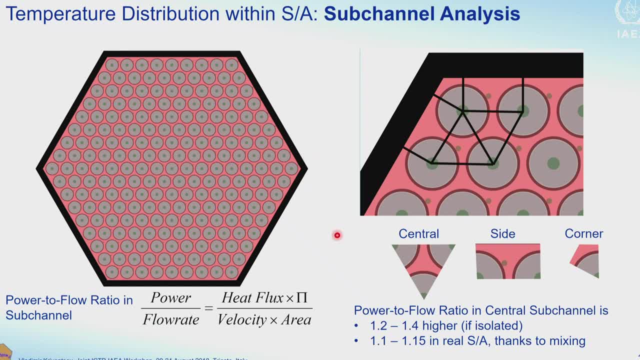 Then you should take it into account because it will have change a little bit: temperatures And in the sense of power to flow rate. it's like heat flux by perimeter of the heating area divided by velocity and area of which is defined by flow rate. 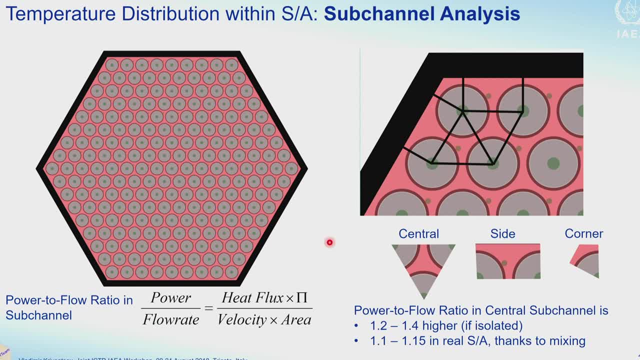 Also it could have less or even higher velocity. Also it could have less or even higher velocity. Also it could have less or even higher velocity here, since, because it's more open channel, it can have high velocity in the side channel. 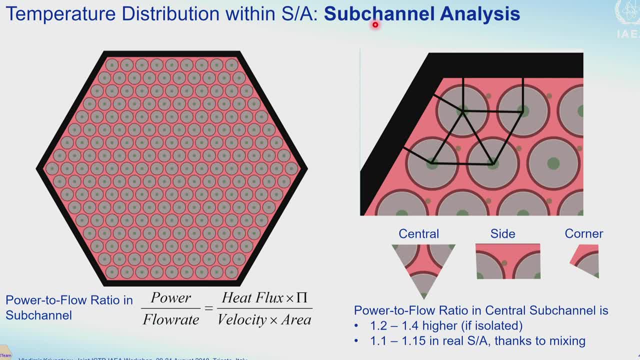 And all these things. for example, the previous task, what I show you non-linear- could be solved by CFD method. Now CFD can be also applied to this whole sub-assembly even, but it will require a huge amount of the CPU power. 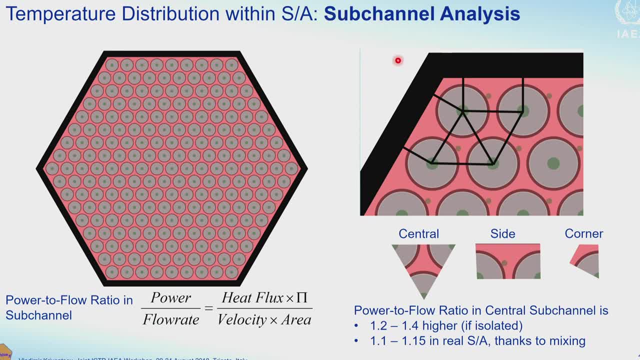 And traditionally long ago we used so-called sub-channel analysis, When all those sub-channels are divided and like different, let's say, volumes, with some exchange of mass and heat between these volumes, and solved with sub-channel analysis. 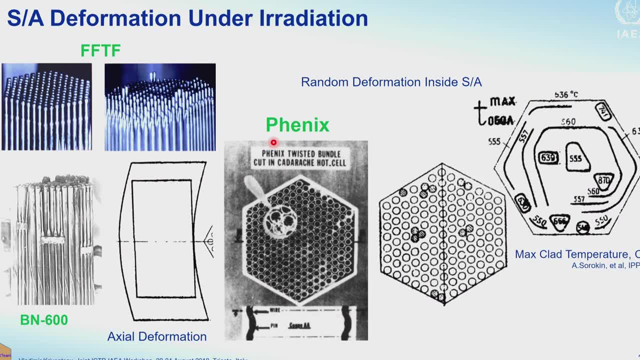 which is simplified but very fast method to solve these problems. Another complication which I'd like to show you is this is the these road bundles of fuel assemblies are not perfect. They are perfect when you design it and you present maybe in the museum or even in. 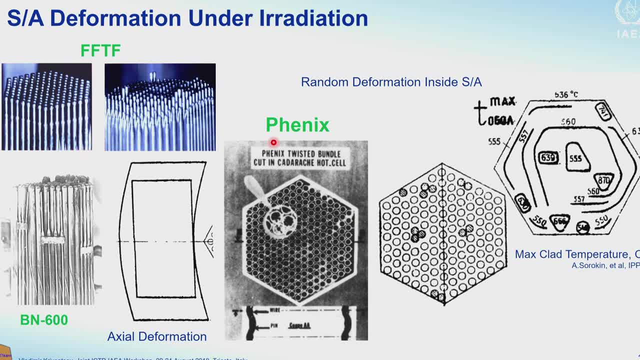 and sort it to the core, But then it is a huge burn-up and huge irradiation in fast reactors, particularly fast reactors. What we have, for example, I sold already, but look again, This is fast flux test facility in there. 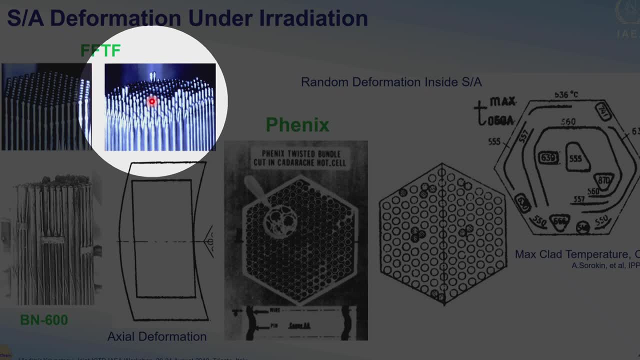 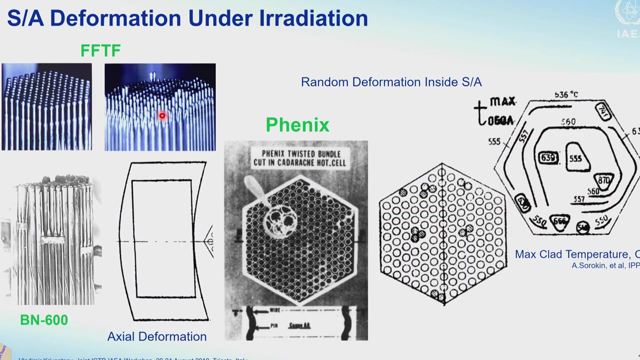 This is before and after they remove it from the active core. You see obviously some pins, for whatever reasons under radiation, elongated much higher than others. What is the explanation? There are many million explanations which we should ask some people from structural material. 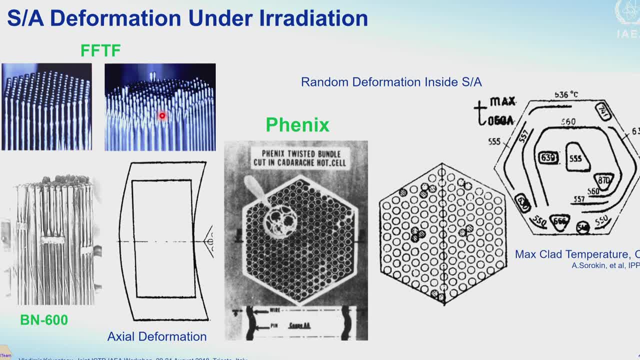 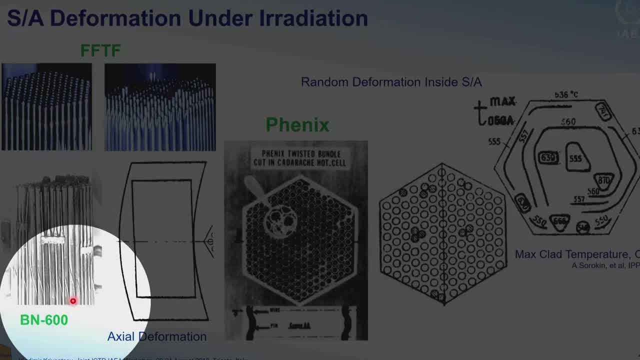 and they provide sometimes different, but it's known effect. It could happen. maybe you know fabrication or whatever. The same for the Benz 600, the same picture of the opened already fuel assembly after irradiation. You see some pins somehow elongated. 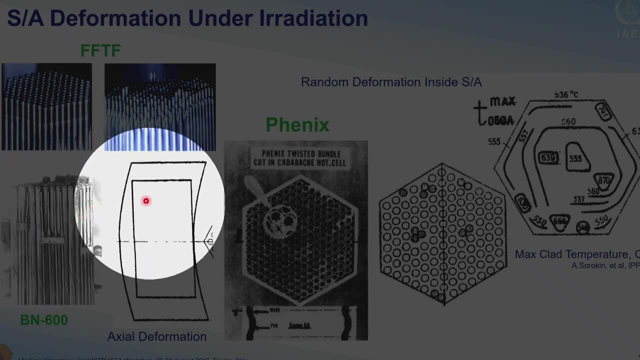 much higher than others. Another effect: then you have this deformation of the hex can tube, because it's small wall something, So it's also dependent on the temperature. It deform it like this, Then you have higher flow rate in this area. 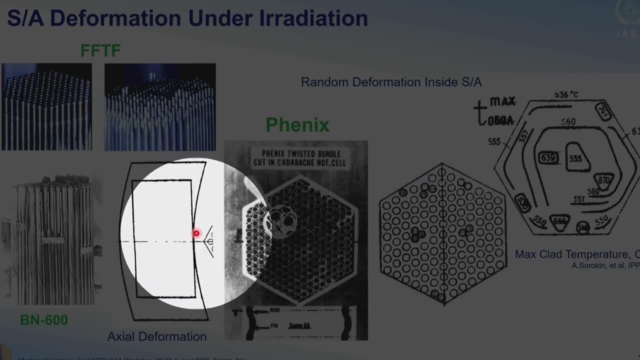 and less heating and colder And you could have huge flow rate. I mean lower flow rate and then huge heating also and overheating in this area. when the can can touch And you see that Wire does not, for example, you don't have wire here. 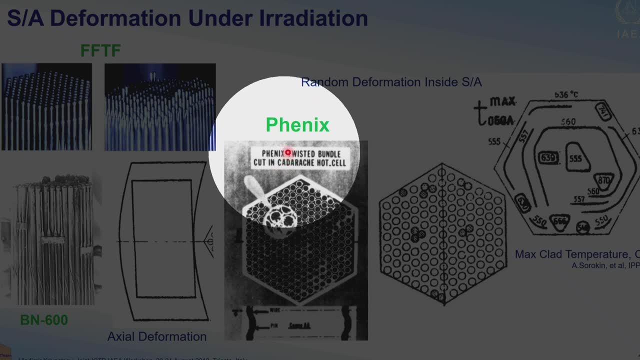 then it can touch directly the wall and something. This is also famous photo from the Phoenix reactor, which, the only one that was disclosed by our French colleagues to the public after the many years of investigation. You see, if you look at this photograph, 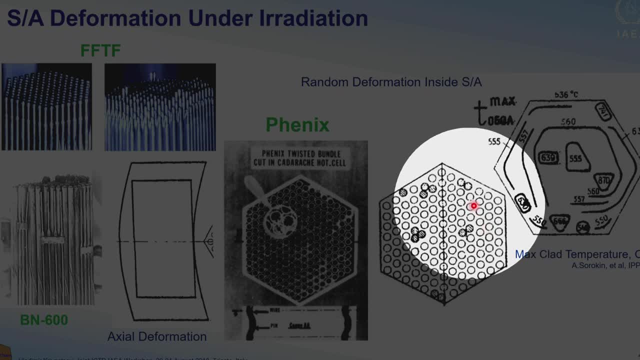 you see that strange. some pins are in a okay, or I mean still, It's still in triangular, but some pins attach each other here, here, here And most zeros, even there the three touch in one. 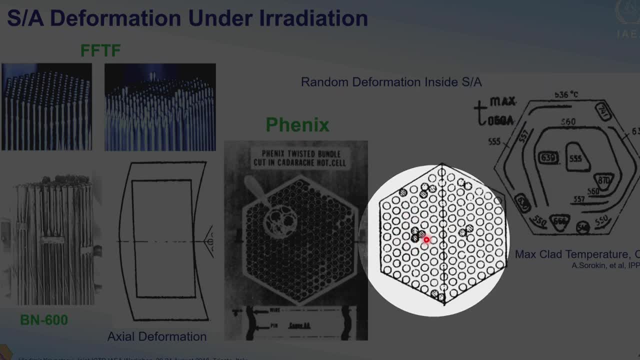 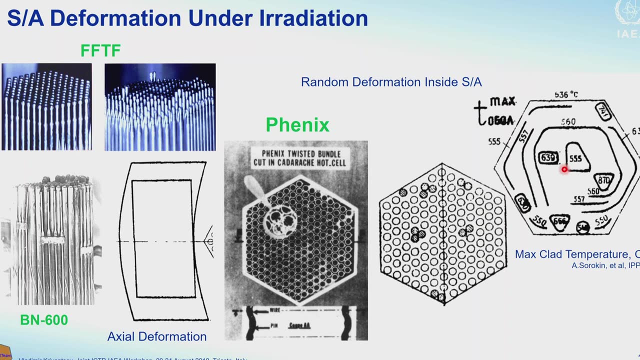 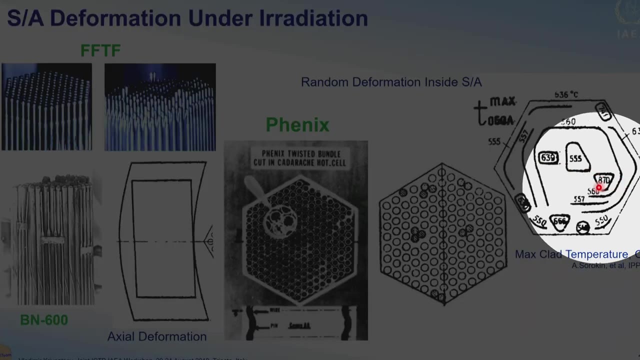 That would definitely result in the overheating and something That also was calculated. If you calculate this sub-channel analysis method, it was done long ago. I believe Krista knows. So the maximum cladding temperature can reach here 870 degrees C, which is much higher than VXC. 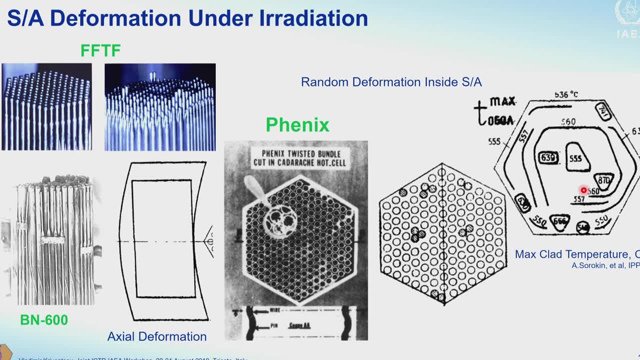 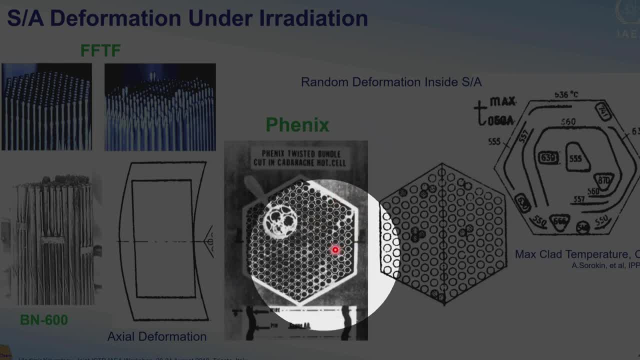 Of course it might be. this configuration was taken, not in the reactor- working reactor, of course- but after the fuel assembly was removed, stayed somewhere. Maybe it was a result of the experimental, because it was cut like this and they were filled with bitum first also. 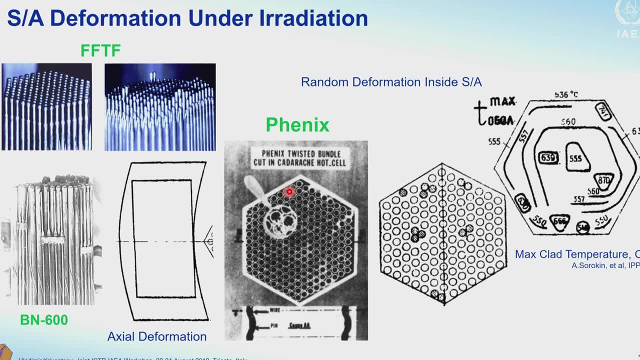 But still we understand that such things are possible because of the pins and deformation. VIA cannot prevent this kind of deformation And thus effects should be also taken into account. And let's say, to simulate such system you cannot use simple method as described before. 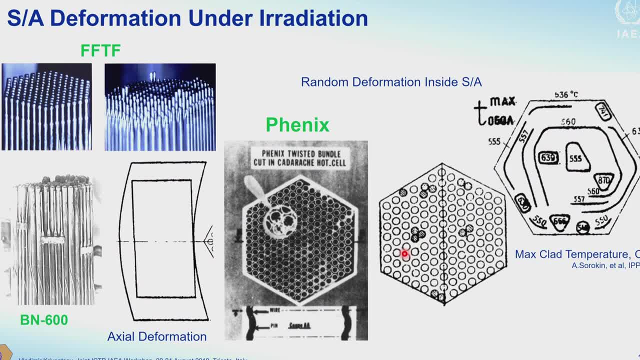 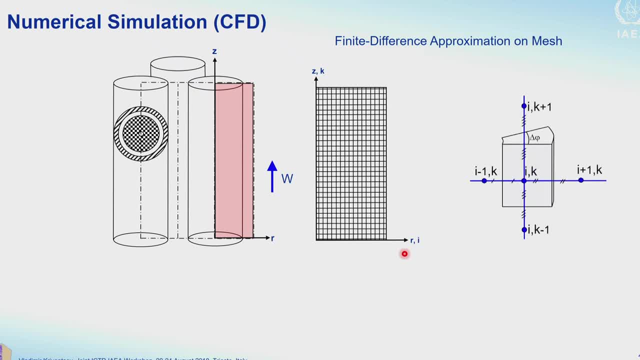 You need at least sub-channel analysis and maybe also CFD, even if you know the geometry. So that's why we usually use numerical simulation instead of head, And calculations are with pen, But hand calculations are also very useful because you understand the physics. 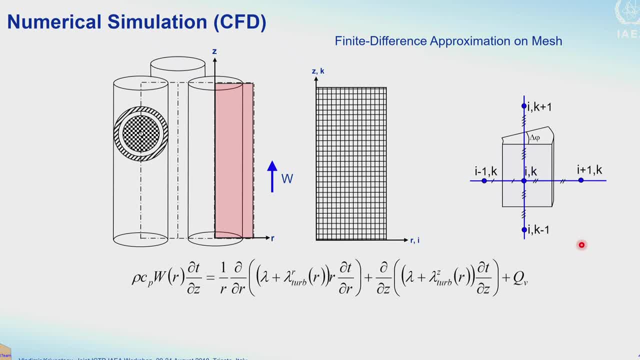 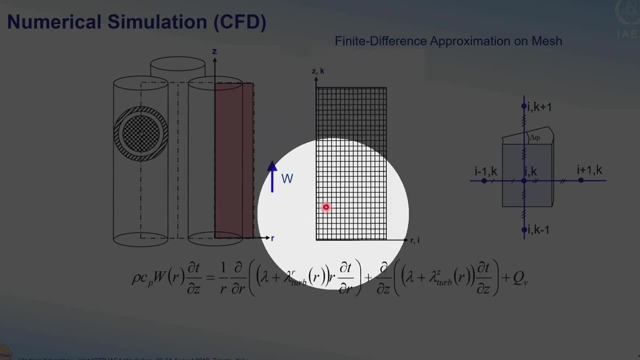 you understand how, what is the influence of the parameters on each other, and so on, And this, let's say using CFD, we define the calculation area is covered by the mesh Somehow. in this case it's two-dimensional RZ. 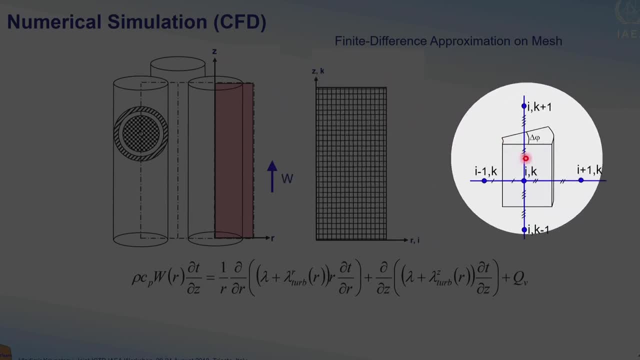 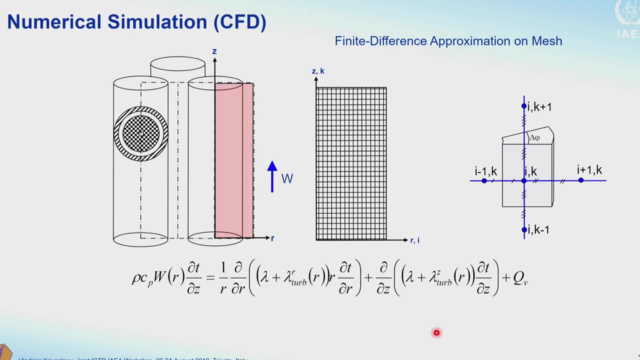 Mesh And the one mesh element represents like this: And to solve this. so you cannot solve this analytically, but you can solve this instead of this, oops, sorry, Instead of this equation, we can solve the system of after discretization. 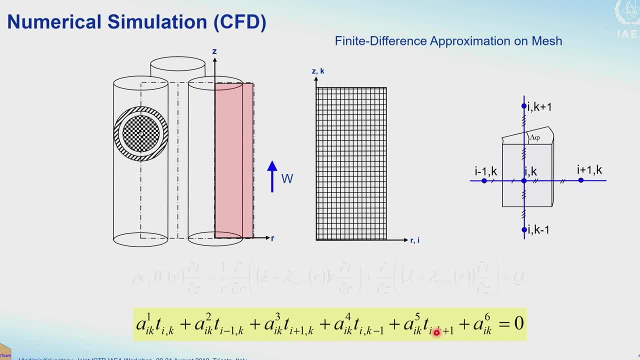 which have different, different methods I don't want to touch. We finally have the system. We have a linear equation for every node and all together for every mesh it becomes a system of linear equations. then can be solved by computers. 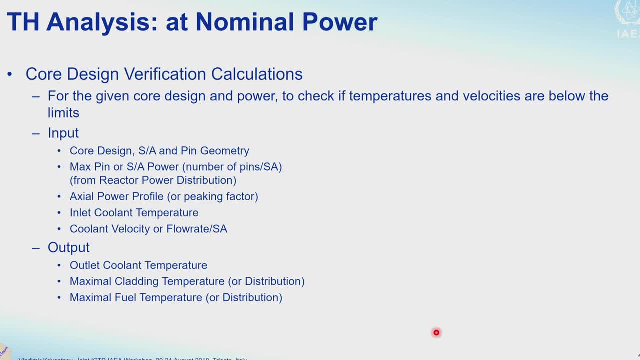 with different methods and so on. So now, what is the tasks or goals of the thermohydraulic analysis at the nominal power and steady state? So there are two types. So there are two types of basic types of the simulations. 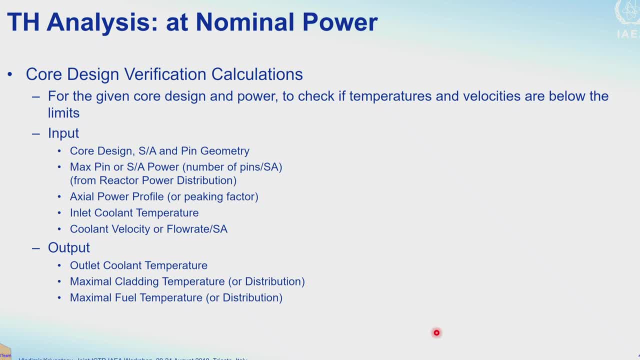 This is core design verification. So if you have a given core design and given core power, you should check if the temperature and velocities don't exceed the limiting parameters. And as an input we have, of course, core design, geometry and power. 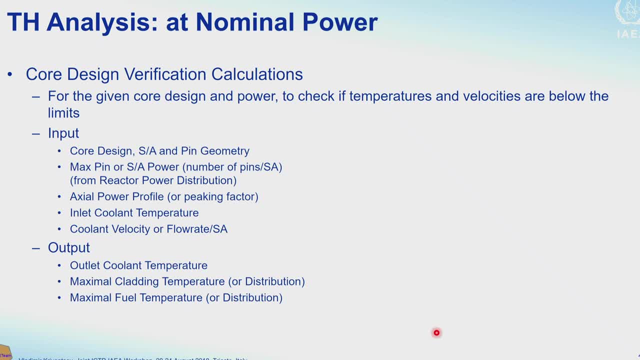 Then you have, let's say, okay, it's power, and then you should also be provided by axial power profile or picket factor, for example, to make simplified calculations: inlet coolant temperature and coolant velocity or flow rate per sub-assembly. 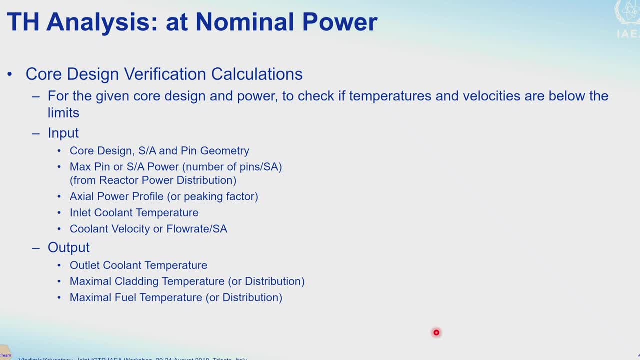 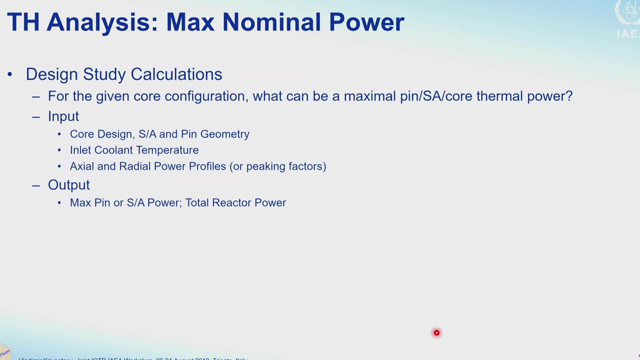 As an output you have outlet coolant temperature, maximum cladding temperature or distribution of temperature versus cladding because of gradients are also important, and maximum field temperature or its distribution. Another type of analysis. it's you should calculate maximum nominal power of the fuel assembly. 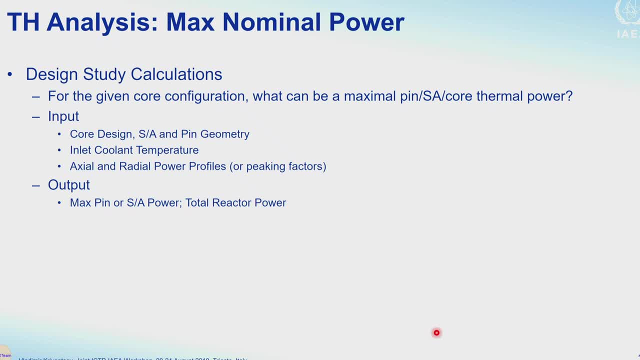 or the reactor for the given geometrical parameters. In this case, you have a configuration, core design, flow rates and everything, and take into account the limiting parameters like maximum field temperature, maximum cladding temperature, maximum coolant temperature.